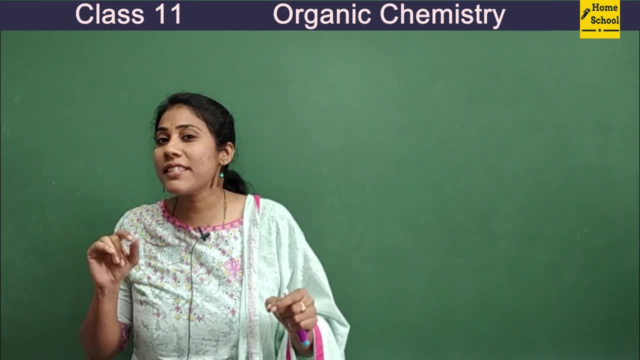 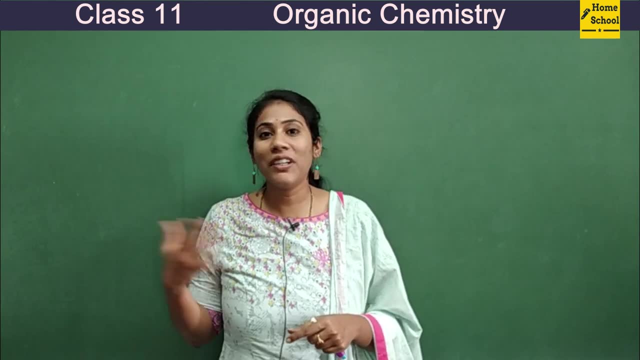 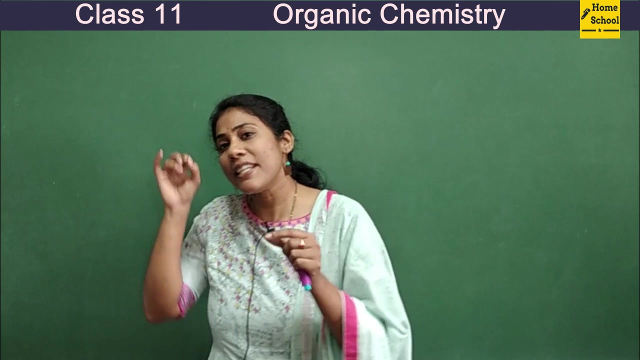 I can say this: organic chemistry is the scoring topic in chemistry for all types of competitive examinations. But many feel working with organic chemistry questions is a difficult task. Why? Because questions will not be asked from a single topic, from a single chapter. You will have combined. 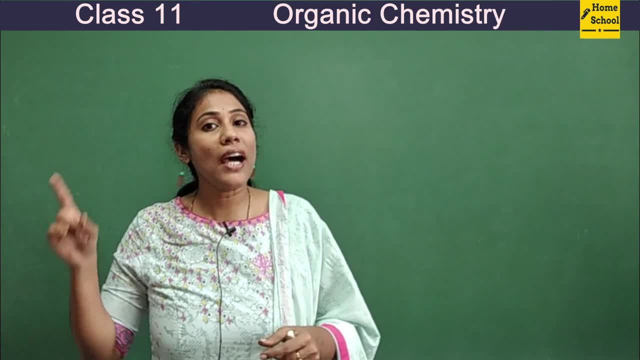 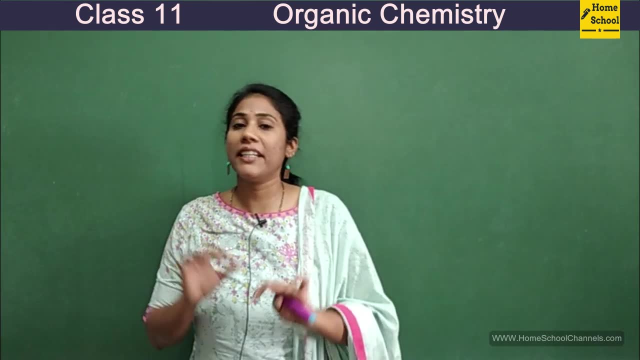 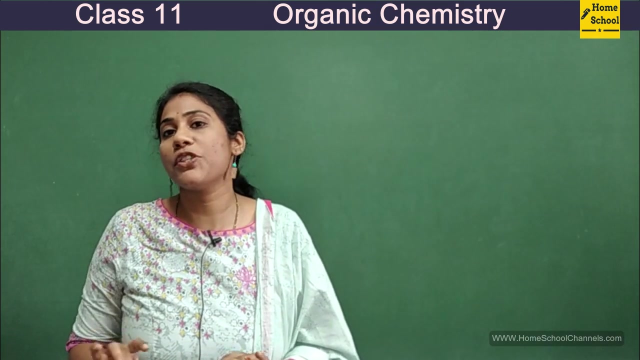 concept from all the chapters. See, if you have to attempt or solve a question of organic chemistry, you should have complete knowledge on all organic chemistry chapters. Two chapters you will study in class 11 and four core organic chapters you will study in class 12.. So all together six core organic chapters. 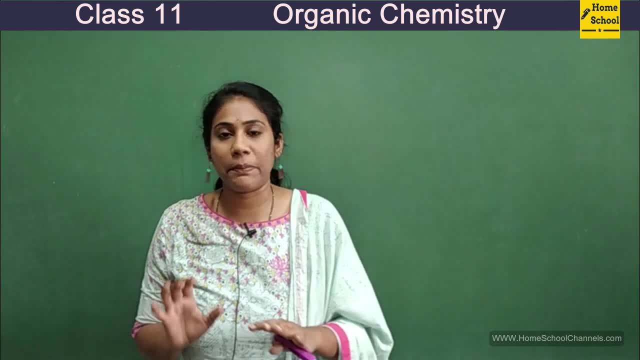 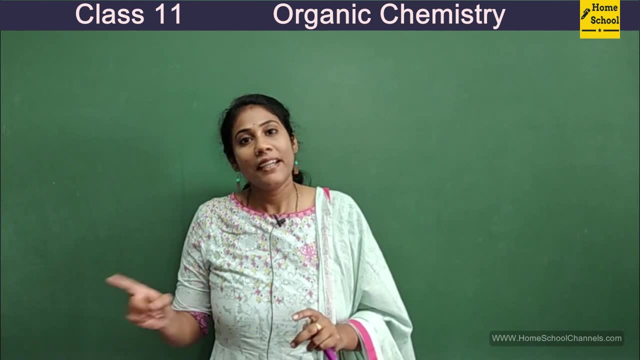 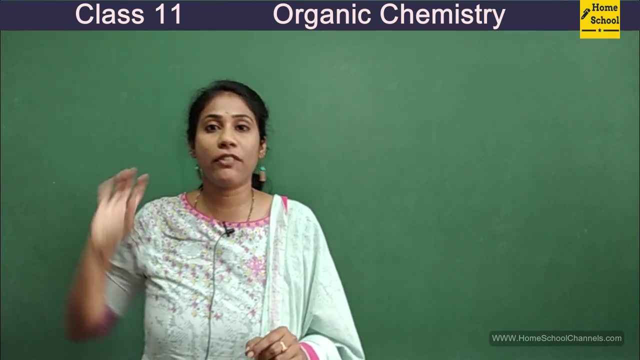 You should have a thorough knowledge on all the six chapters. Only then you can confidently attempt the questions relating to organic chemistry Right. So they will not be asking you from a single topic, From a single chapter question is a combined question- To attempt a question you should have. 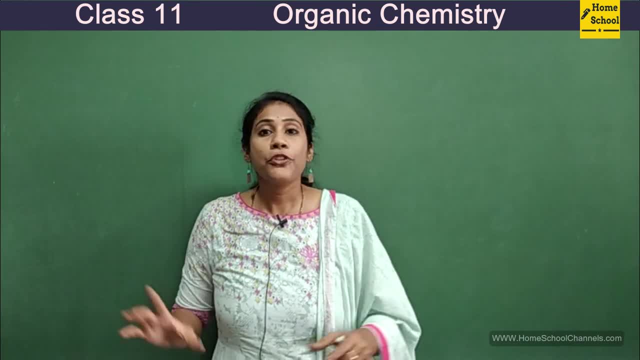 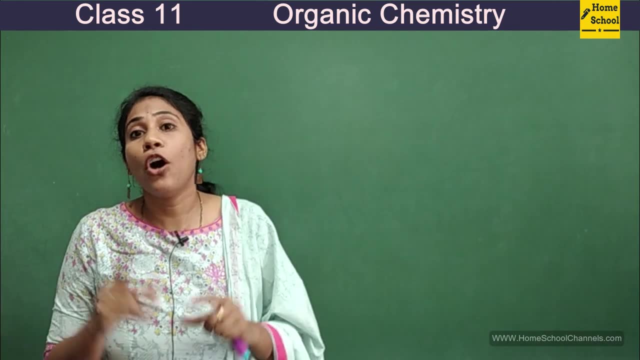 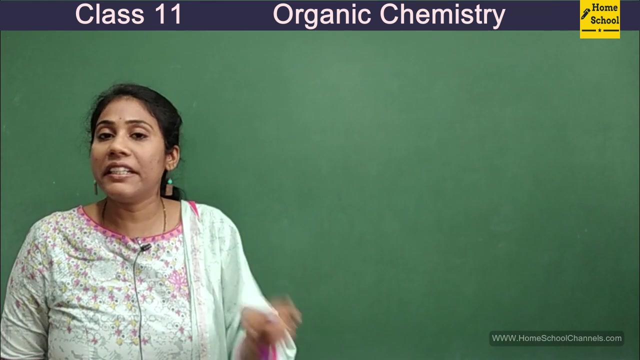 knowledge on all the six chapters. right So, and coming to this particular chapter, very, very fundamental and very, very basic chapters of organic chemistry, very much essential to understand each and every topic of this chapter in a detailed way. Only then you can confidently understand or confidently study. 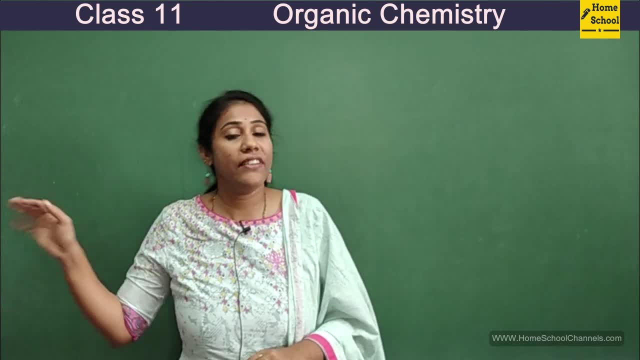 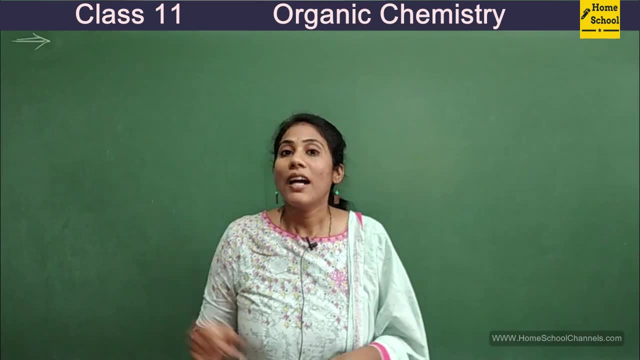 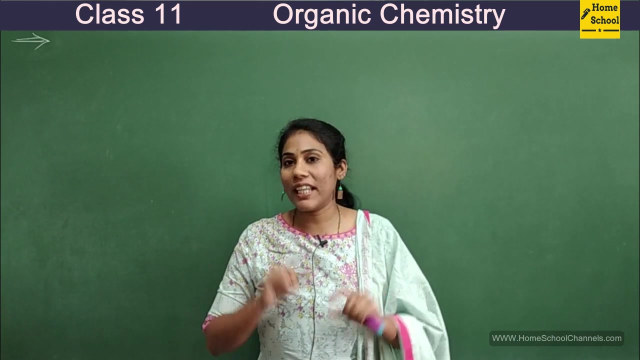 the rest of the organic chapters, both in class 11 and class 12. so i am here to make your study of organic chemistry much easier. i can assure you that after watching my videos, your confidence levels will increase in studying organic chemistry. so do watch the videos till the end and get. 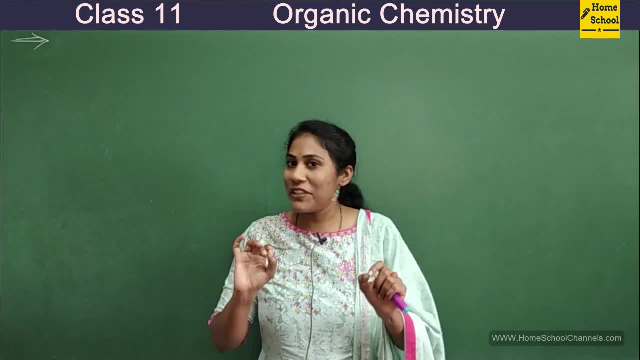 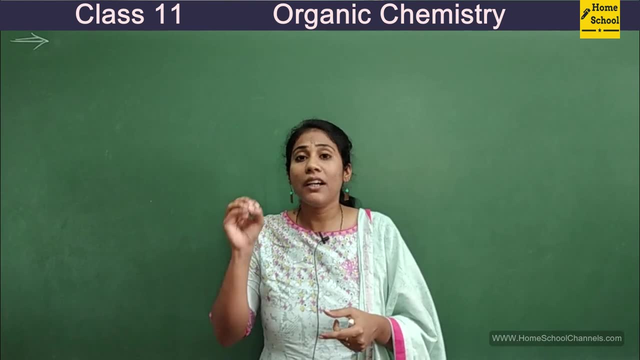 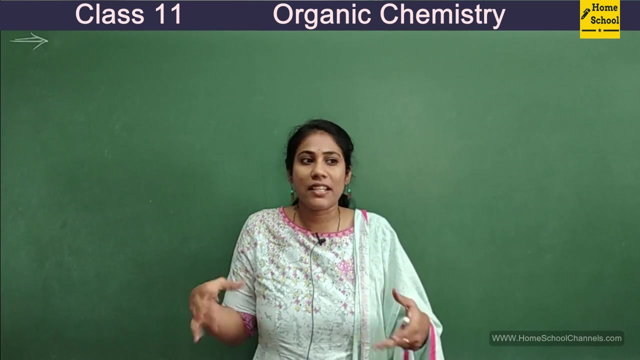 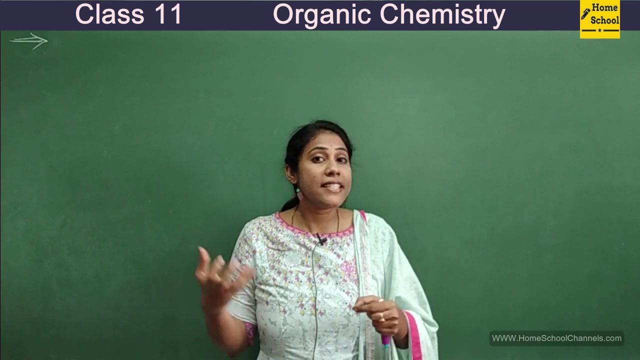 maximum benefit. okay, let's come to a chapter: organic chemistry. so today i will give introduction of organic chemistry, some history of organic chemistry and why this carbon is so special. organic chemistry is nothing but study of carbon compounds, so carbon is a very, very special element. we'll discuss why this element is special, why this separate branch for studying carbon. 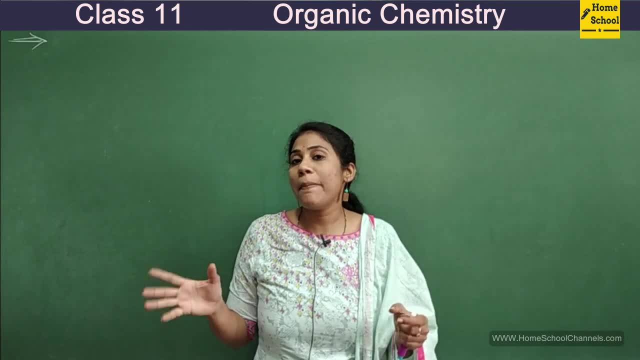 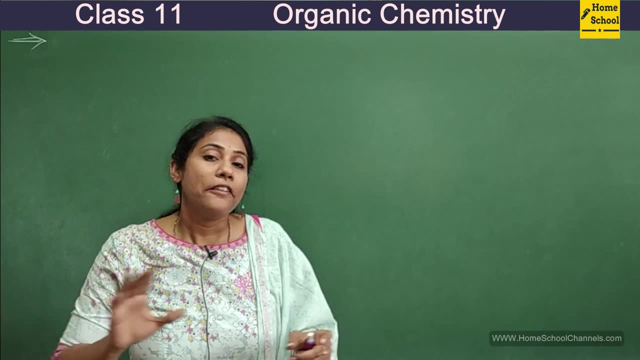 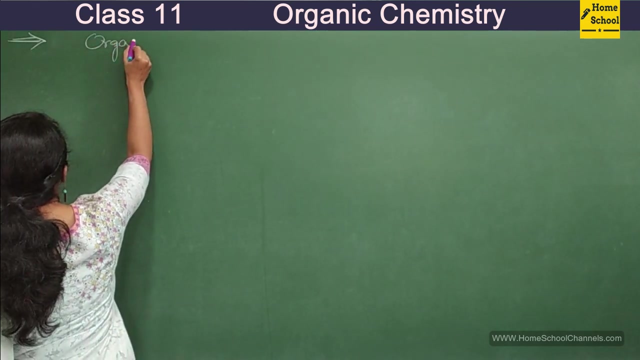 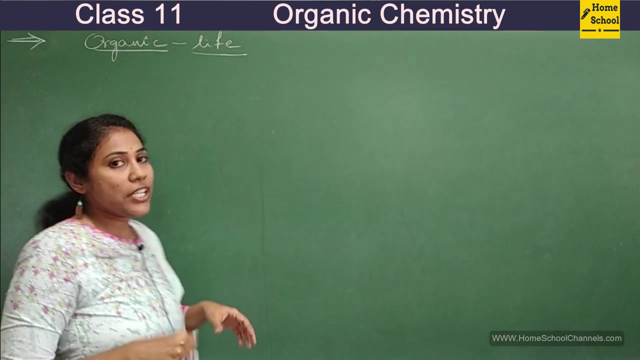 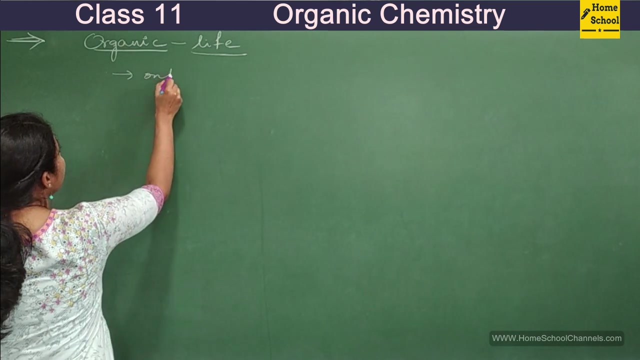 compounds. you know all that. and also, let's discuss about hybridization of carbon atoms. i mean shapes of organic compounds. okay, fine, coming to the word organic chemistry, try to understand the meaning of the word organic. organic means life, right? so initially, long back, people thought that organic compounds can be obtained only from plants and animals. okay, so they. 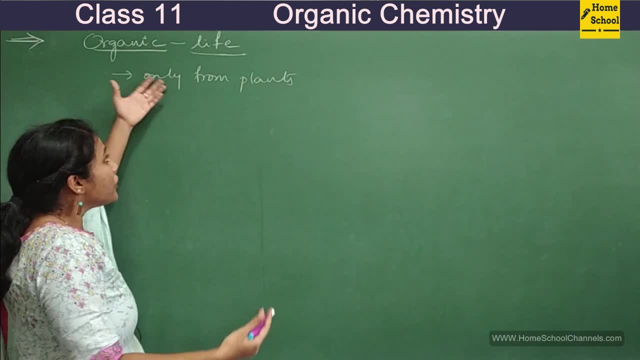 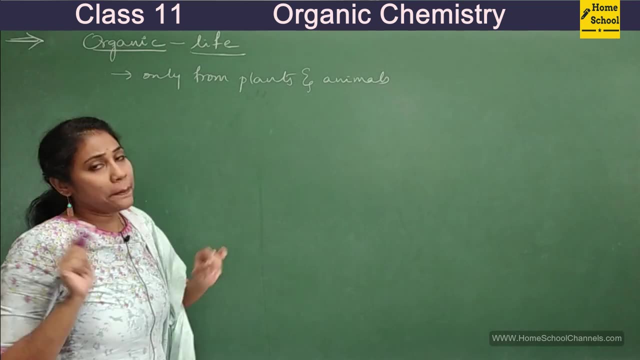 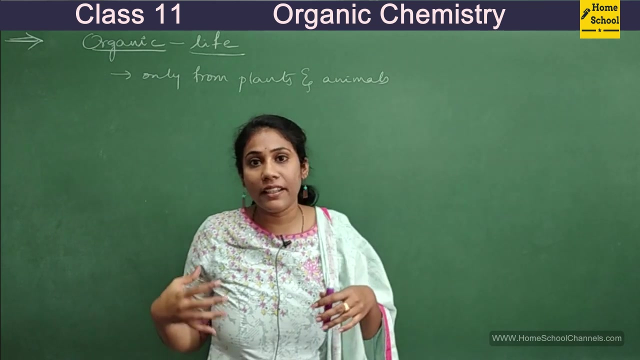 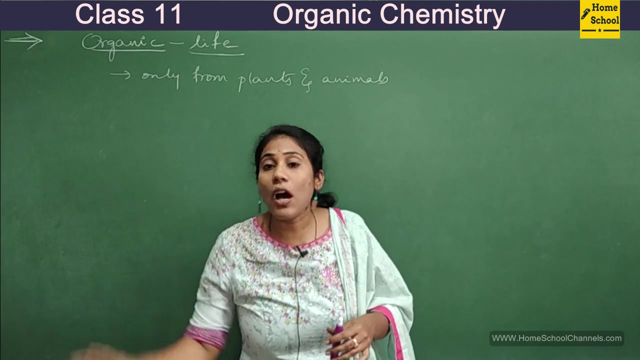 introduced plants as an way to have life right. they are in the knew production. they can grow fruits and vegetables at the same time. but that do not mean that organic compounds are the only good for this, but only an strangers binding liquid in. there are responses that these are certain chemical compounds which are naturally present in plants and animals. see, take human beings. our body is completely made up of chemicals, so we have lots of chemicals inside us, right and uh, you, you, you take a plant body and plant body also has lots of chemicals inside it. so these natural chemicals were bunch of different. you want to have many different chemicals? 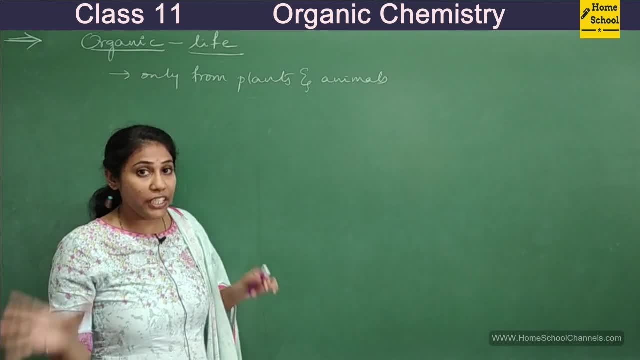 but obviously different sections. so there you should be. you must fresh mistakes, but you- God will work with it- rewrit you creative steps and you have to find solutions to get the right thoughts as well. and you should called as organic compounds initially. okay, and they thought that these organic compounds cannot. 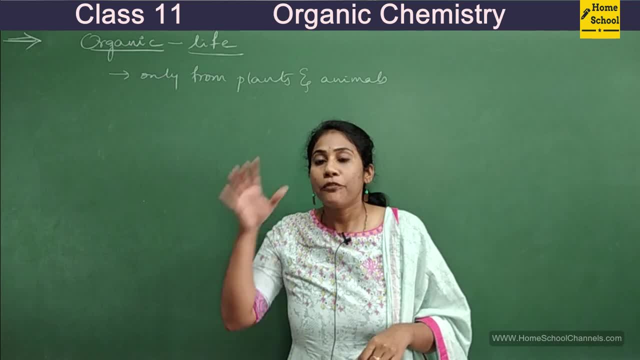 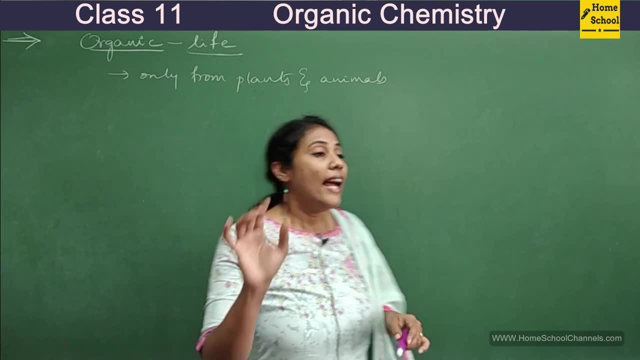 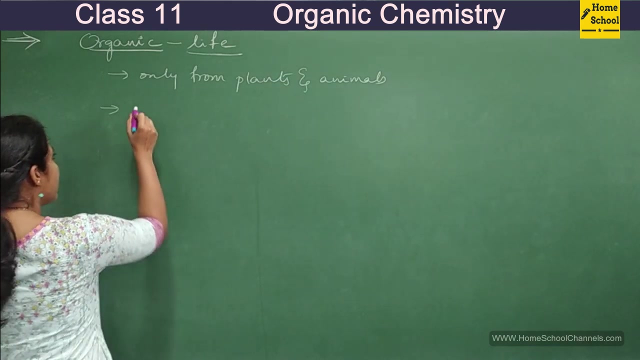 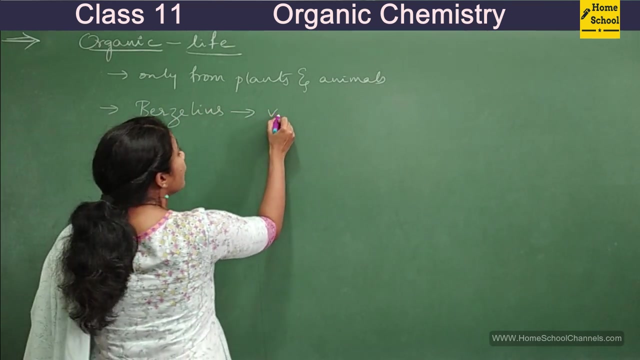 be artificially prepared in chemical labs. if you want organic compound, you should take it from plant or animal. they thought: okay, and there was a vital force theory which was introduced by berzelius. so berzelius was the scientist who introduced a theory called vital force theory. 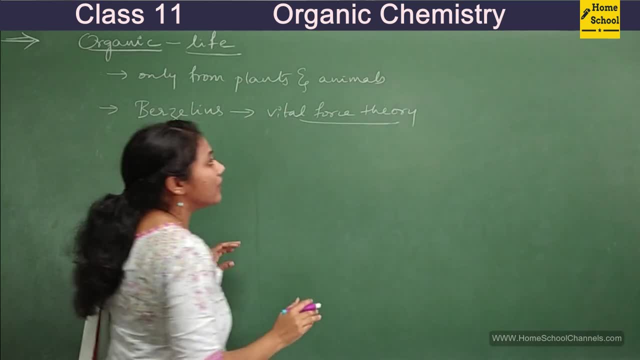 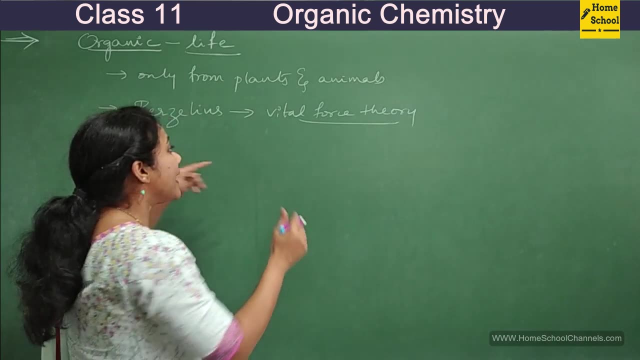 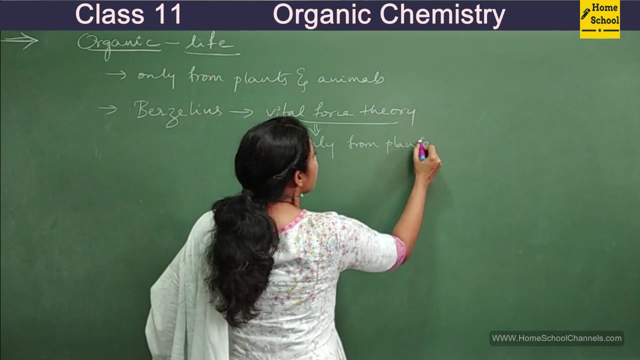 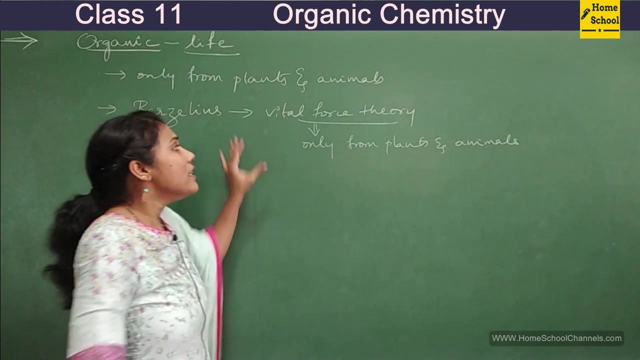 and according to this vital force theory- you know you can't prepare organic compounds artificially- if you want them, you should get. you should get only only from plants and animals. okay, so so to make this organic compounds which are present in plants and animals some vital force, some? 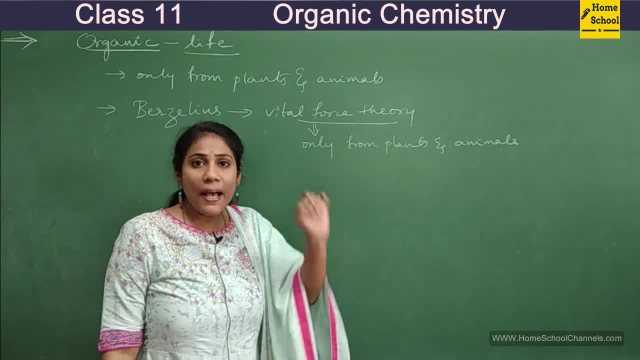 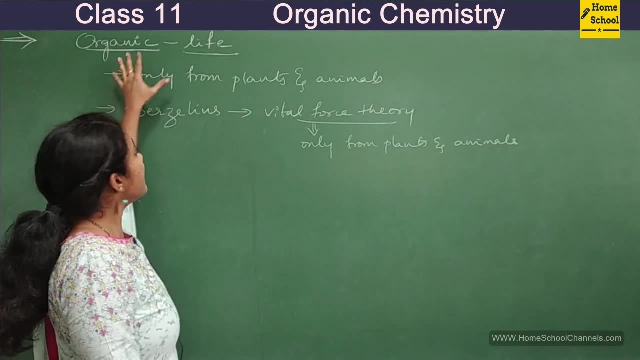 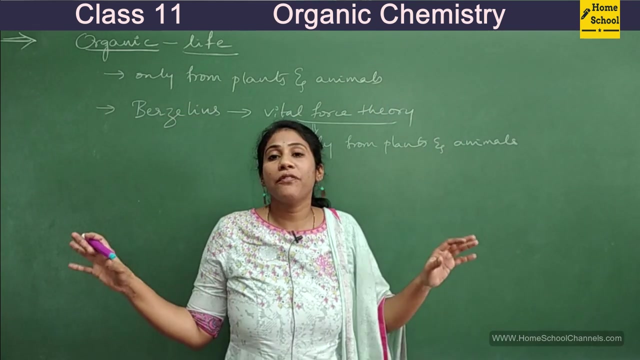 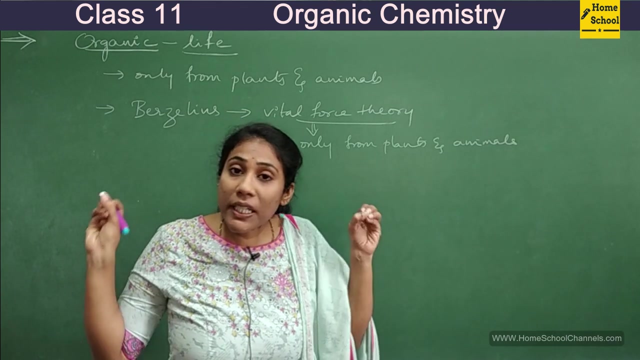 natural force is required. okay, so some natural force is responsible to prepare. you know, to make these organic compounds which are present in plants and animals, okay, so you can't prepare them artificially. you know, to make them, some vital force is necessary. some natural force is necessary so you can only get them from plants and animals. he said so. that is what. 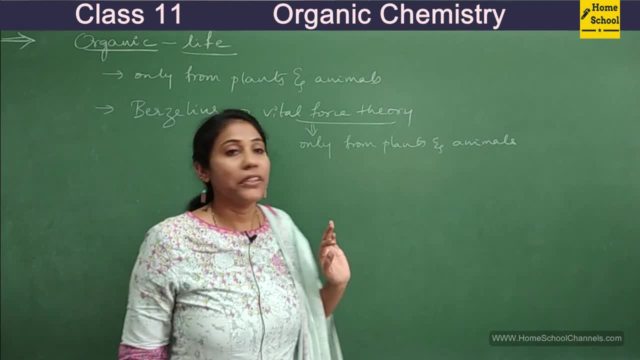 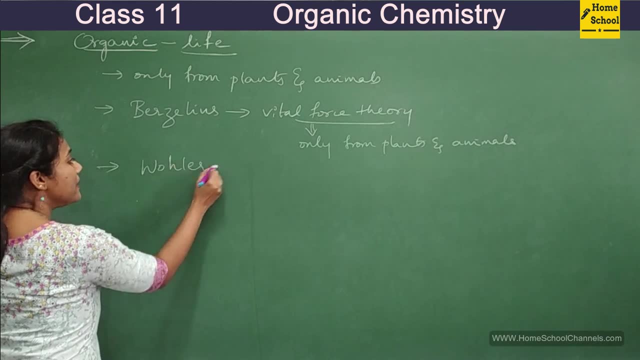 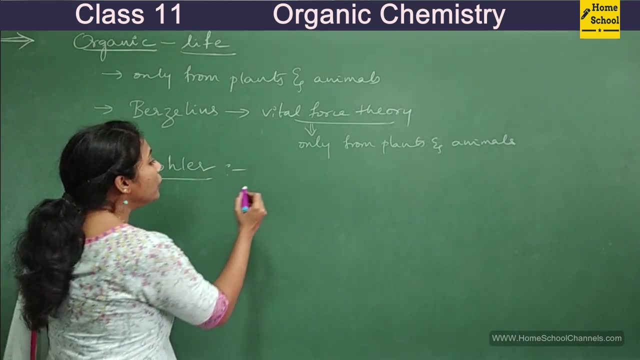 we call, as you know, vital force theory. okay, but there came another scientist called oler, okay, very famous scientist. so this oler has done some experiments in a chemical laboratory and he took ammonium cyanide, nh4 cno- this is the one which is called ammonium cyanide- and he took 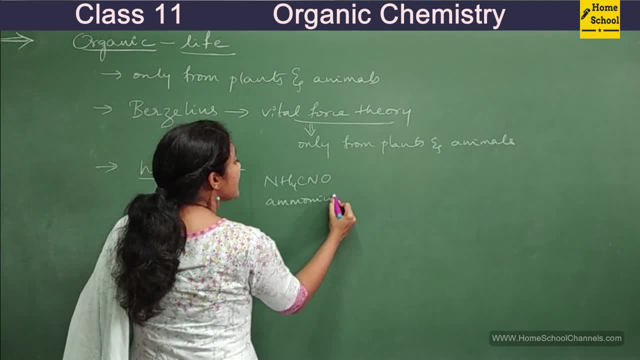 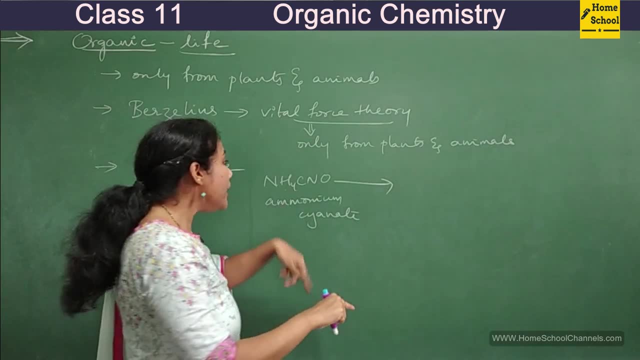 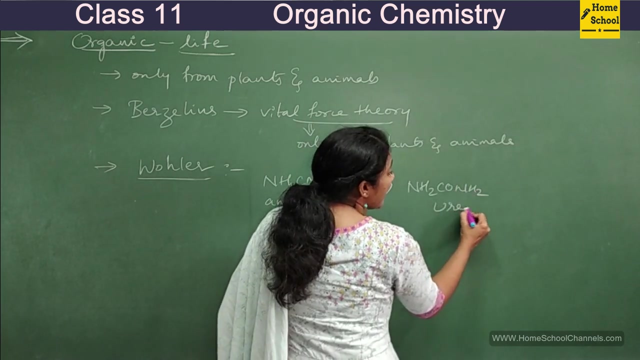 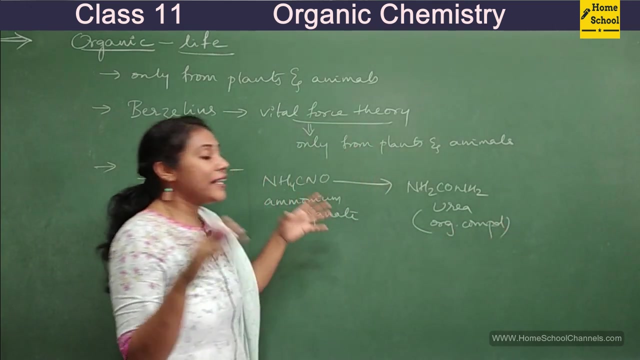 the formula of ammonium cyanide. okay, so from this ammonium cyanide in a chemical lab he could prepare, you know, nh2, co, nh2, which is nothing but urea, and urea is organic compound. okay, see, artificially in a chemical laboratory from inorganic substance and you. 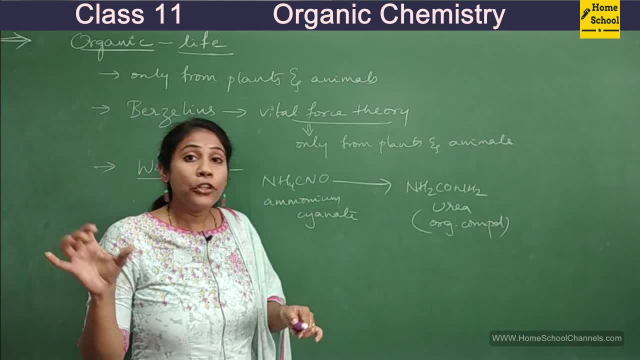 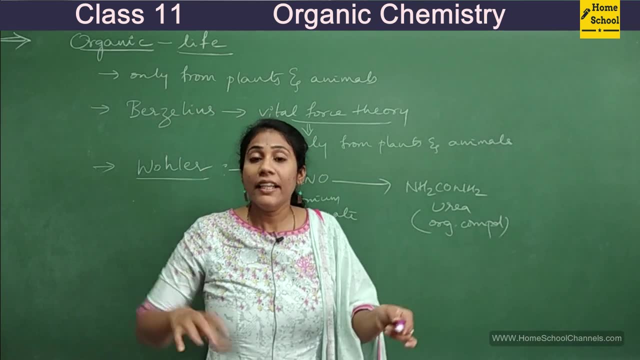 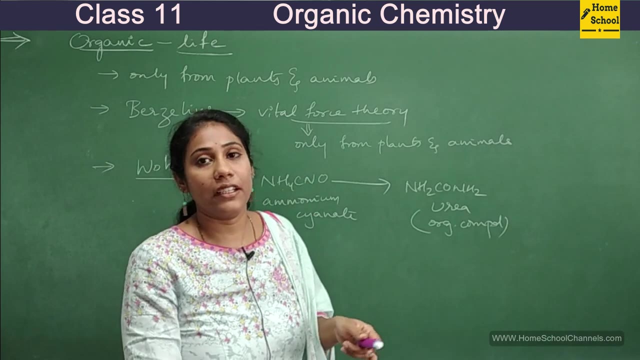 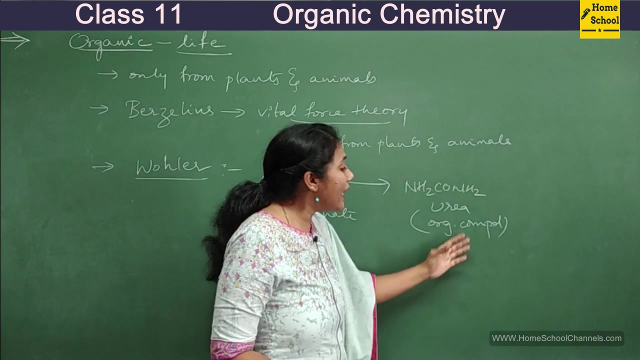 know, this substance is called as inorganic substance. you know, previously all chemical substances which are present in plants and animals were called as organic. every other chemical substances which are not present in plants and animals were called as inorganic. okay, so what did this oler do? he took some inorganic substance and from this he could prepare an organic compound. 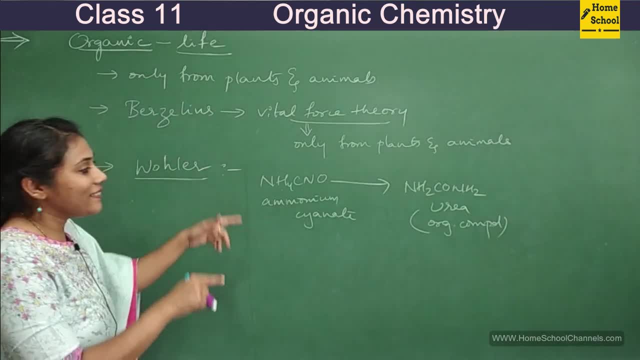 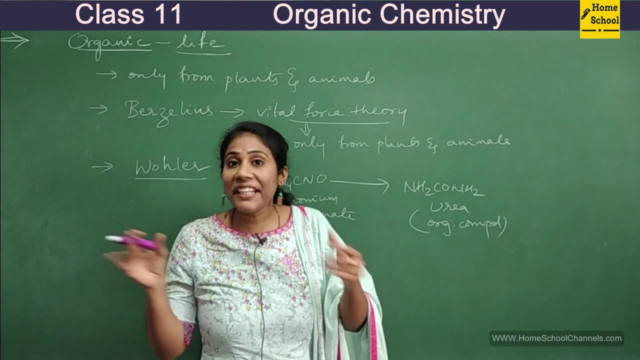 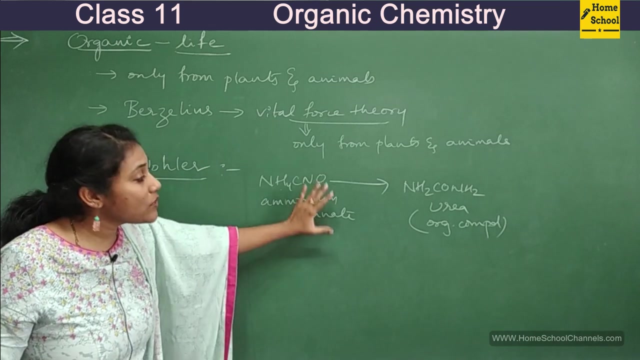 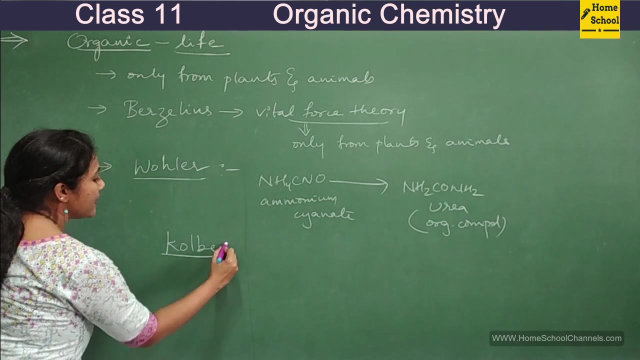 called urea. okay, so this came up as a revolution in the field of organic chemistry. from then, different scientists have tried preparing different organic compounds from inorganic sources. okay, so this was one of the example, and there came another scientist called cole. he's a very famous scientist and you have 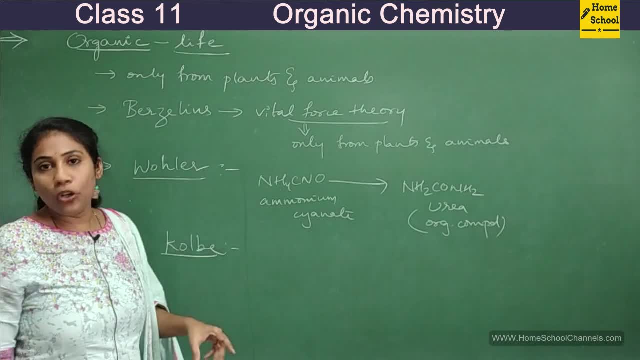 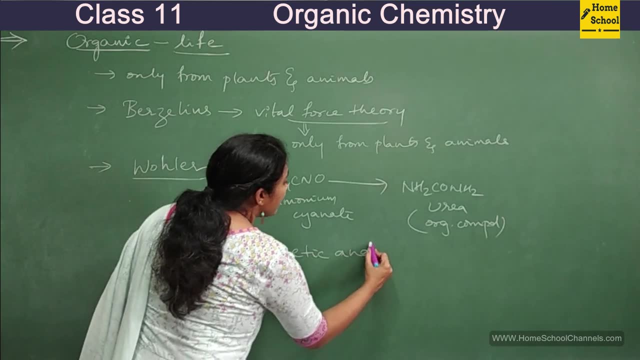 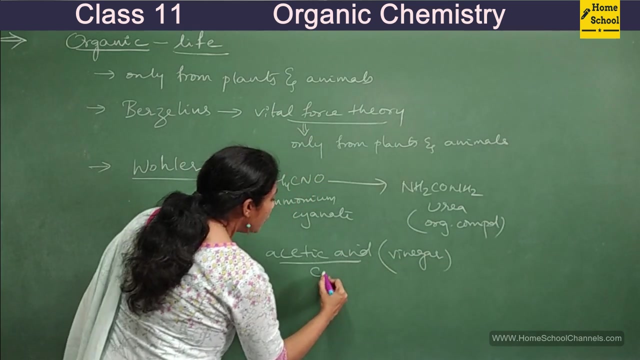 many reactions on his name. a person, cole, okay, and he prepared acetic acid. similarly, in a chemical laboratory, he prepared acetic acid. acetic acid is nothing but vinegar, okay, vinegar. so, uh, you know the formula right: ch3, co, h. little of organic chemistry. we studied in class 10 carbon and 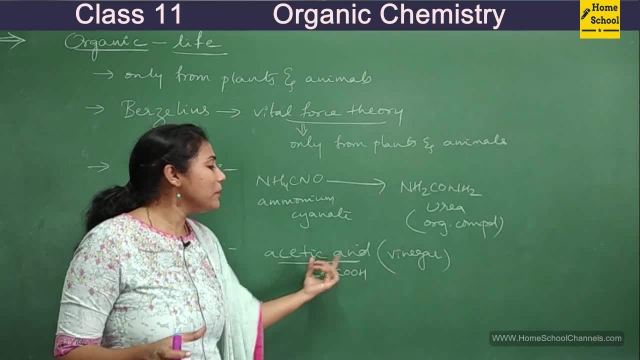 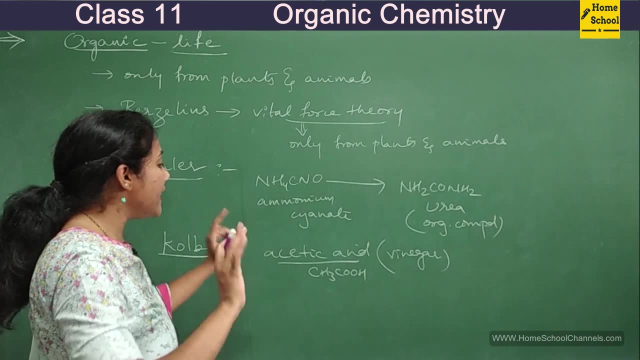 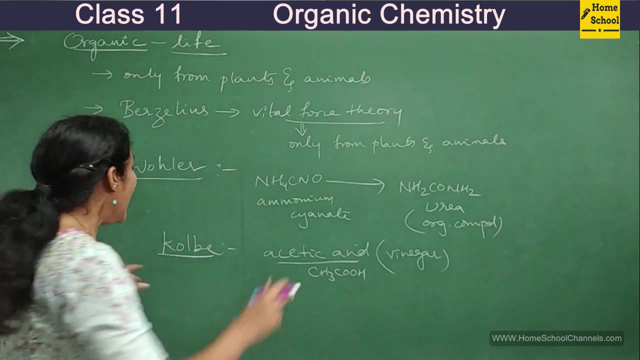 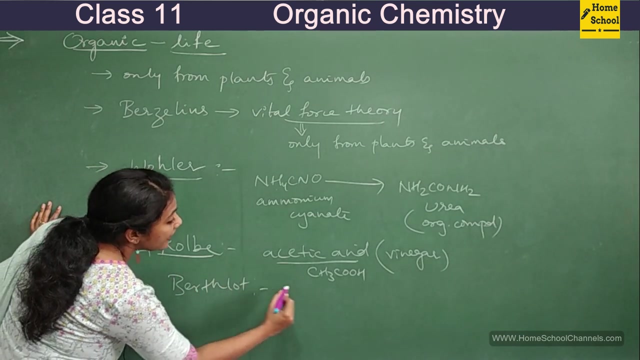 its compounds, right. so there we know the formula of acetic acid, that is, ch3, co h, which is nothing but a vinegar. okay, so this, uh, you know, this compound was artificially prepared by a person, cope. okay, and there came another person called berthlot, berthlot, okay, and he prepared. 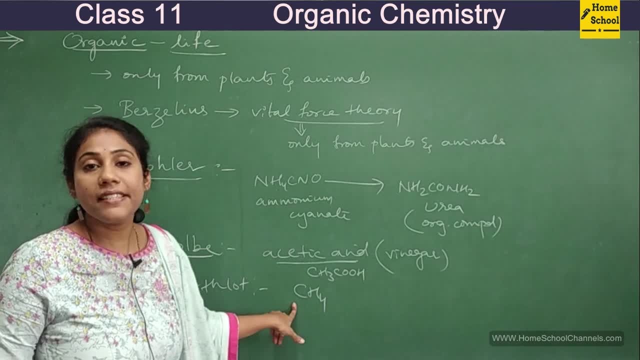 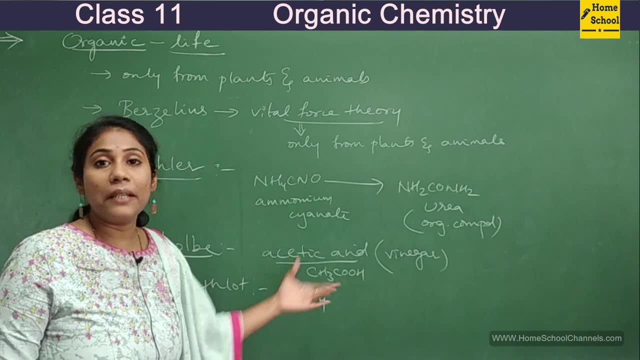 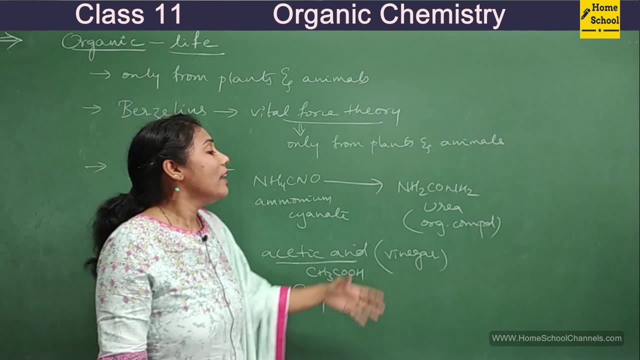 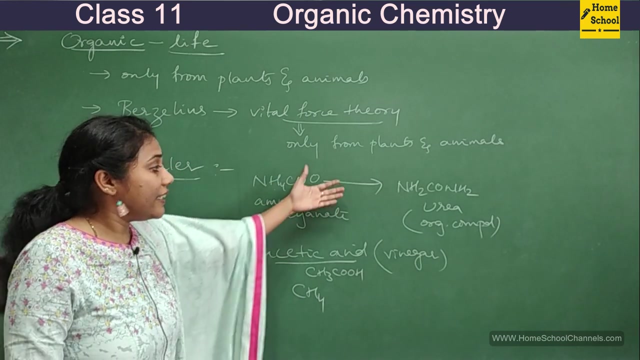 methane. so we all know what is methane right. ch4. so methane was also artificially prepared, you know, from the elements, that is, carbon and hydrogen, right. so, uh, like this, many scientists came up and they could prepare organic compounds at home artificially in the chemical laboratories you know from inorganic substances. they are not. 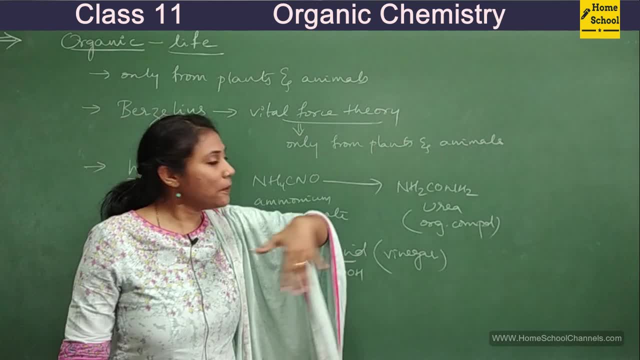 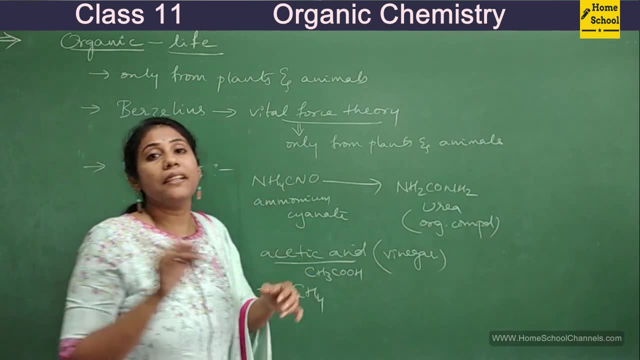 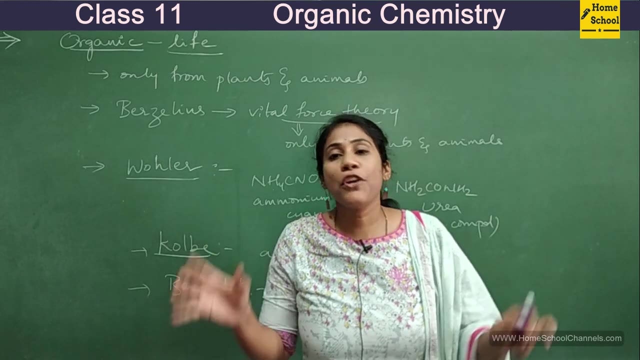 preparing from plants and animals. they have not extracted from plants and animals in turn. they have prepared from some inorganic substances by conducting some chemical reactions they could prepare artificially in the chemical laboratory. from then you know, hundreds of organic compounds were artificially made in a chemical laboratory and these organic compounds are. 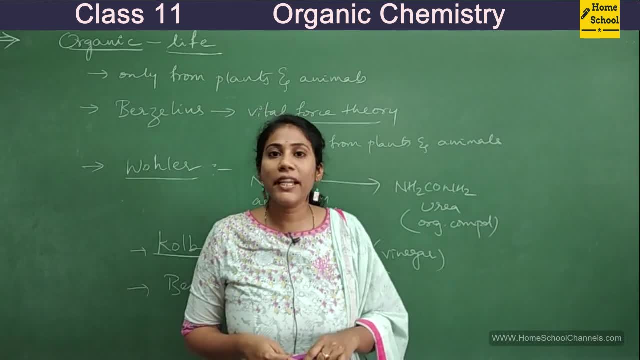 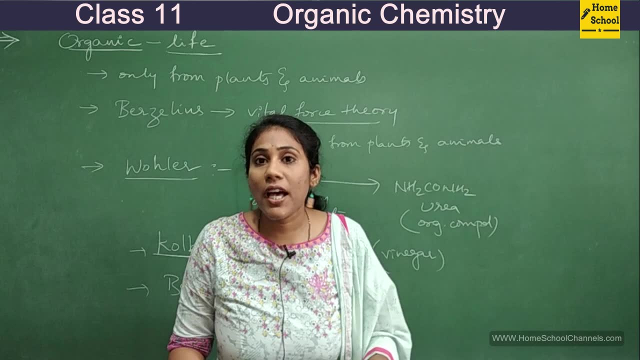 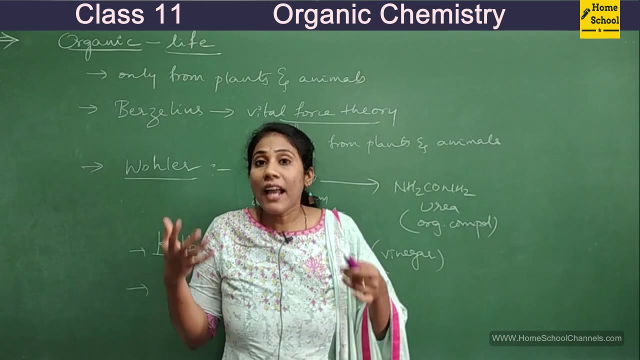 extensively used in all kinds of fields. okay, see, naturally speaking, all the chemicals which are present, all the substances which are present in plants and animals, is organic compound. right, so that we know, and apart from that you know, the drugs or the medicine that we take up during various 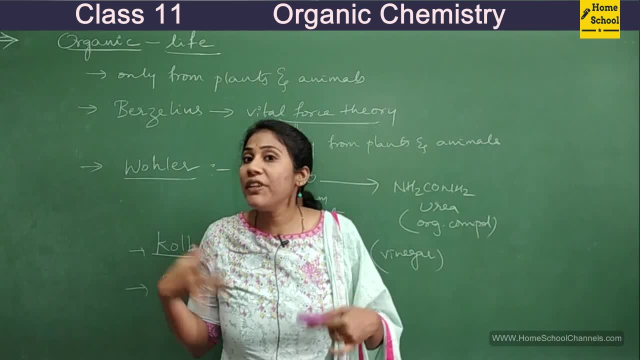 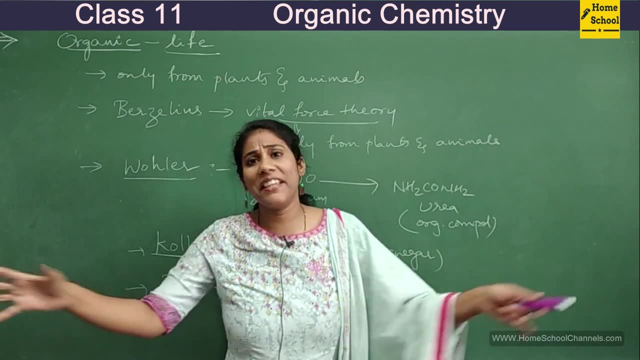 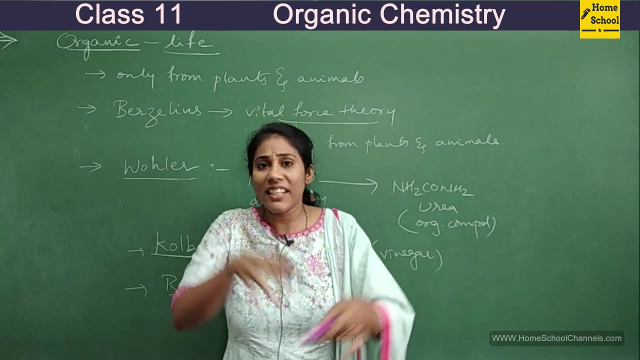 diseases belong to organic compound. you know the cloth we wear is organic right and the food we eat, etc. dust. these are 그러면 day products, as well as uh chemicals andмотря on these. all these plastic compounds are subjected to organic compounds, and bakery products and various 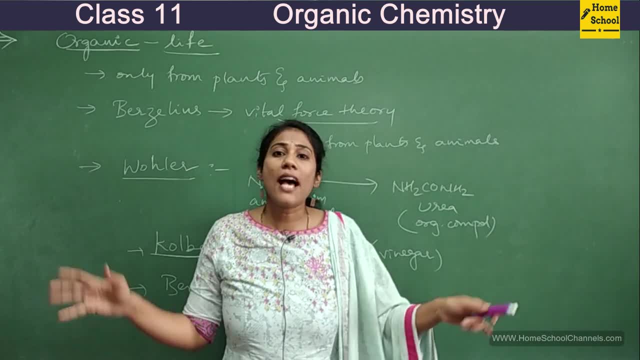 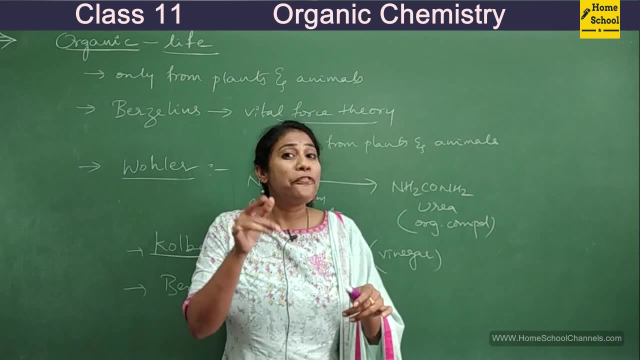 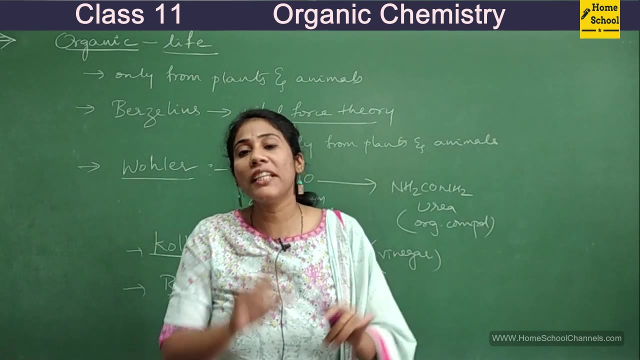 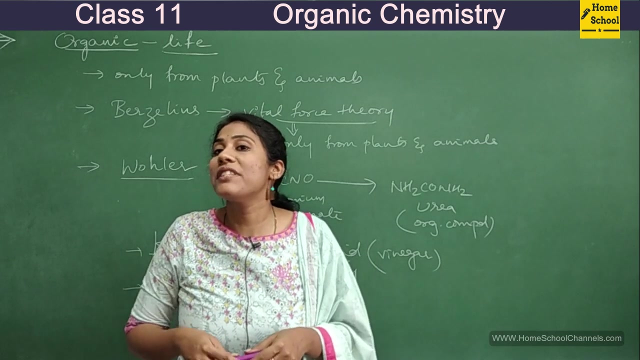 things, various things that we use. you know: the fertilizers, insecticides, so dye, industry colors, various colors, various pigments, various flavors. you know all these are organic compounds, right so you know what already about пом it. and every year 30 000 new organic compounds are being discovered, right so this way, you know. 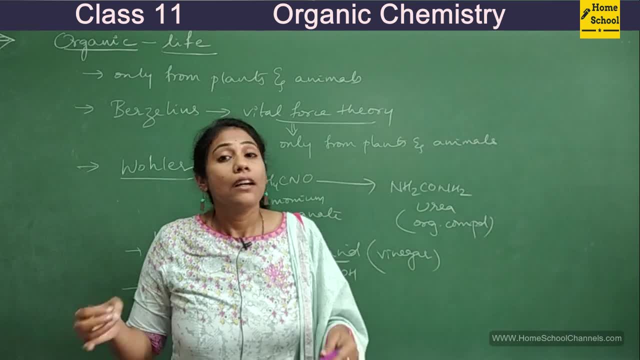 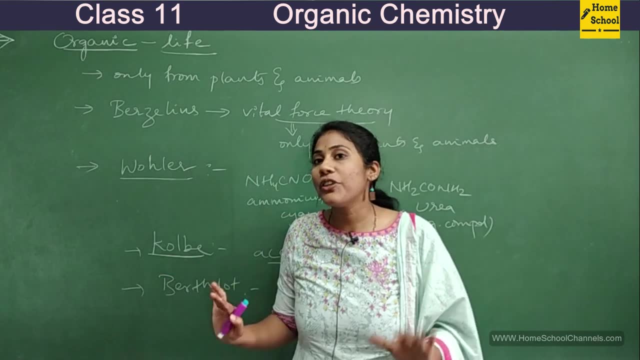 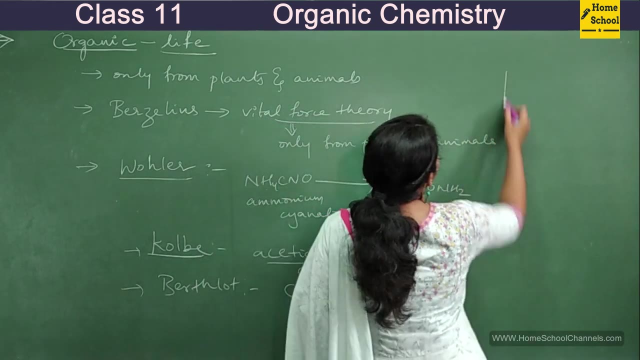 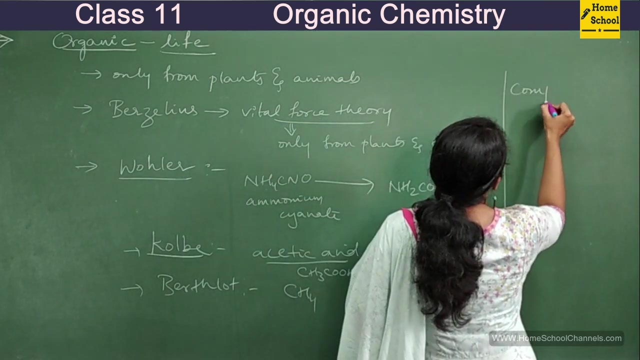 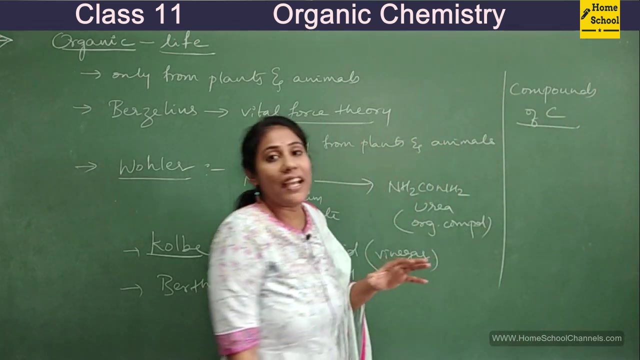 by conducting various reactions, people are making hundreds of organic compounds which have so many uses. right? so now we understood how this organic compounds are prepared and their history. right now, let us try to understand what actually we mean by organic compound. okay, so organic compound is nothing but compounds of compounds of carbon. okay, so, in in a simple language, if i have to, 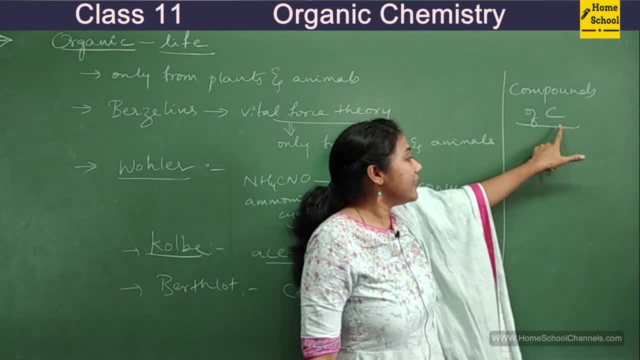 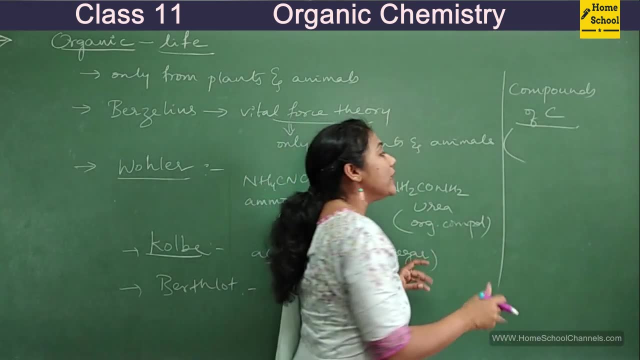 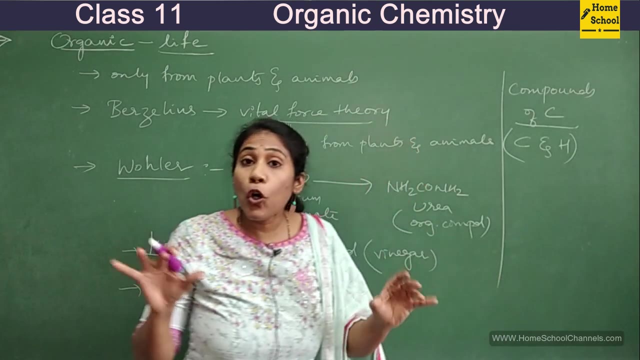 talk about organic compound, i can say they are nothing but compounds of carbon. okay, say the: if you have to call something as organic compound, then that compound must come with hydrogen, right? so if you have to call something as organic compound, then you have to compulsorily have carbon and hydrogen, okay, so only then you can call it as organic compound. 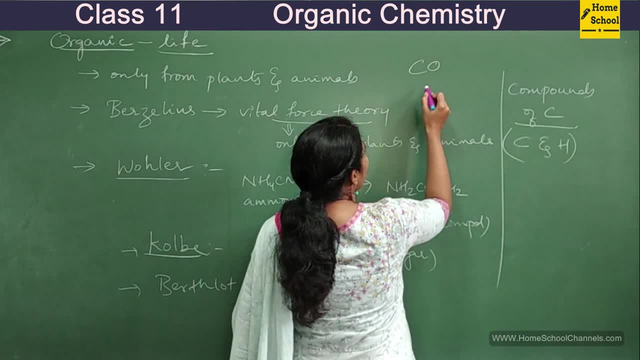 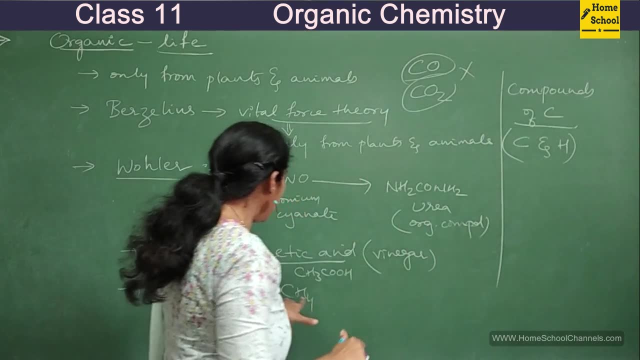 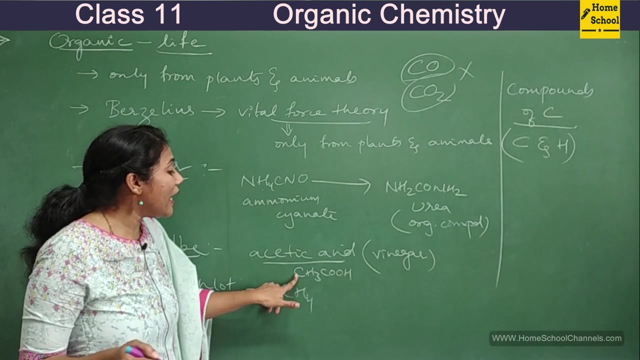 is that clear? say: we have carbon monoxide, we have carbon dioxide, we will not call them as organic compound. right, but we call ch4 as organic compound, ch3, co, oh. as organic compound. why? because carbon is there with hydrogen. so what is the compulsory? carbon and hydrogen, right. so what is the 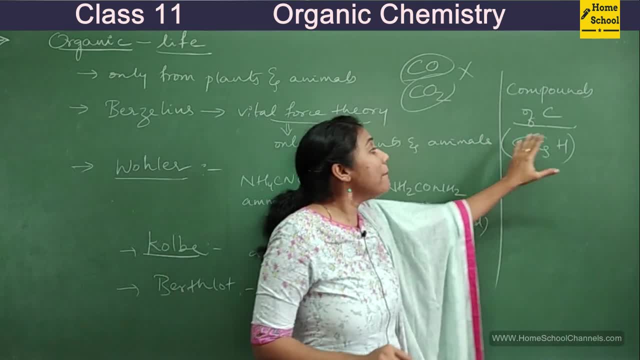 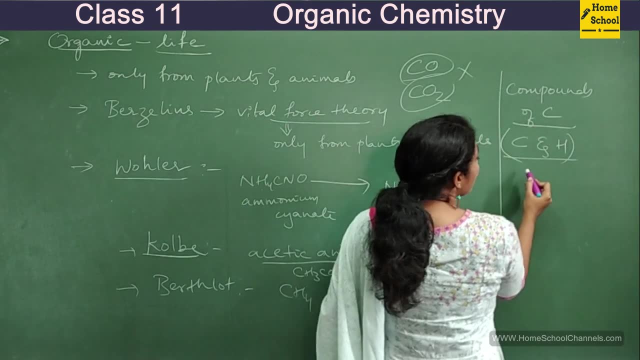 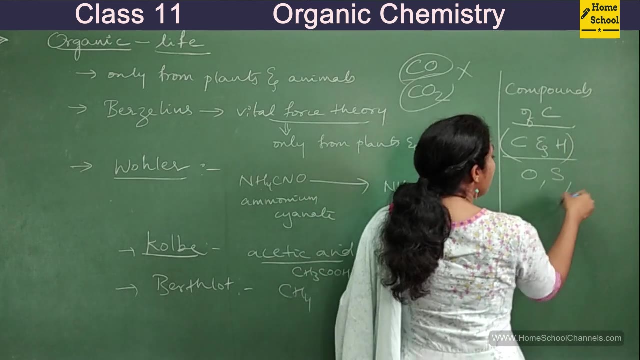 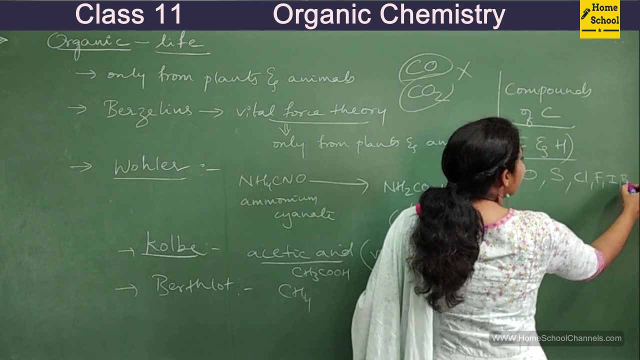 criteria to call something as organic compound. the compound or a substance must have carbon and hydrogen. along with carbon and hydrogen you will also find oxygen. sometimes, many times, oxygen you will find, or sometimes sulfur can be present, sometimes halogens like cl, f, i, b? r these guys. 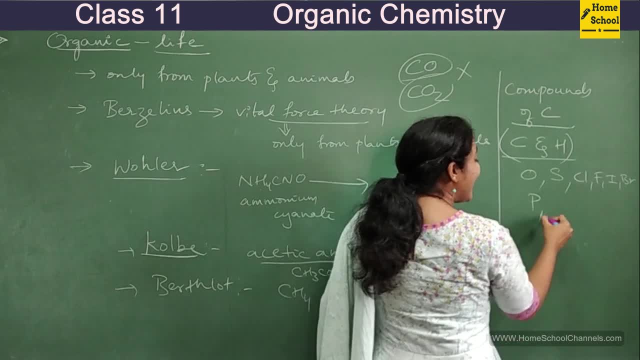 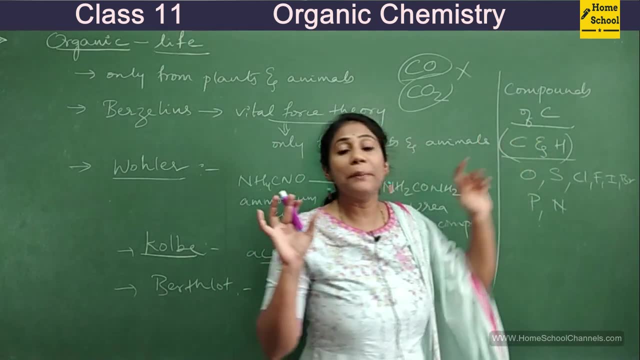 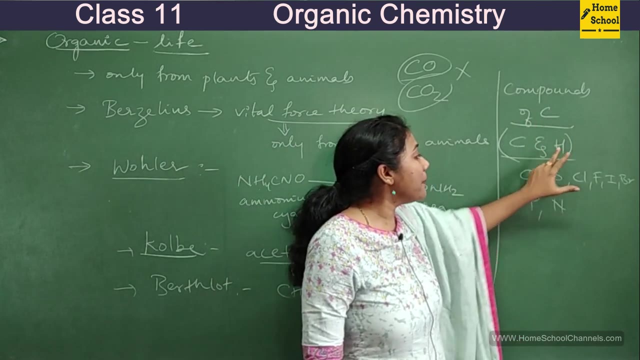 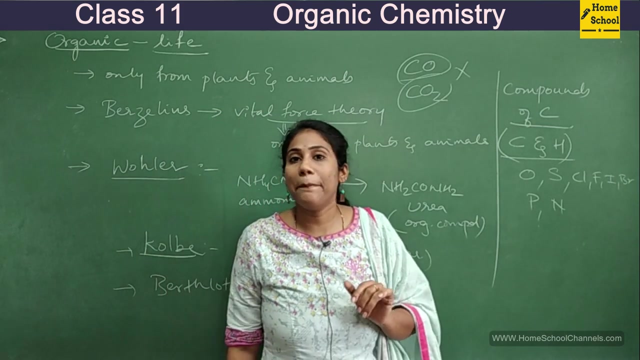 can be present, or phosphorus can be present, okay, nitrogen can be present: okay, and hydrogen can be present: right. but the necessary condition is: compound must have carbon and hydrogen, not just the carbon. carbon must be there with hydrogen, along with these two elements. these elements also can be present. only then you will call it as organic compound. okay. so organic chemistry is all. 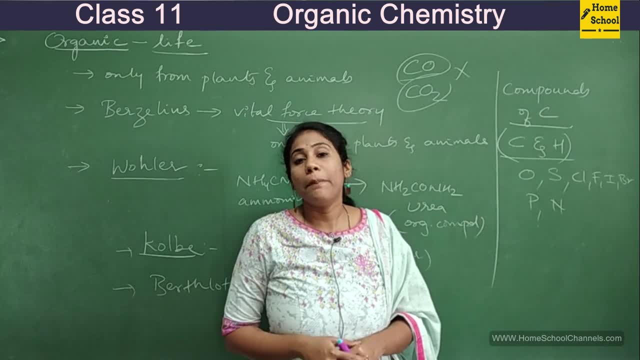 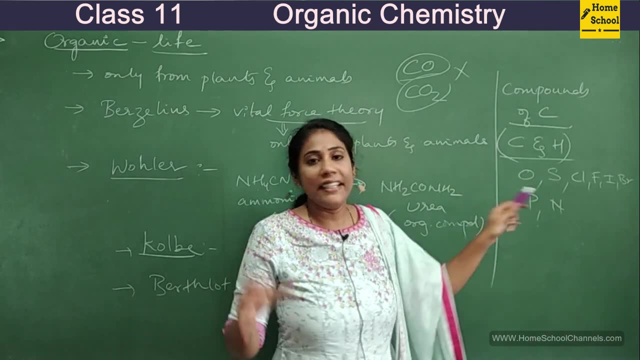 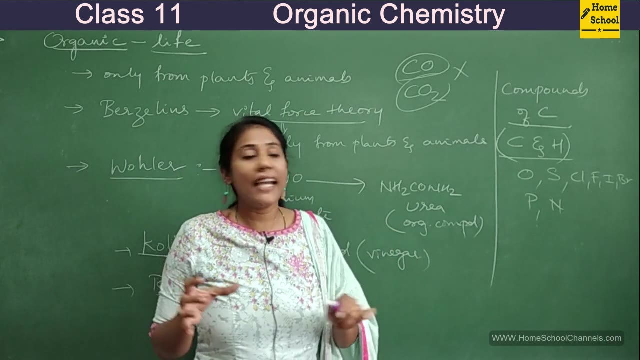 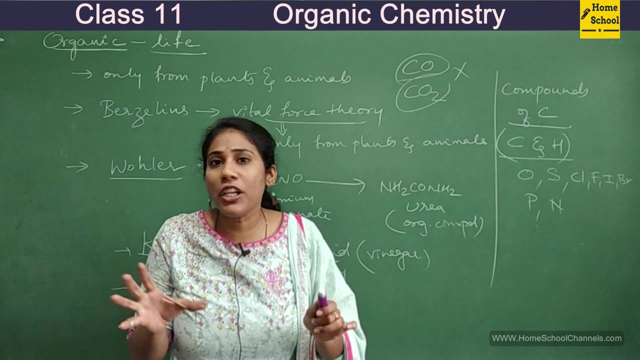 about studying the nature of organic compound, properties of organic compound, reaction of organic compound and everything about organic compound. okay, fine, see carbon. the main element present in organic compound is carbon, so without carbon you cannot call it as organic itself, right? so what is so special about that carbon? right? so why? this carbon can make crores. 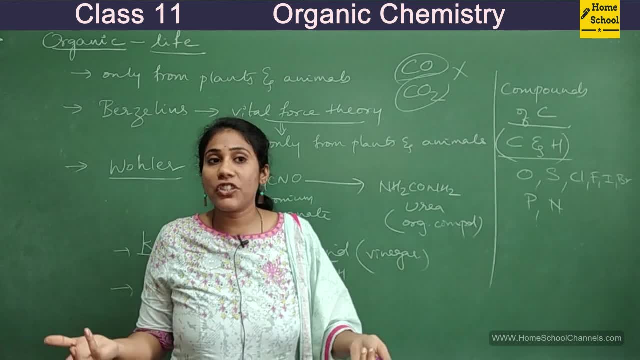 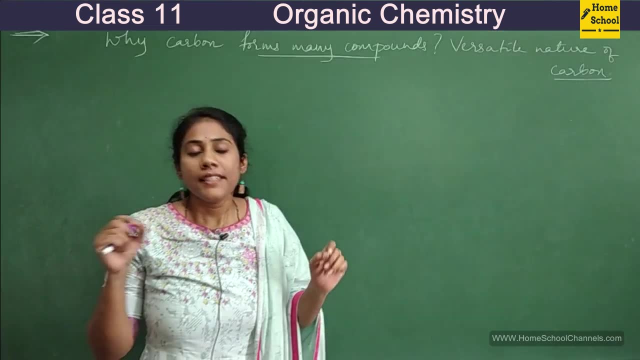 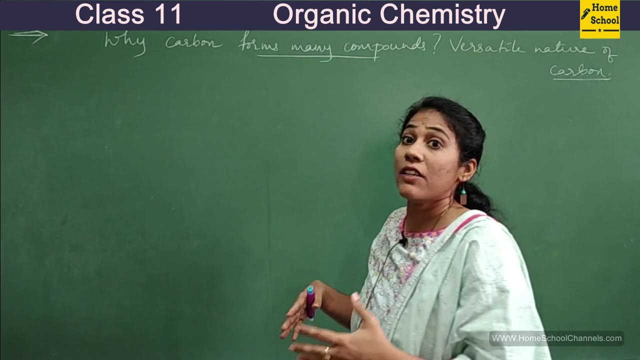 and crores of compounds. you know that can exist in our nature. so what is so special about this guy called carbon? that's what we will try to discuss now. see, guys, there are mainly three reasons why carbon is very, very special, right? so normally we say: uh, the versatile nature of carbon. 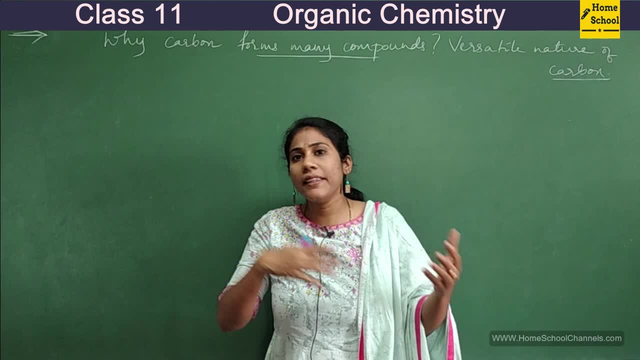 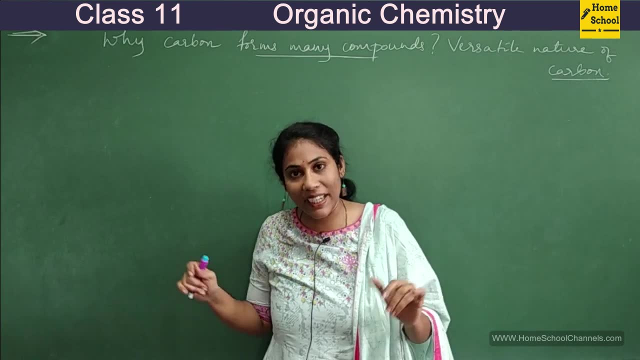 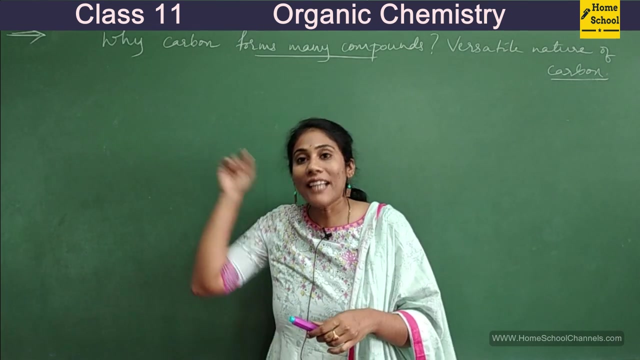 versatile in the sense what you know we say. the person is very much versatile. that means if he is multi-talented person, we call him as versatile, right? so, like that, our carbon is also multi-talented element. okay, it will show many, many different properties. that is the reason it is so special. 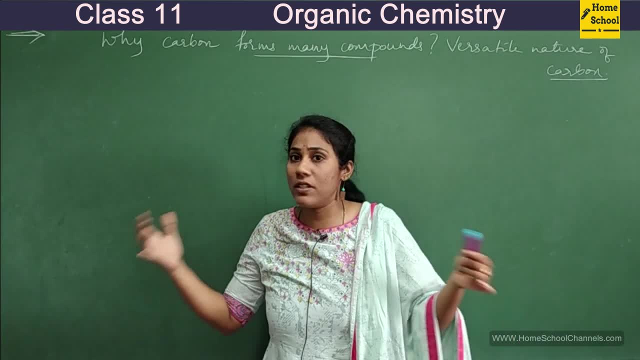 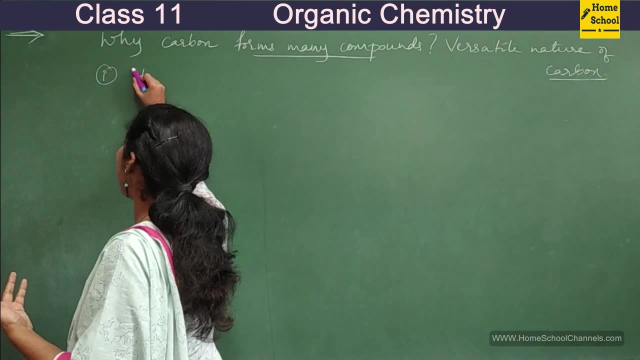 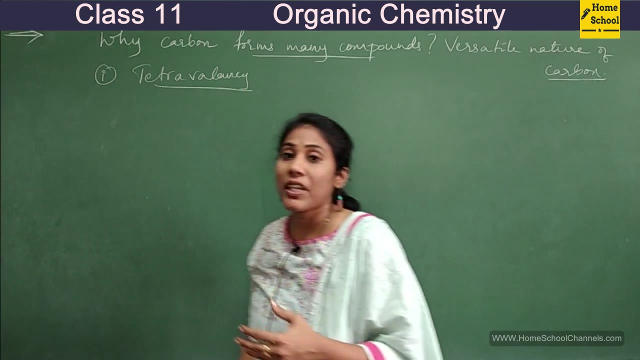 and it is forming many molecules or compounds in our nature. okay, so the first special character of carbon is having tetra valency, so tetra valency, nature. so what do you mean by tetra valency? tetra valency, in the sense valency of carbon, is four right. 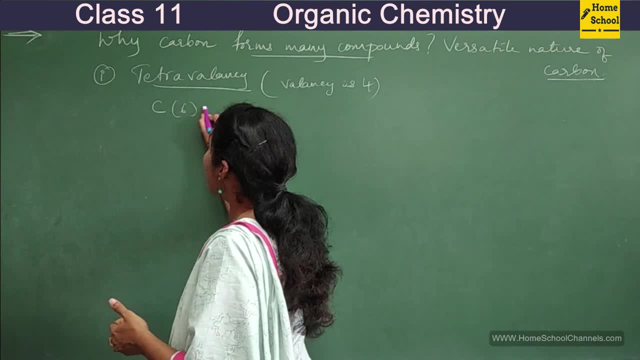 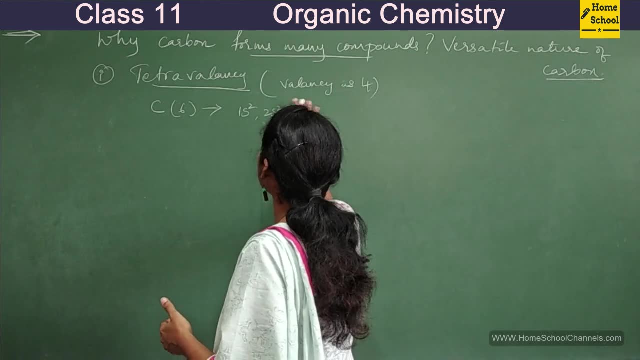 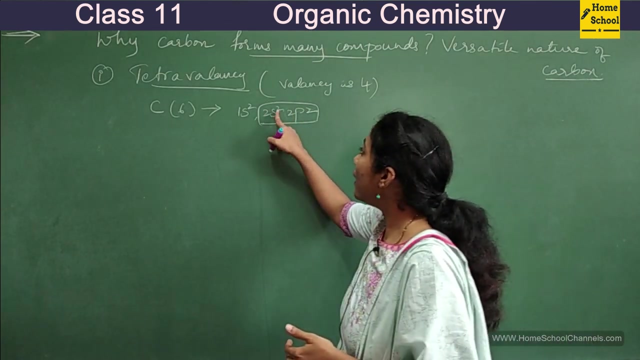 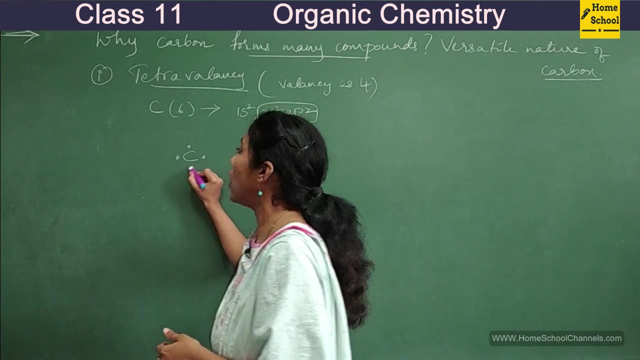 say carbon atomic number six, if i have to write its electronic configuration, one, s2, 2s2, 2p2, right? so in the outermost shell. outermost shell is our second shell and you have four valence electrons. okay, so our carbon has four valence electrons, right? so since four valence electrons are there, 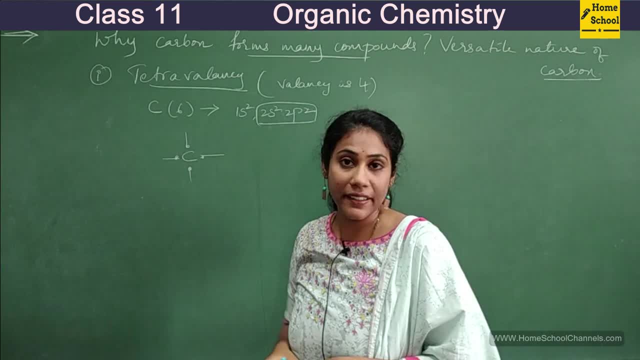 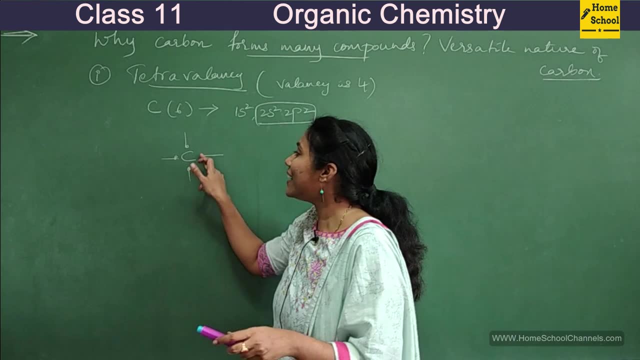 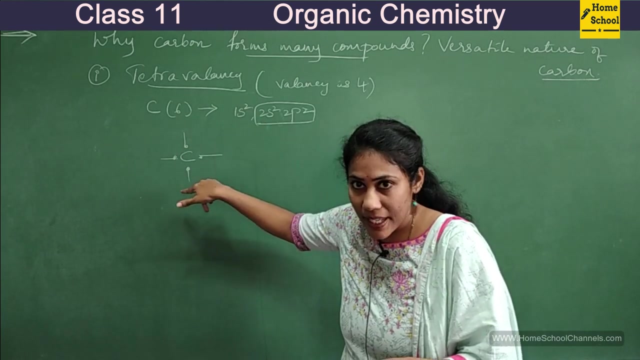 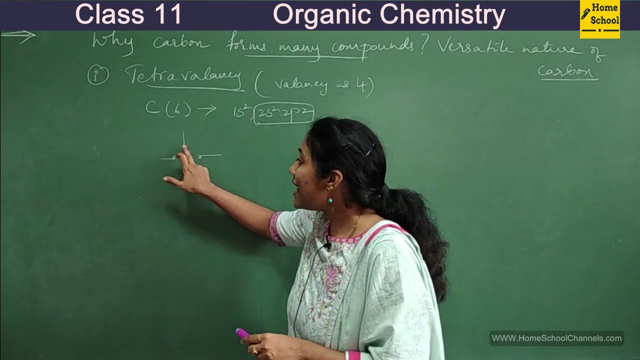 it can form four bonds around it. how many bonds it can form maximum around it? only four bonds. okay, so here the four electrons can be shared with other atoms. the other atom can be carbon itself or the other atom can belong to any other element. okay, so it has a ability to share. to share, it has a 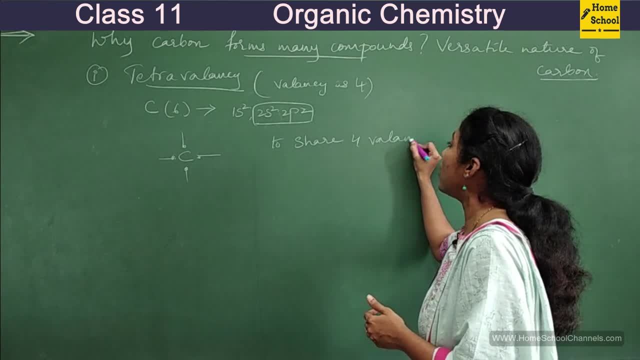 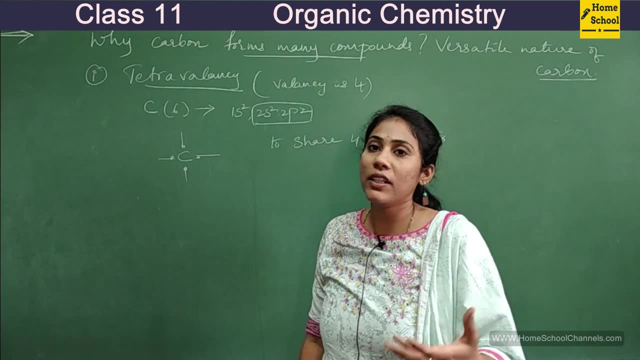 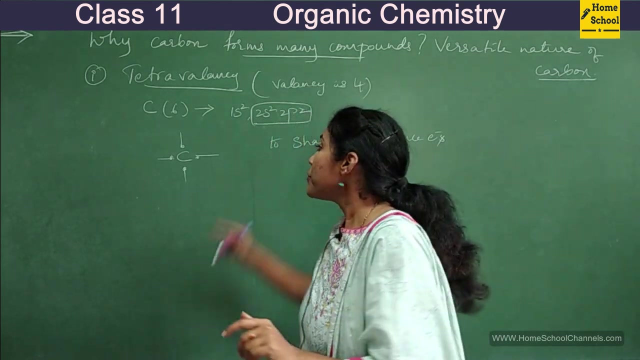 ability to share four valence electrons. okay, so that way it can satisfy octet rule. right, all these octet rule? uh? why? uh, the atom sharing electron, all that we have discussed in chemical bonding chapter, isn't it? so, since four valence electrons are there, it can share four electrons with. 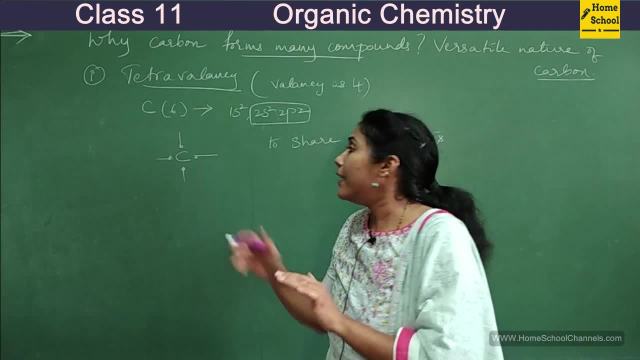 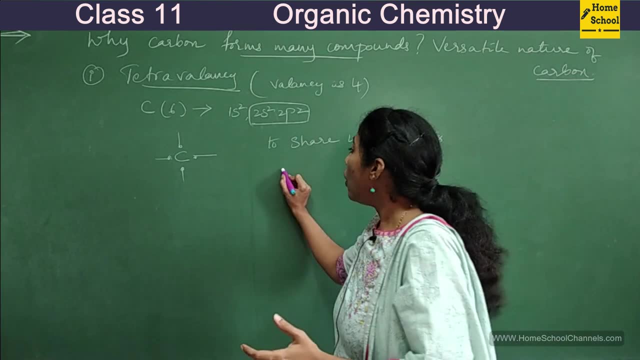 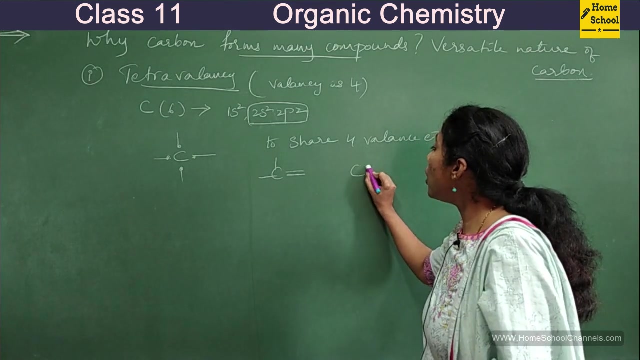 carbon itself or with some other atoms, and form four bonds. okay so, uh, it can form a�ium, build black, all four single bonds around it, or it can form, you know, two single bond and one double bond around it, or it can form one triple bond and one single bond around it. okay, so, altogether. 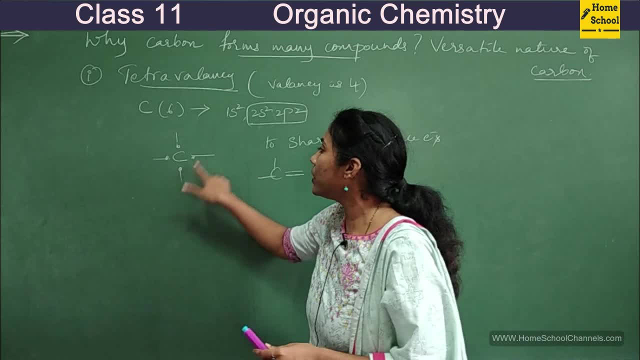 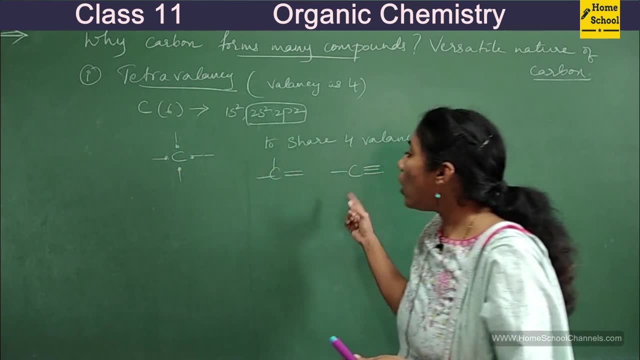 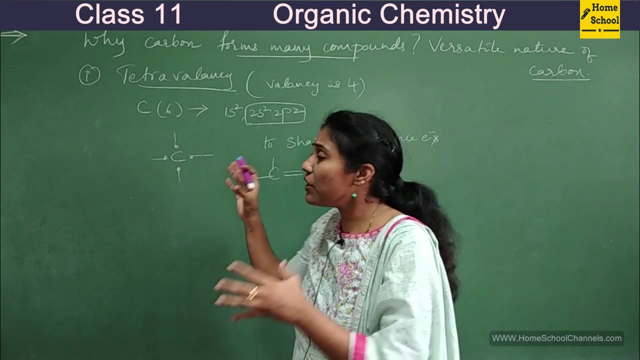 you will observe only four bonds. you see here one, two, three, four. you see here one, two, three, four. you see one, two, three, four. right, so all four bonds can be single, or it can have a double bond, or it can have a triple bond. okay, so this nature, we will call it as tetravalency nature. okay, fine. 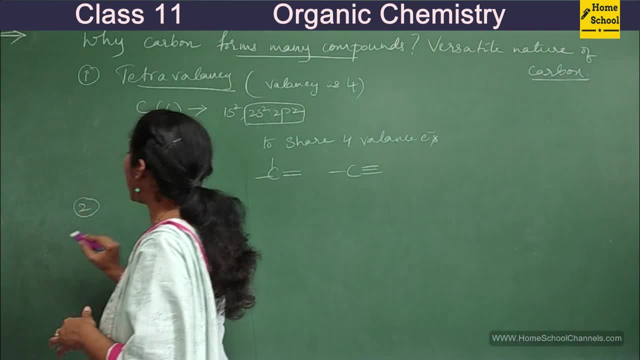 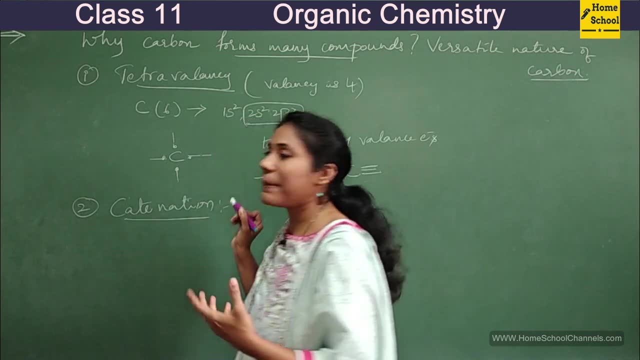 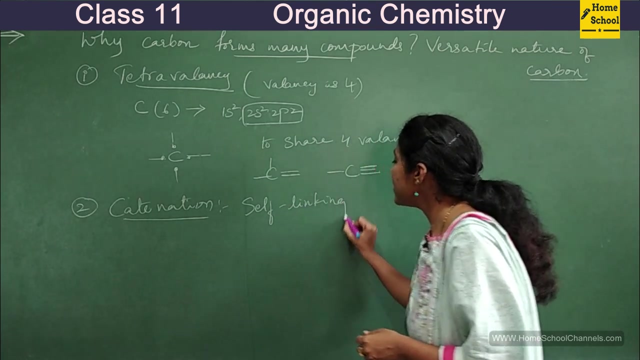 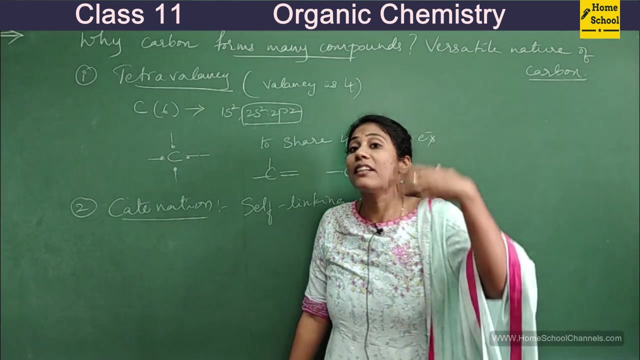 and coming to a second special property of carbon, that is catenation. so this is very, very important property we have studied in our basic classes. also, catenation is nothing but self-linking capacity of carbon, self-linking capacity of carbon, right, so carbon can link with carbon atoms itself. 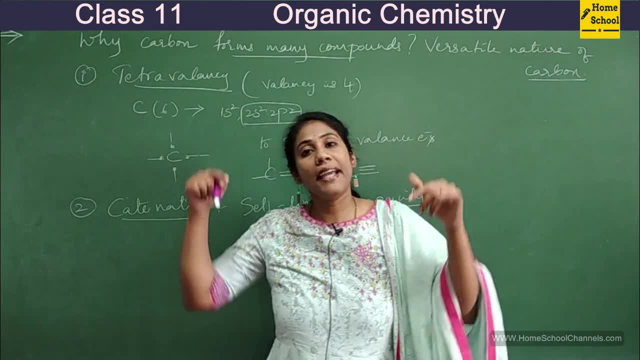 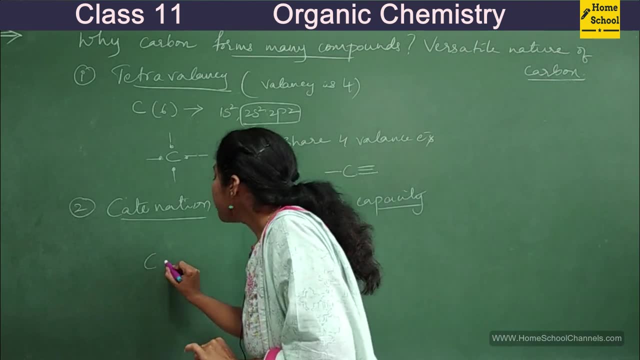 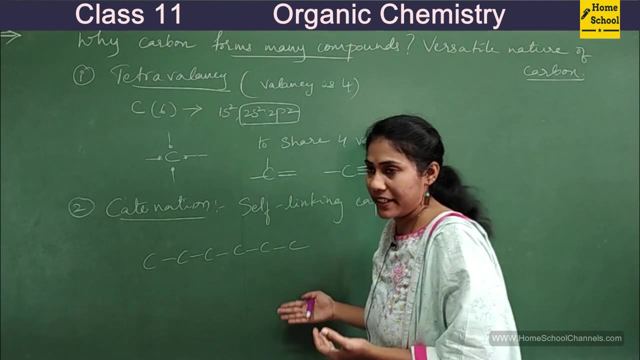 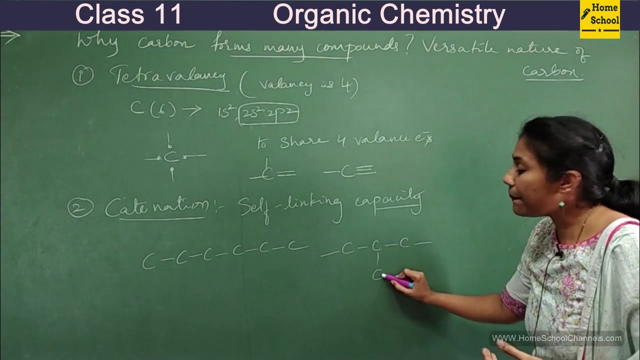 to form a long chain, to form a cyclic chains, or it. it can form various shaped chains, isn't it? say, for example: uh, you know, carbon links with other carbons and forms a long chain. we call it as long straight chain, okay. or you know, you can observe bonding something like this: right, so a long chain with a branch, so this we will call it. 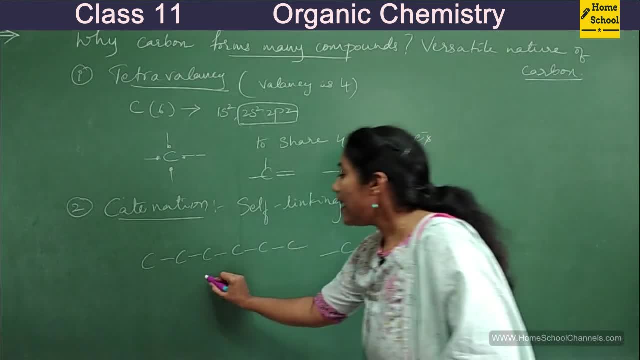 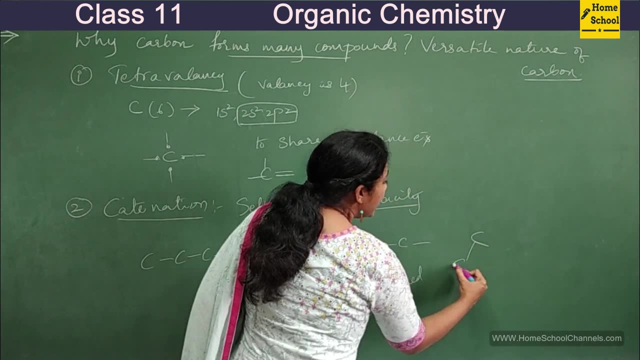 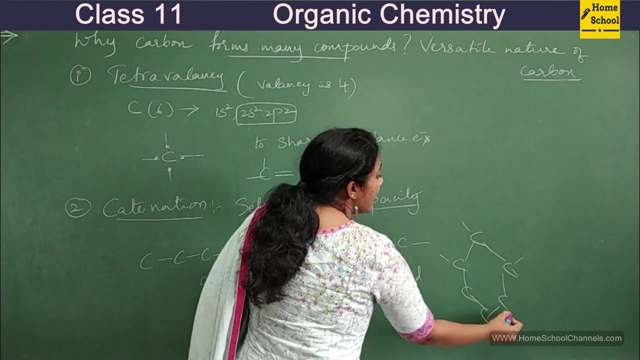 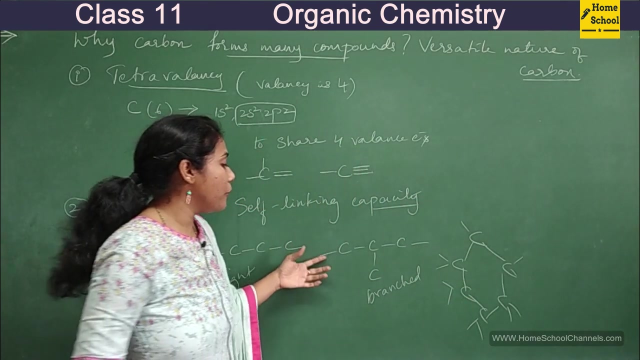 as branch to chain. so this is a straight child, right. and carbon can link with its own carbon atoms and form a cyclic chains. also like this, carbon can link in a cyclic manner, right? so you know, it can form a straight long chain, it can form a branch to chain or it can form a cyclic structures. 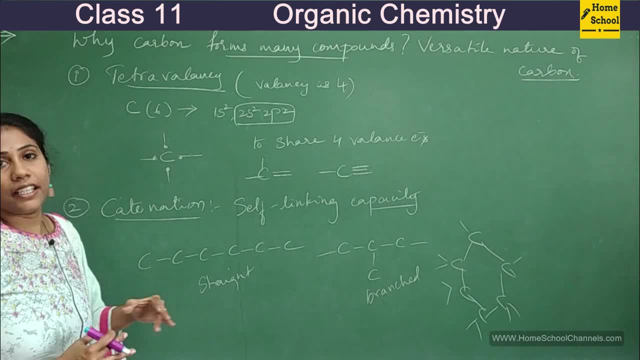 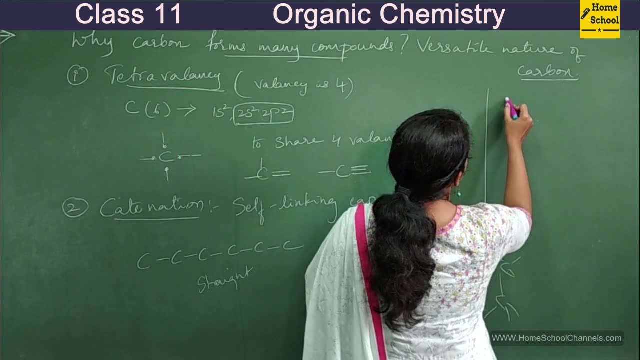 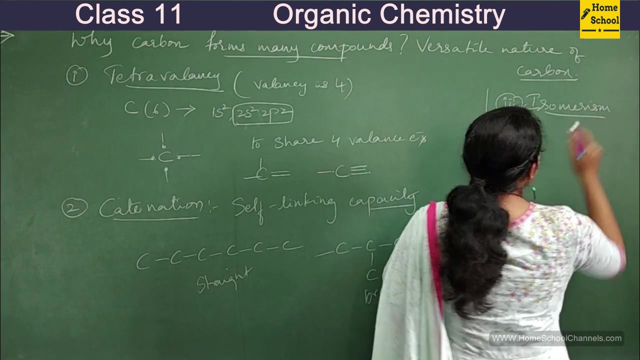 right. so this nature, we will call it as catenation, second important special property of carbon. and coming to the third property, that is isomerism. carbon shows isomerism. so what do you mean by isomerism? carbon compounds exist as isomers, isomer. 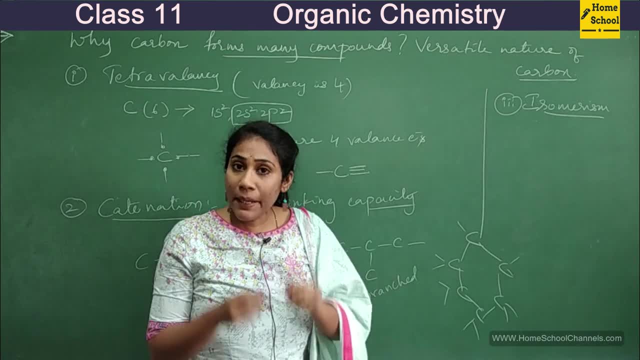 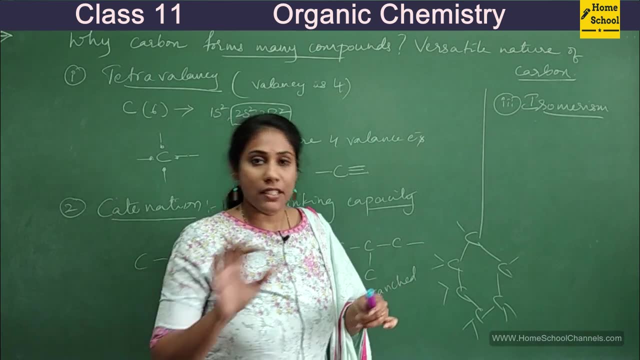 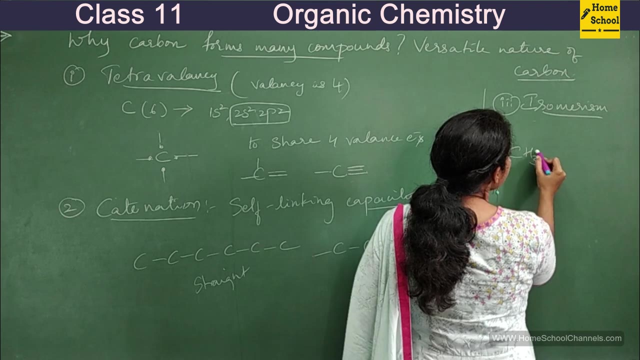 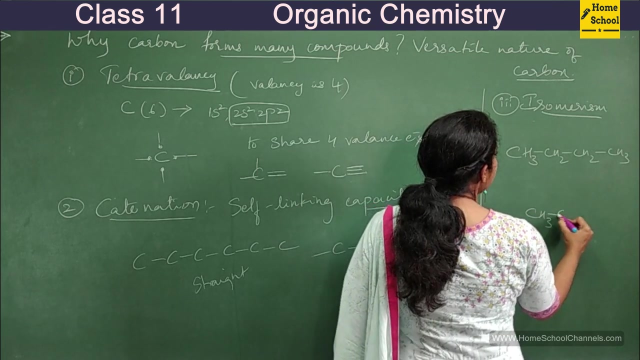 in the sense compounds which have same chemical formula, okay, but different structures or, you know, different chemical properties, for example. don't worry, uh, understand this particular example. see, i have a compound ch3, ch2, ch2, ch3, okay, so i have another compound, ch3. uh, this is what, don't worry. 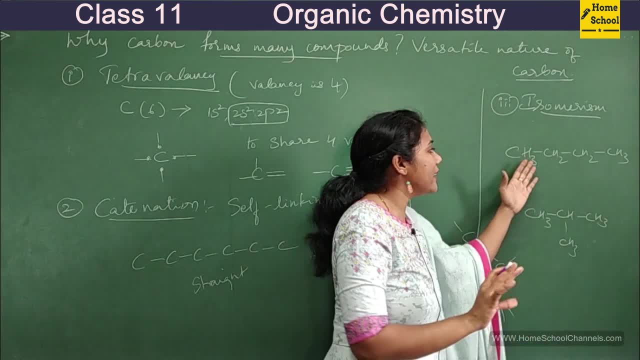 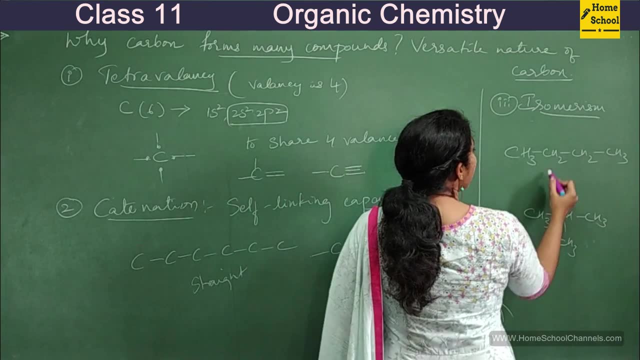 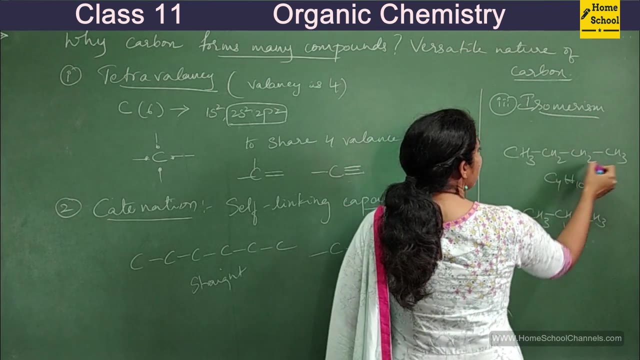 about, uh, their names, their properties, they are not the same, so they are not the same. so they are not the same. they are the same, so they are not the same. so these are the types of compounds which you've mentioned here. i think 1996. so this is just you know. you just write it my name's, yeah. 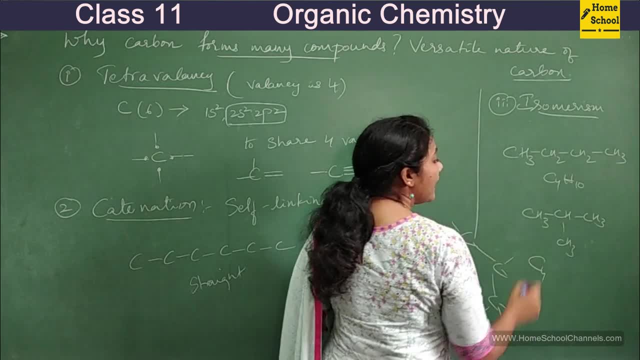 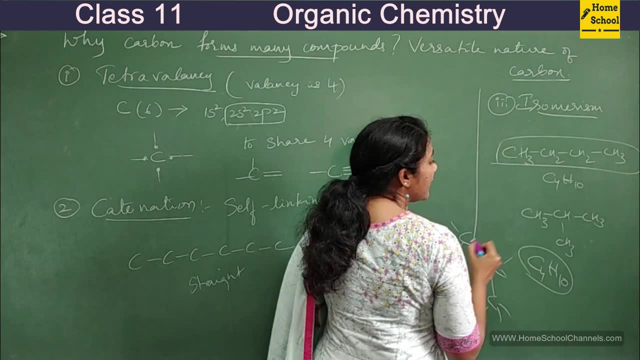 so the structure we will learn now we will talk about that actually literally from the uh, from the heart condition. so just think like that, cause you can reef liverbank, give you some some arguments. so this is the picture at all. this is everything you with life. you know there is no. 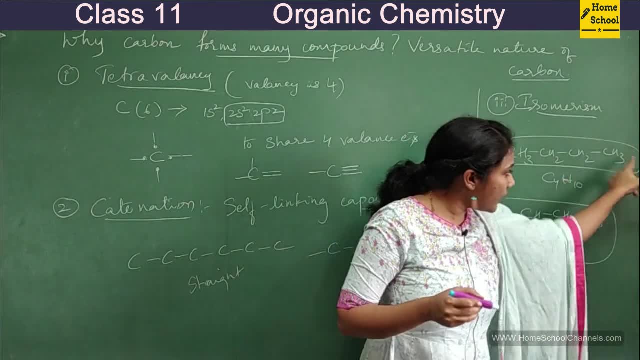 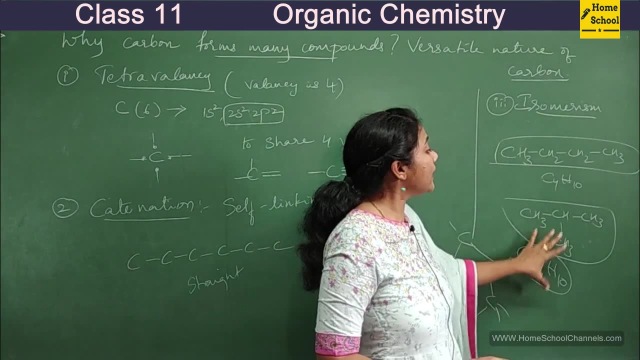 so i have an idea now i will give you the picture at all. you with life, you will give it into the. this is another organic compound. this was having a straight shine. this is a branched one, right? okay, molecular formula is same, but both compounds are very much different. okay, so this compound behaves. 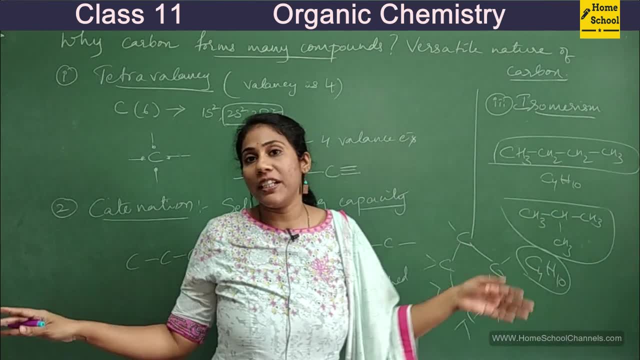 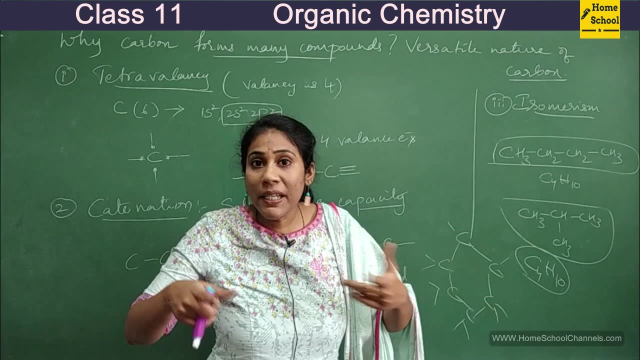 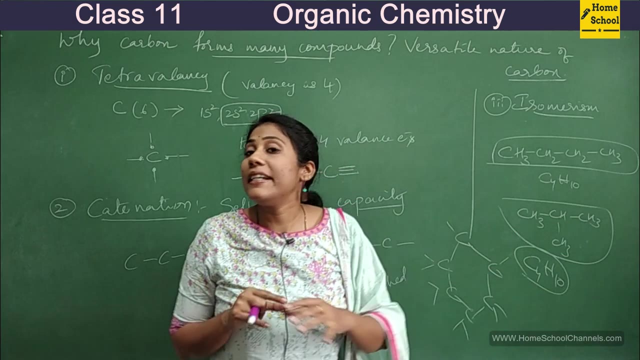 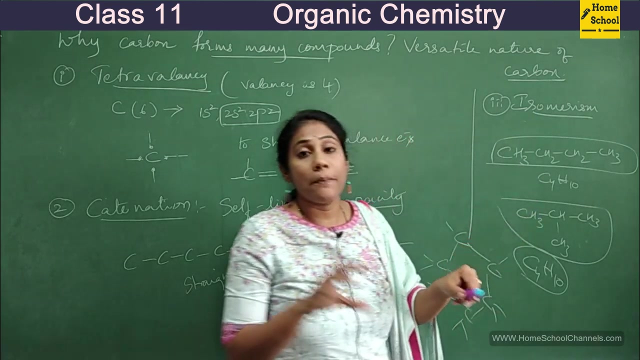 in a different way and this behaves in a much different way. there is no comparison between the properties of this compound and this compound. what is similar? molecular formula is similar. what is different? their physical and chemical properties are entirely different. okay, so carbon compounds have this kind of isomerism. they will show this kind of isomerism. this is one of the 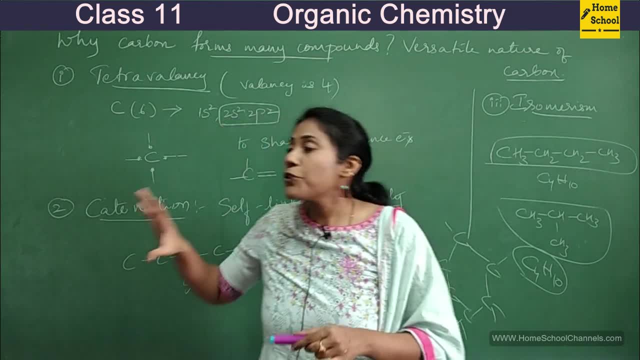 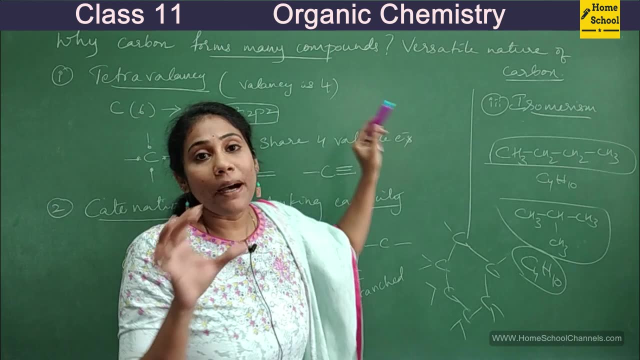 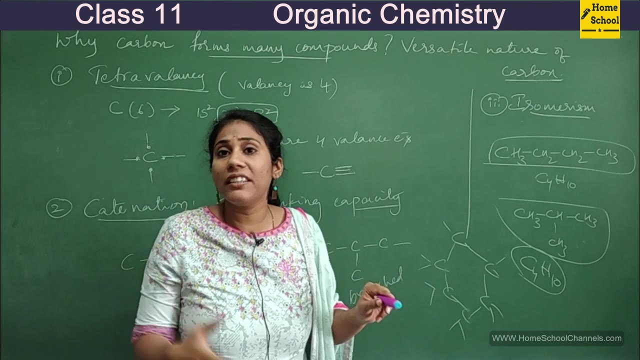 different property of carbon. okay, so mainly three reasons why carbon is special and why carbon is forming many compounds in our nature. i told you know we have around five million carbon compounds so far and every year 30 000 compounds are being synthesized newly, right, so why these? 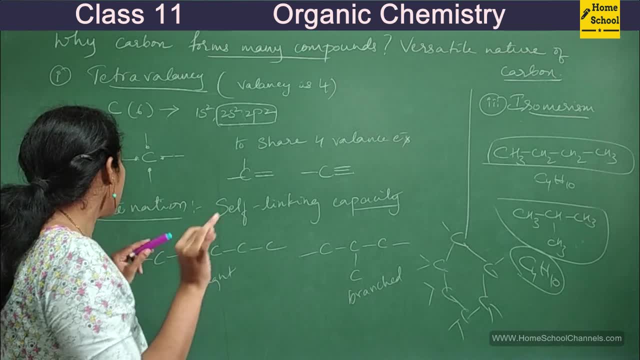 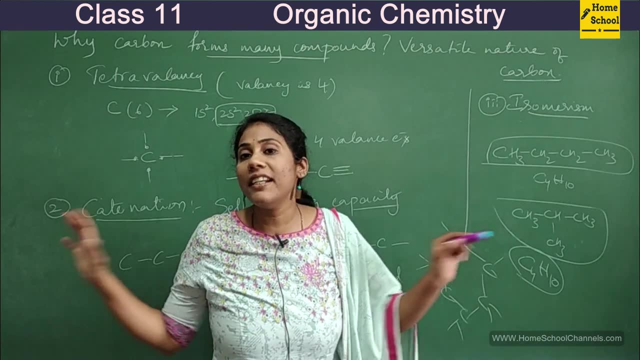 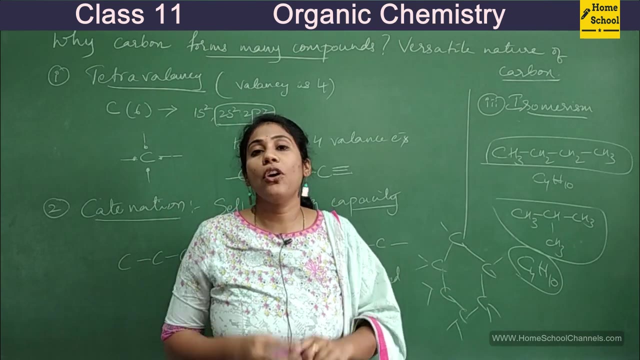 crores of compounds are being manufactured every single year is because of mainly these three properties. okay, so this is the versatile nature of carbon. now let us understand the type of bonding that you will observe in organic compound. okay, so here i will teach you the concept of. 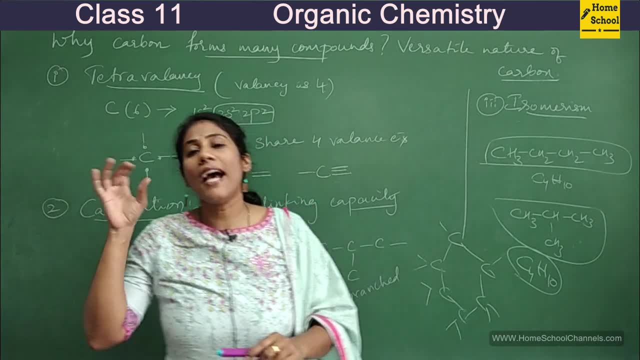 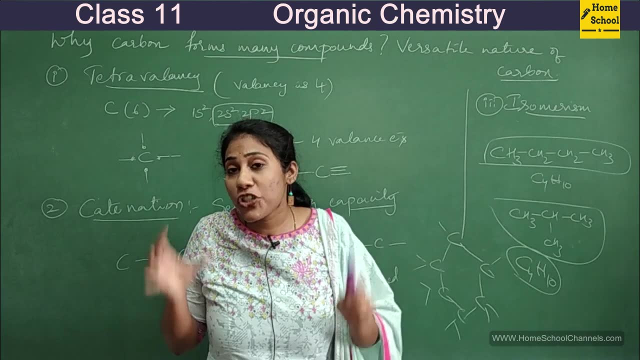 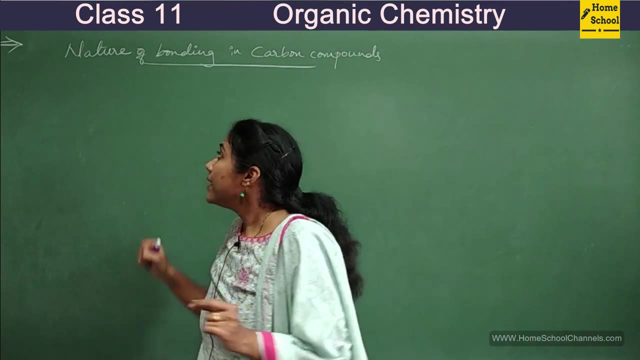 hybridization also okay. so more detailed aspects of hybridization you will study in chemical bonding, but now i will teach you how much ever is essential to understand the structure of organic compound. that much i am going to teach you see, guys, the type of bonds that you observe. 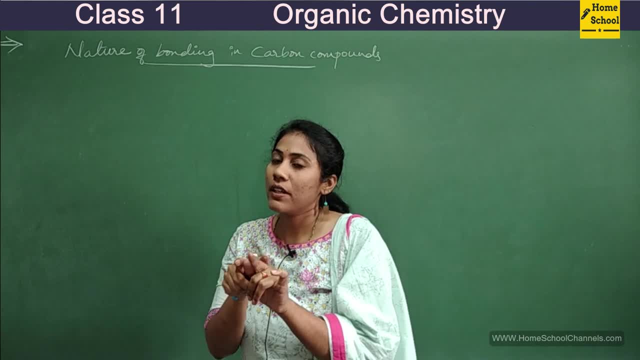 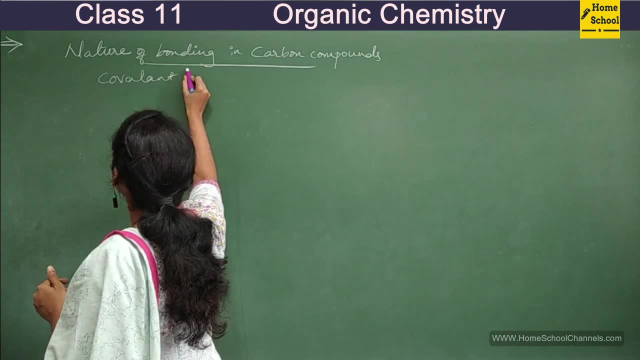 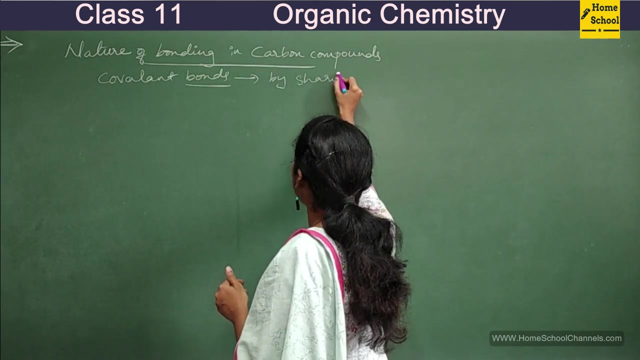 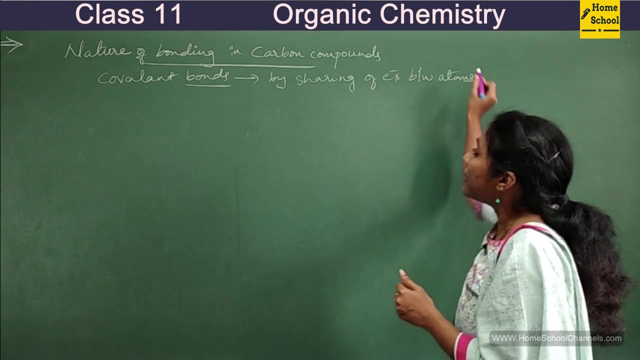 in every single organic compound is covalent bonds. so remember this point, very, very important, and the type of bonds you will observe is covalent bonds. So how are covalent bonds are formed? It is by sharing of electrons, right? Sharing of electrons between the atoms leads to the formation of covalent bonds. Okay, 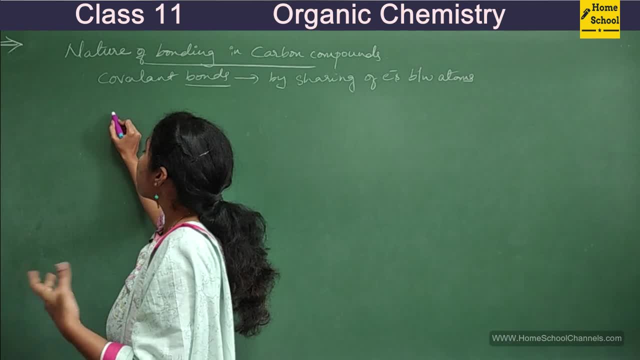 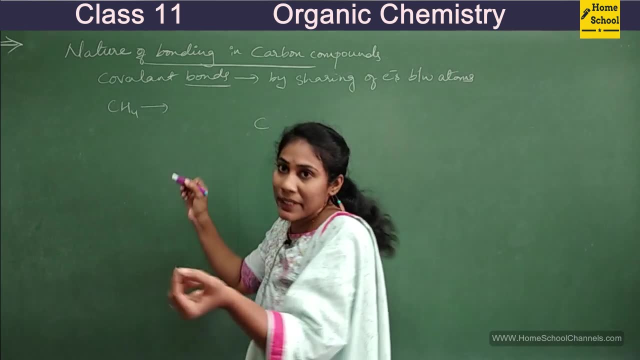 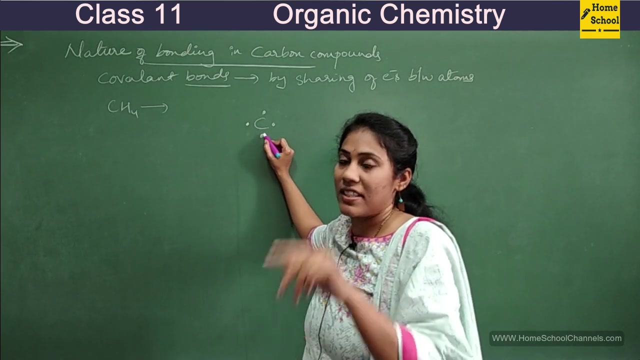 so in the lower classes we have studied. you know the dot structure for methane, right? So how did methane molecule formed? Say you will mention carbon. Carbon has four valence electrons, right? So always, which electrons can be shared Valence electrons, that is, the electrons present in the last shell. So it has four valence electrons and hydrogen has one valence electron. This is one hydrogen, this is second hydrogen, this is third hydrogen and this is fourth hydrogen. right, So these two electrons are shared between carbon and hydrogen, So that this hydrogen gets stability. right, So it will have two electrons around it, so that it 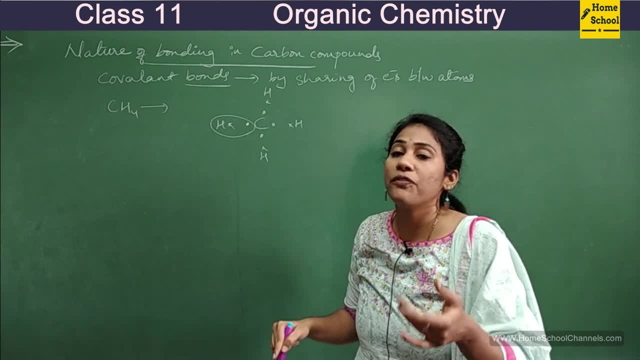 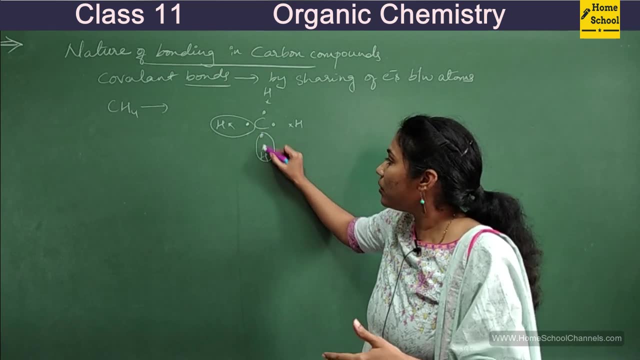 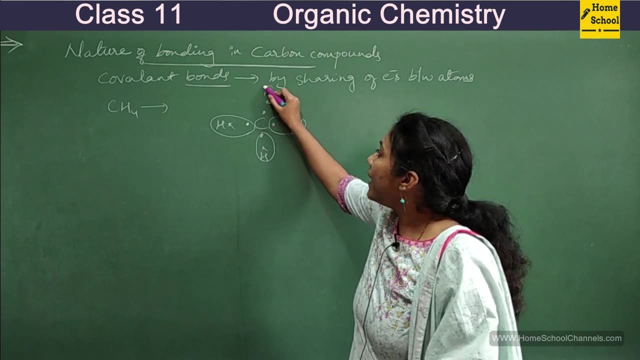 becomes stable. It just shows the electronic configuration of helium. so it is stable. And you know these two electrons are shared between carbon and hydrogen, So it's like these two electrons belong to carbon also and they belong to hydrogen also. So this is how all hydrogens are becoming. 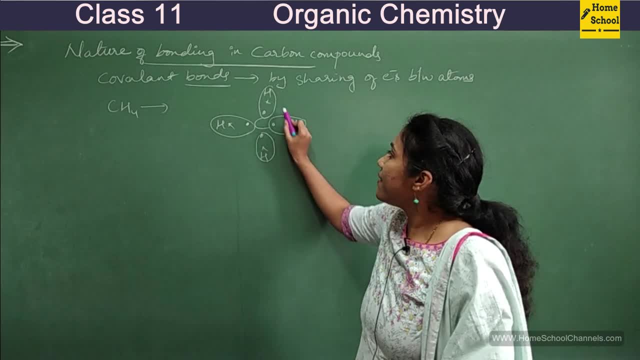 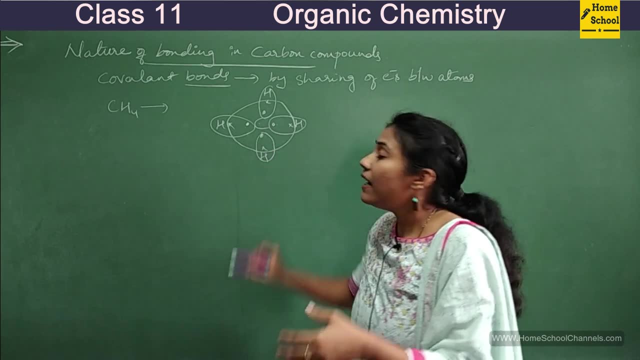 stable And carbon: 1,, 2,, 3,, 4,, 5,, 6,, 7,, 8, right? So this is how you will show the electrons present around carbon. So this way, carbon has eight electrons around it so that it is getting stability right. So this one, how do you show? 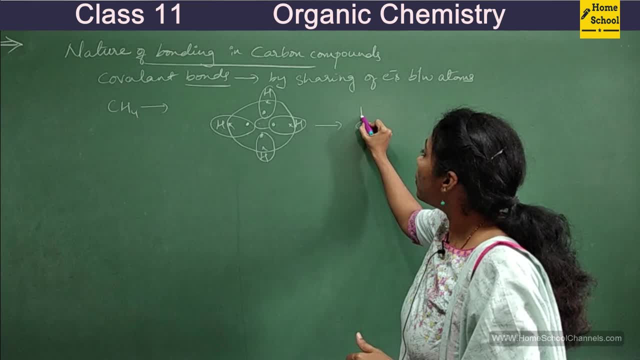 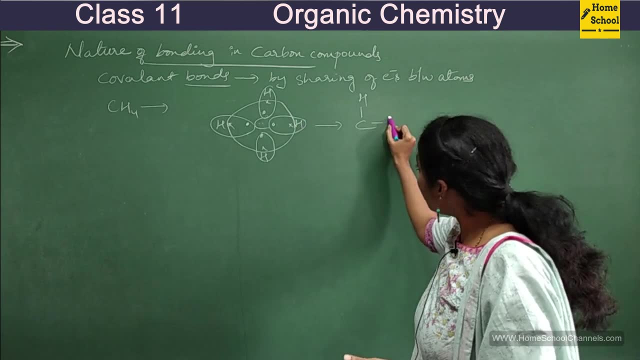 Between this carbon and this hydrogen two electrons are show, two electrons are shared. So you will write that as bond. So between this carbon and this hydrogen, two electrons only shared, So one bond. So here also one bond. here also one bond. So this is how you will. 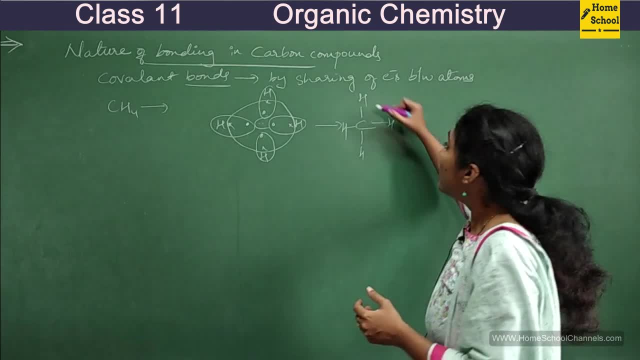 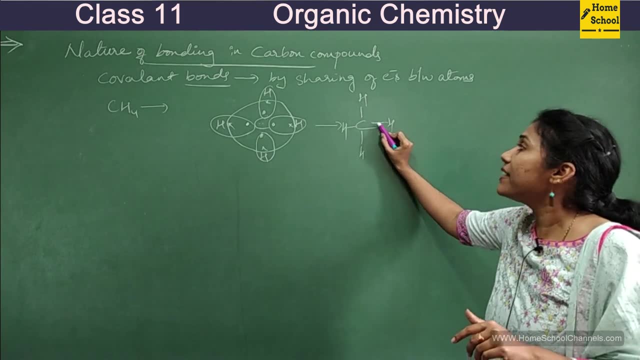 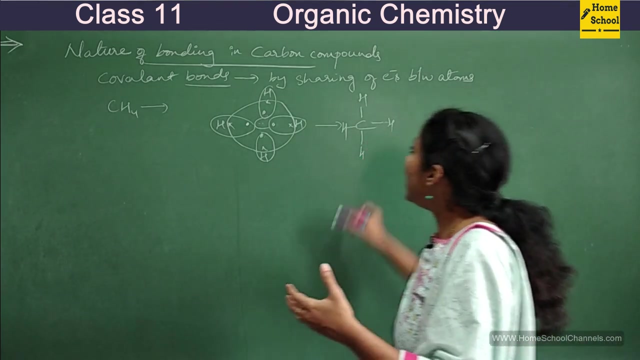 write the structure of methane right. So here, when one pair of electrons are shared, you will write one bond. This is one covalent bond. This is another covalent bond, third covalent bond, fourth covalent bond. So this is how you will show how electrons are shared between carbon. 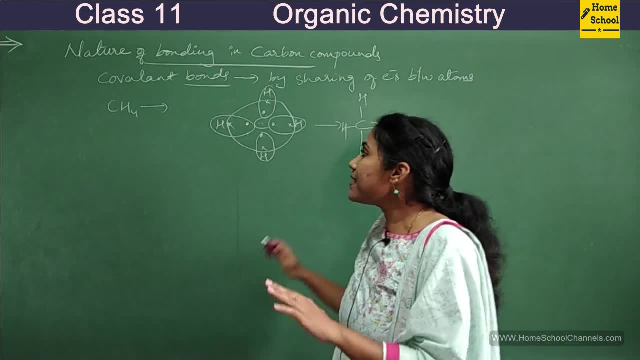 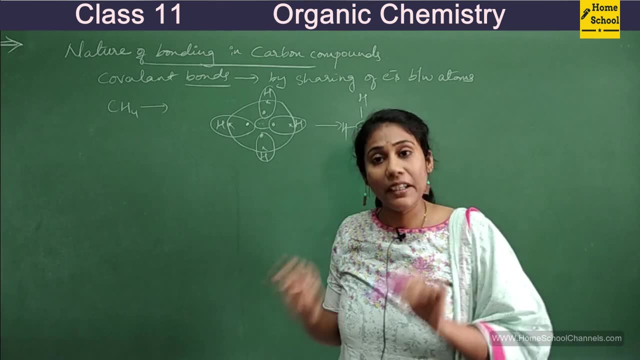 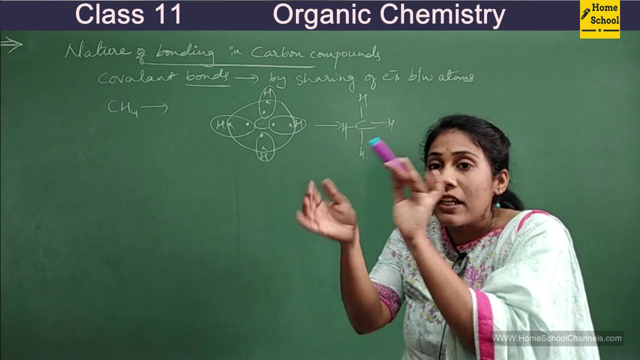 and four other hydrogens. okay, So this is a basic way of learning covalent bond, But actually speaking, in the chemical bonding chapter we will learn that covalent bonds are found when atomic orbitals overlap. So when do the electrons are getting shared between this carbon and 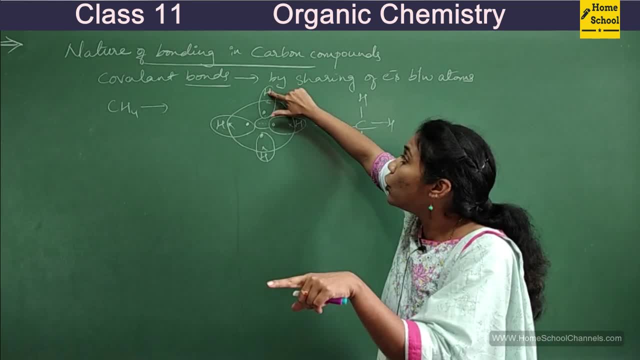 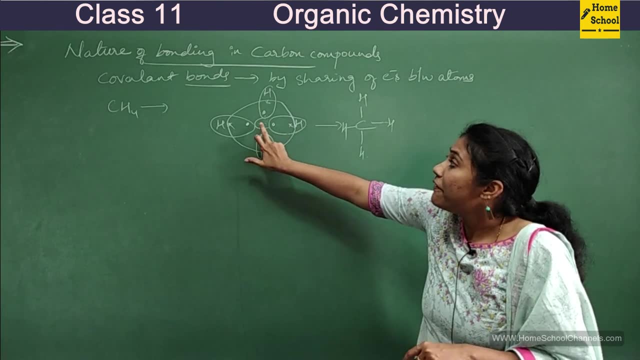 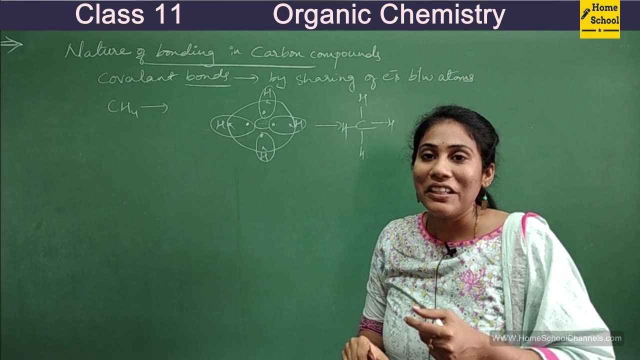 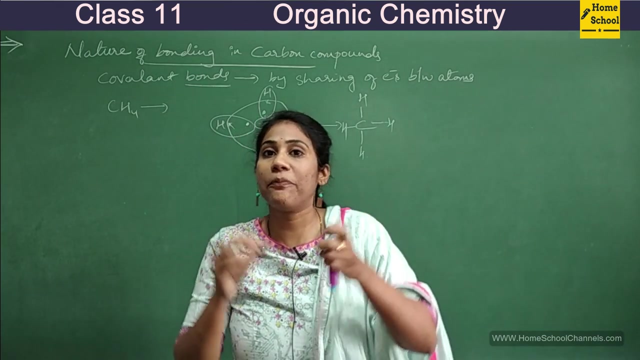 this hydrogen When carbon's orbital overlaps with hydrogen's orbital. When do sharing of these two electrons takes place? When carbon's orbital shai ah with hydrogen's orbital. Okay, So covalent bonds are formed when atomic orbitals overlap with each. 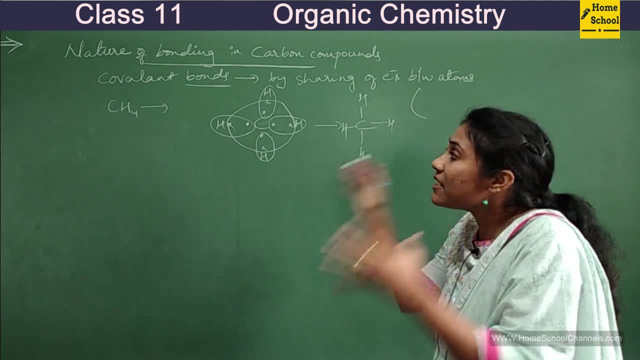 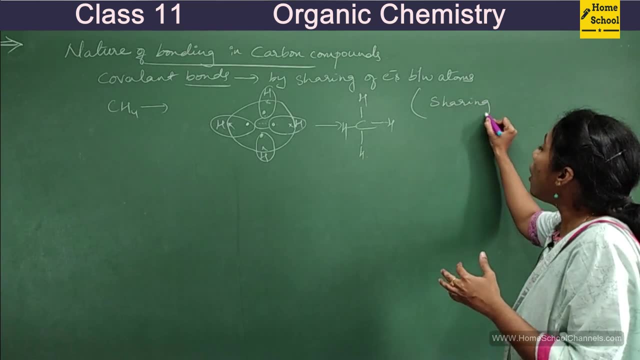 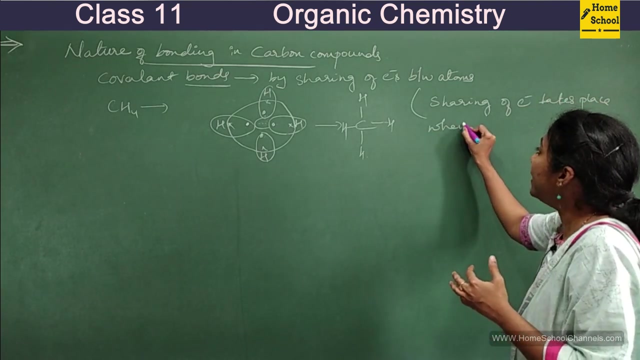 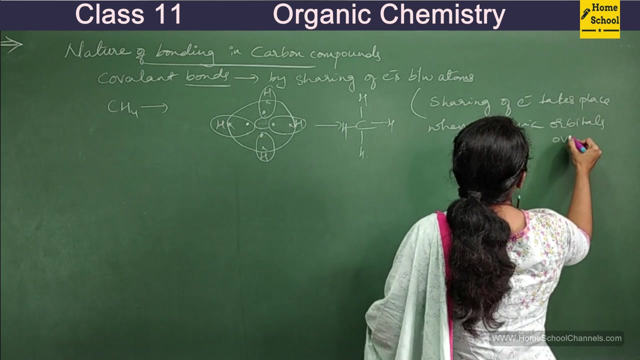 other. Okay, So I am giving much a standard definition for covalent bond. actually, You know, covalent bonds means sharing of electrons takes place, takes place when when atomic orbitals overlap. Atomic orbitals overlap. Okay, You see, here I am showing you how this atomic orbitals 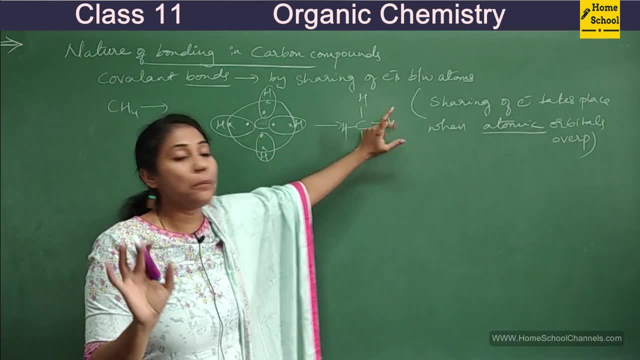 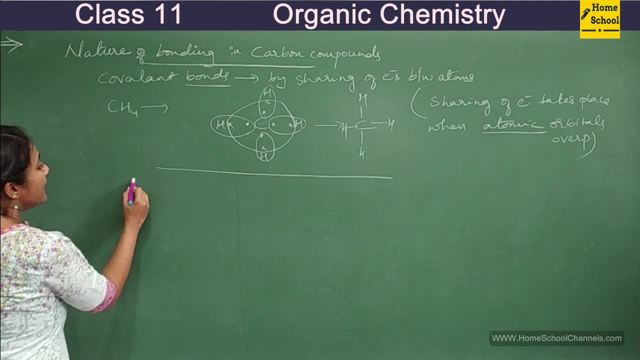 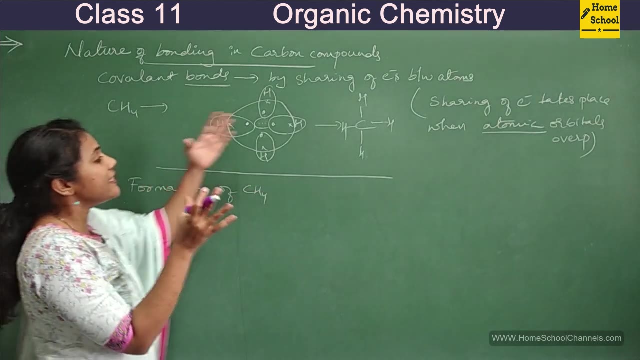 can overlap with each other to form these covalent bonds. Okay, So, observe carefully, guys. this is very, very, very important. Okay, Fine, So I am explaining you the formation of formation of CH4.. Okay, We know how this is formed Basically. we studied like this in our class 10.. But now we are going to study in a 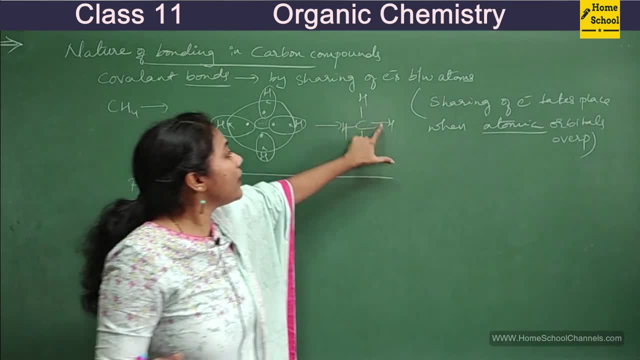 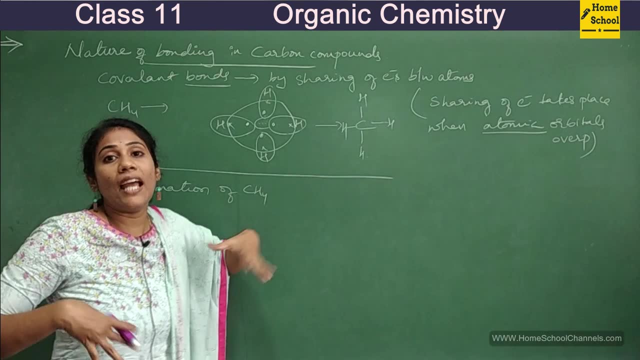 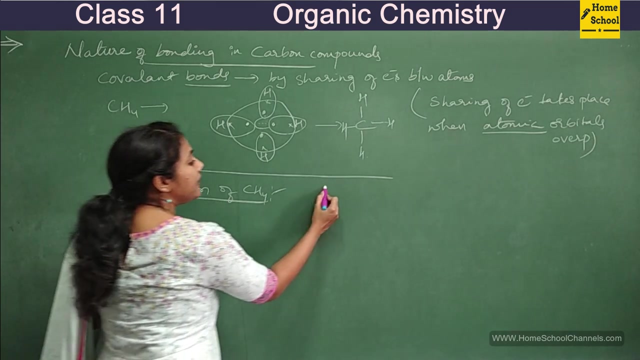 detailed way. Okay, So actually these bonds are formed when atomic orbital of carbon overlaps with atomic orbital of hydrogens. So how that overlapping business takes place, That's what we are going to learn. Okay, First, what I will write here is carbon's electronic configuration. Okay, So it is. 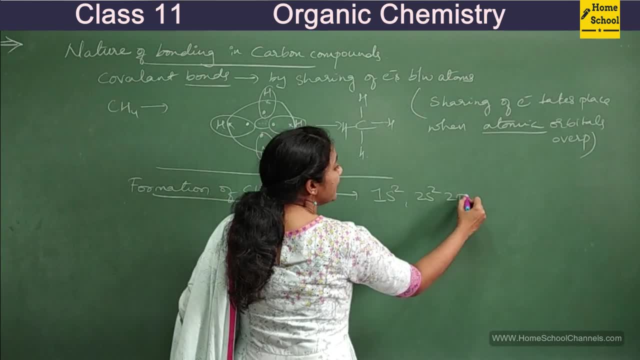 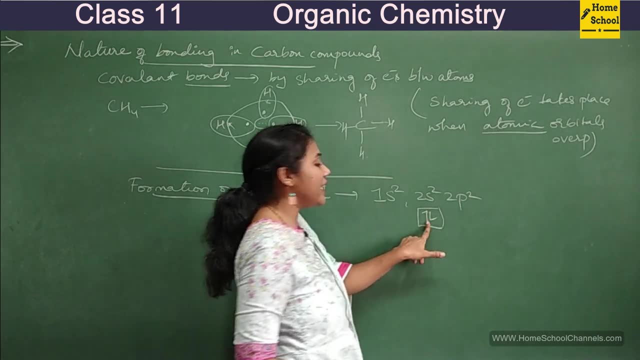 1S2, 2S2, 2P2.. Okay, So I will see. 1S S orbital is only one right, So one box. This way of writing electronic configuration also I taught you in atomic structure, So I told you you should have. 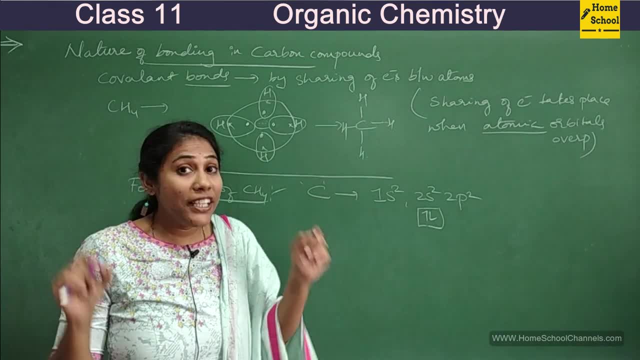 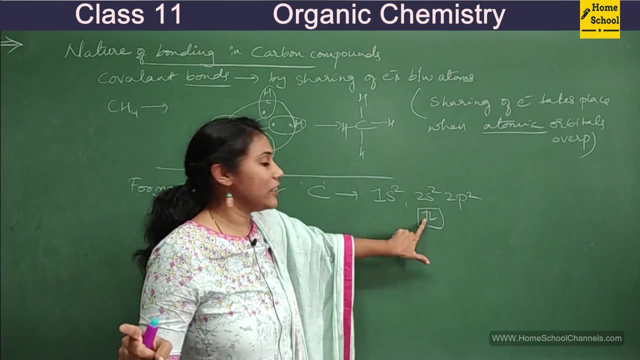 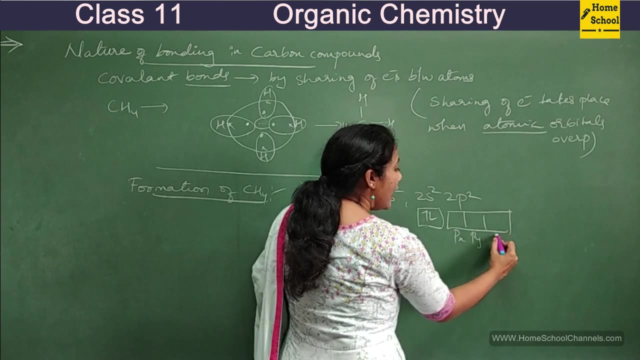 complete knowledge on atomic structure and chemical bonding. Video playlist links are on the screen provided in the description. go and check it out. s orbital is only one, in that two electrons are there. p orbitals are how many? there are three p orbitals: px, py and pz right. so two electrons one. 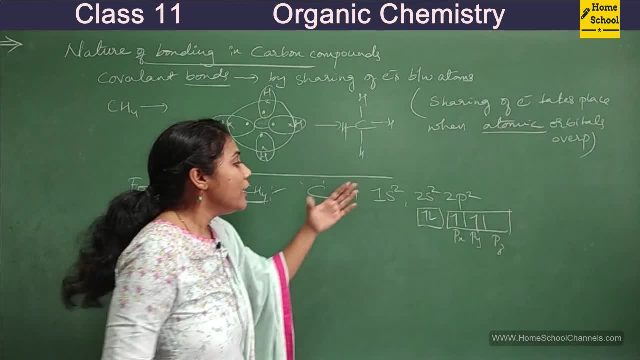 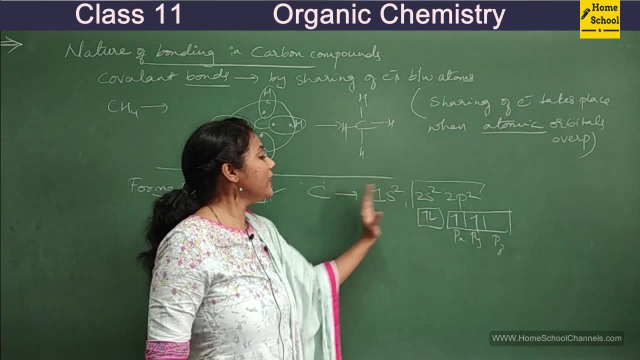 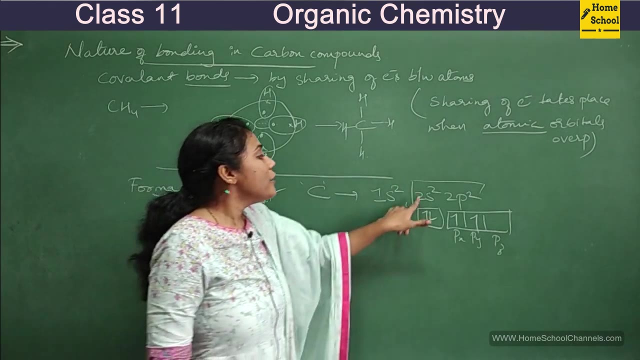 electron in px, the other electron in py. okay, so this is how the electrons are present in the valence orbitals. okay, so i'm not worried about this. orbital inner shell electrons will not participate in any kind of bonding. okay, so valence shell is second shell, so this is a s. 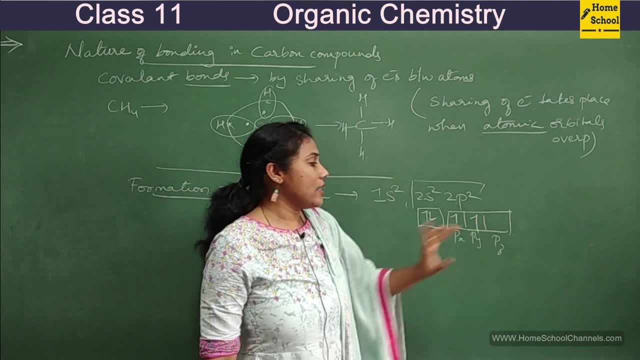 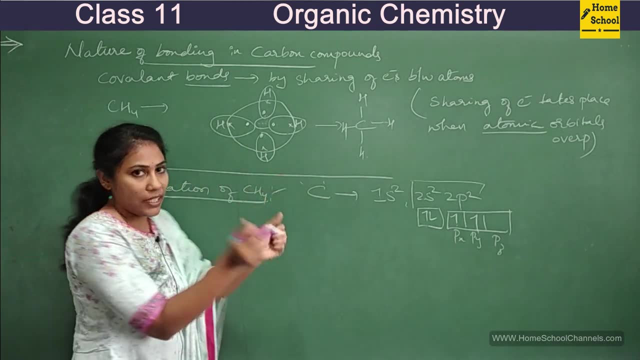 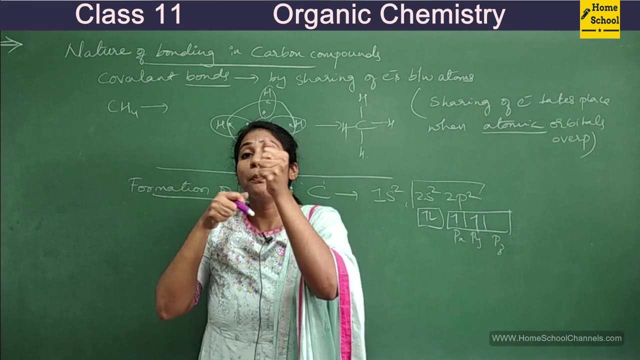 orbital, two electrons. p orbitals are three. two electrons are there, like this: okay. so now what happens is, you know, as hydrogens approach, carbon is here, okay, hydrogens are coming to make a bond. so as hydrogens approach to make a bonding with this carbon, this carbon will excite, this will get. 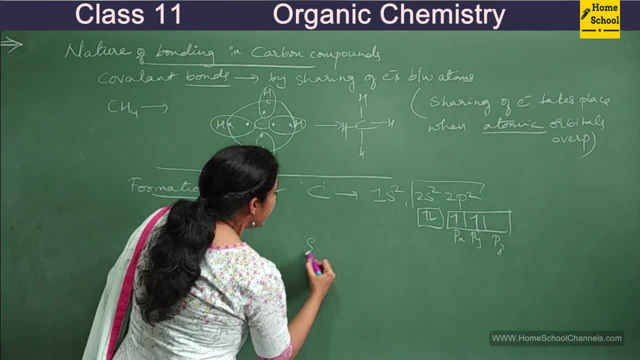 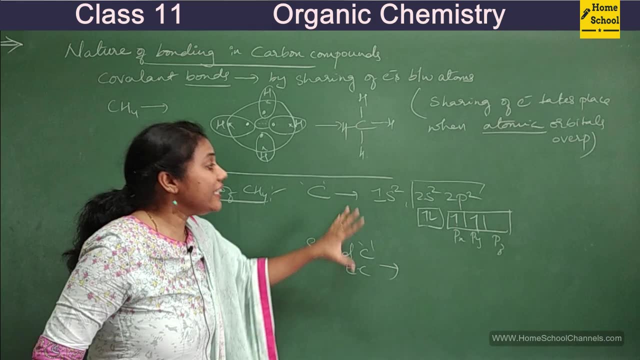 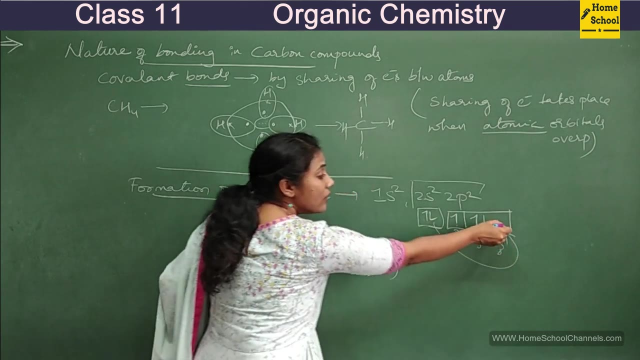 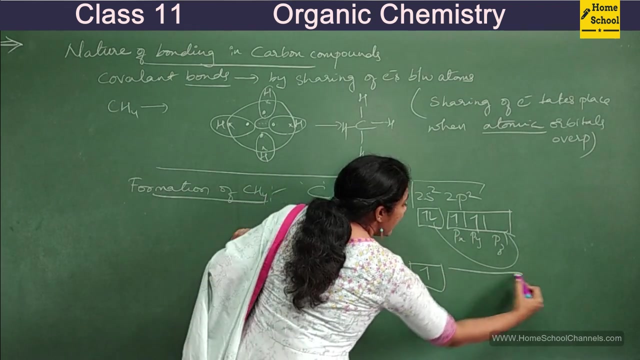 excited. okay, so i am writing you excited, excited carbons. electronic configuration: carbon: when it gets excited, one of the electron from s orbital will get shifted to pz orbital. so now the electronic configuration. last electronic configuration is like this: okay, so this is our 2s orbital. this is: 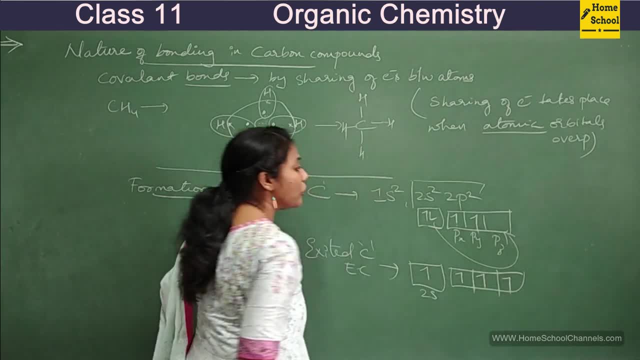 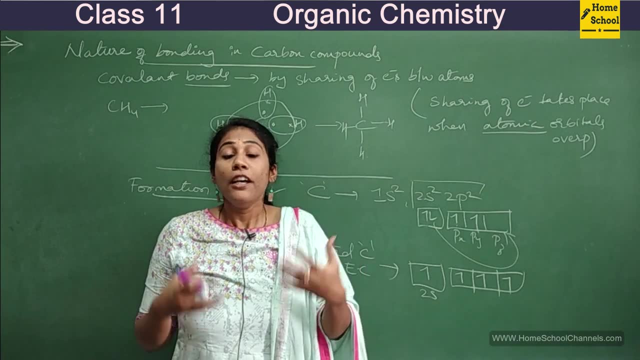 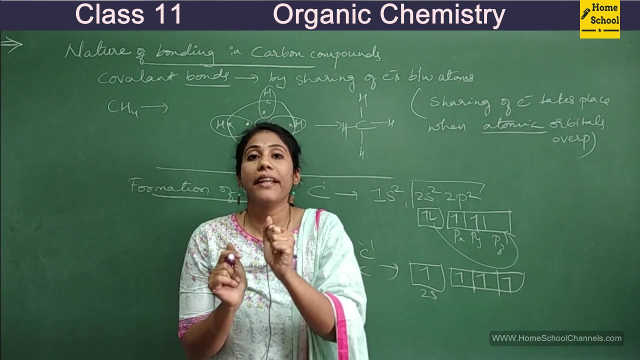 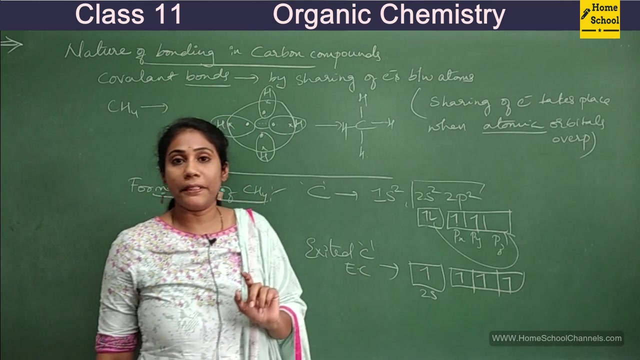 px. one electron: py1, pz1. okay, so when does this electron will go to this empty orbital? when carbon gets excited, okay. when does carbon gets excited? when four hydrogens are coming near to it to make a bonding? okay, fine, so now this is excited state. electronic configuration of carbon. 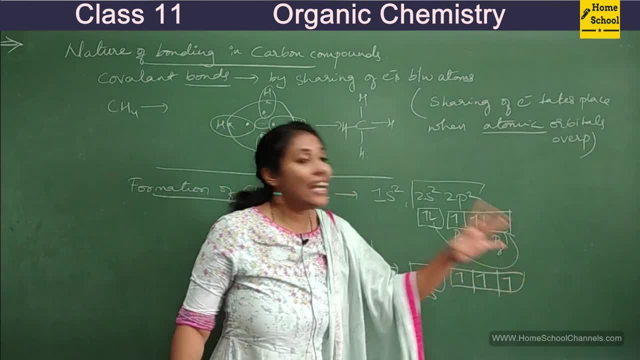 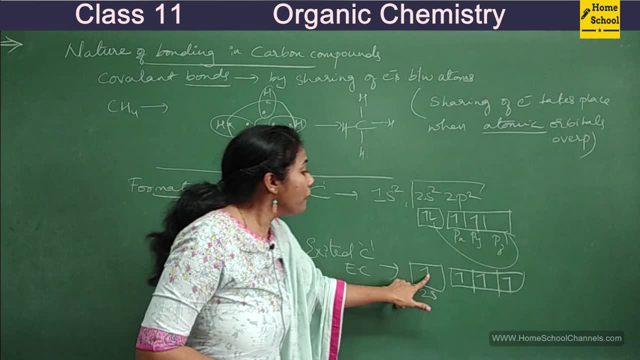 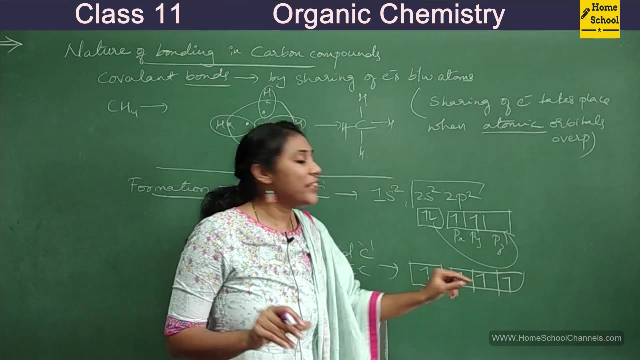 right. okay, so these are whatever atomic orbitals ready to overlap with each other. okay, so this is with hydrogen's atomic orbital. okay. so how many orbitals are there? four orbitals are there. okay, but actually all of them must have same energy, otherwise they are not ready to make a bonding. 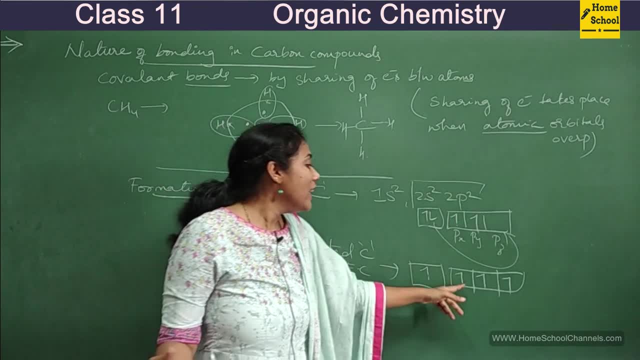 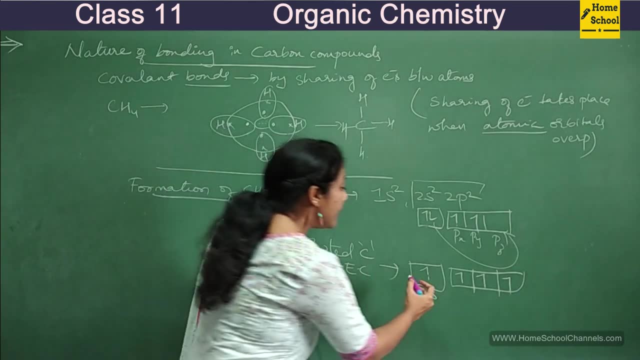 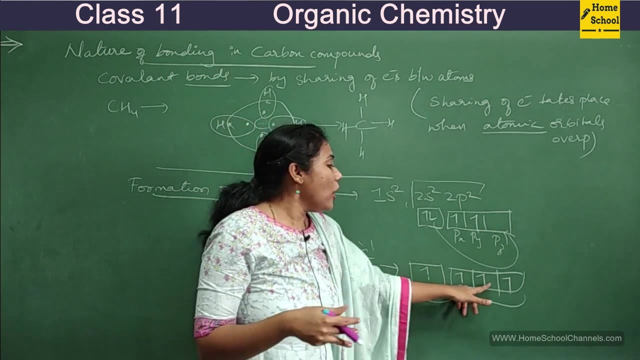 okay, so here, 2s orbital has different energy. these 2p orbitals have different energy. okay, so to make their energies equal they will combine with each other. they get mixed up. it's like they distribute their energy. okay, say, p orbital has much higher energy, s orbital has. 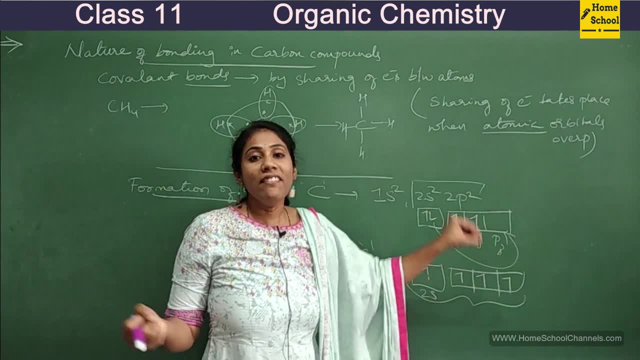 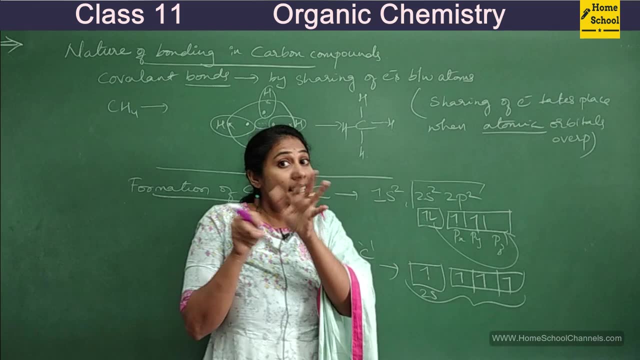 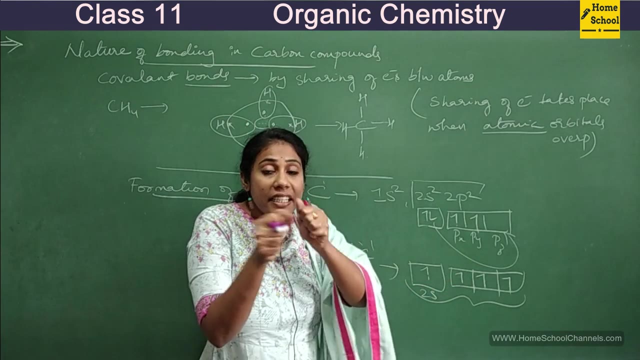 lower energy. so what do these p orbitals do? they give little of their energy to s orbital. okay, so you know, the mixing of orbitals takes place. during this mixing of orbitals, energy gets distributed equally. okay, four orbitals are getting mixed up to make their energies equal. 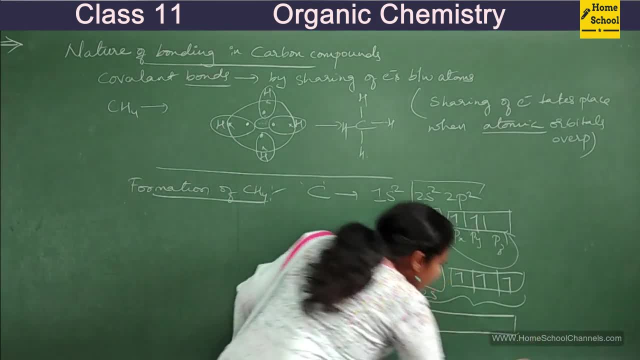 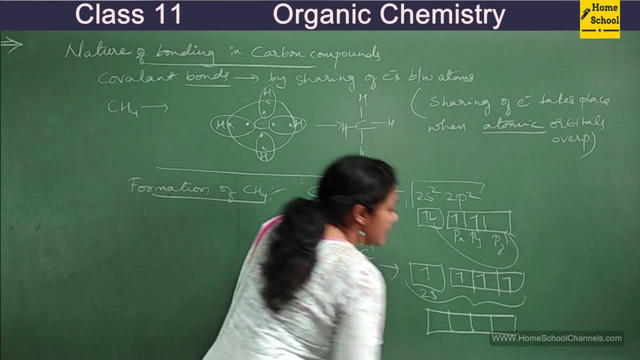 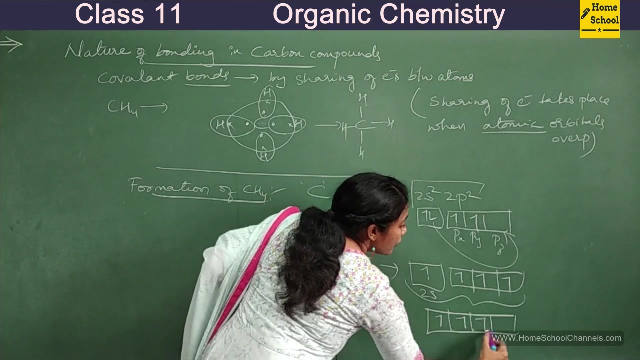 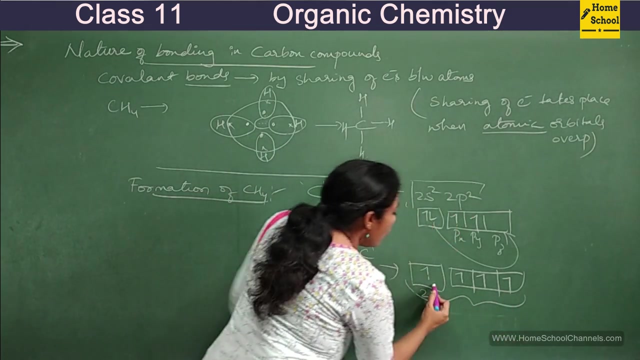 so we are getting four rejuvenated orbital, i am not telling new, four rejuvenated, four rejuvenated orbitals i am getting okay. so see, all orbitals. energy is equal now right. so which orbitals have combined here? one s orbital, right, let me do it. one s orbital and three p orbitals have combined to make their 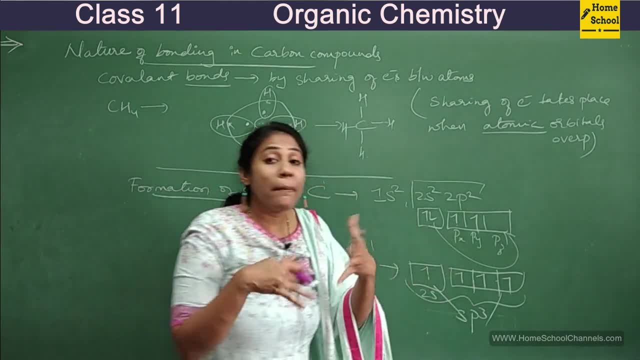 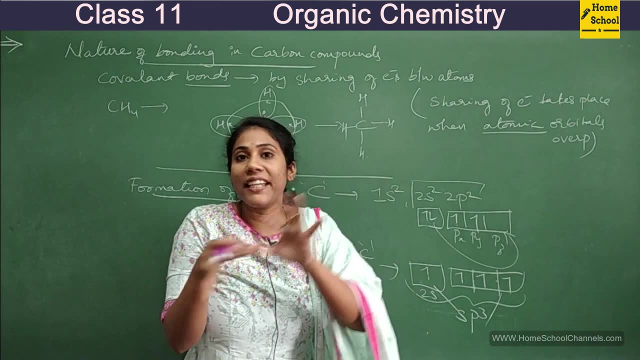 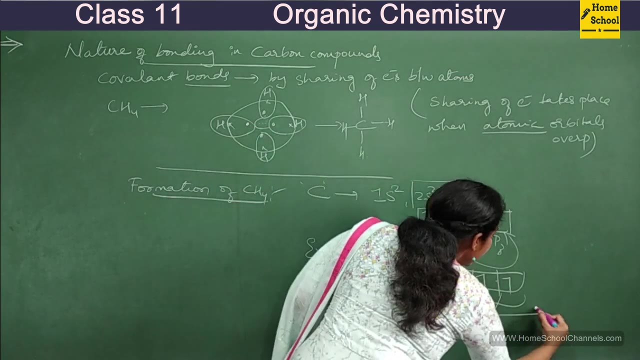 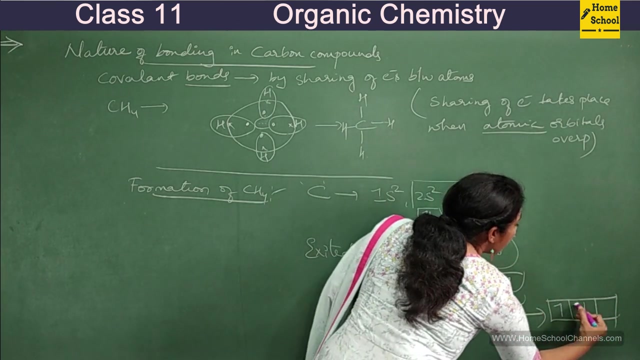 energies get equalized, right. so that is why this mixing of orbitals only we will call hybridization. okay, so four orbitals. if they get mixed up, four new rejuvenated orbitals are formed. okay, so now how many sp3 hybrid orbitals are formed? there are four sp3 hybrid orbitals are formed, each orbital. 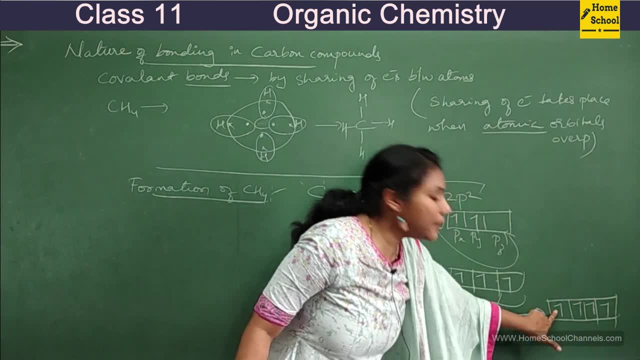 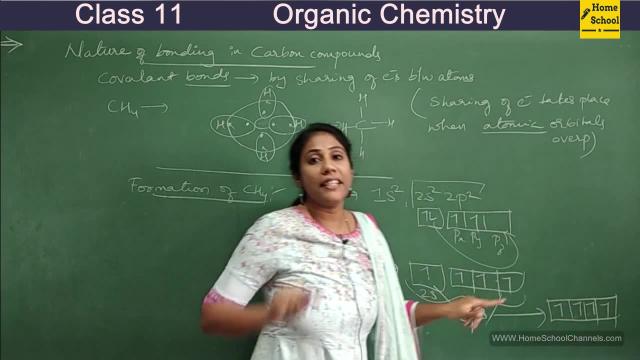 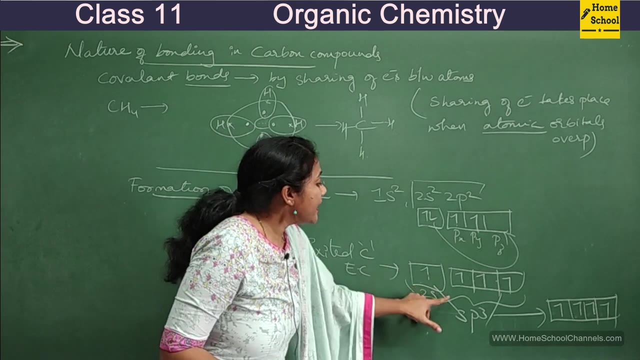 has one, one electron. this is one sp3 hybridized orbital. this is one sp3 hybridized orbital. this is second sp3 hybridizedorbital. third sp3 hybridized orbital. fourth sp3 hybridized orbital. okay, so now this, this is what we call. say, if somebody asks you, what is the hybridization of carbon in methane? 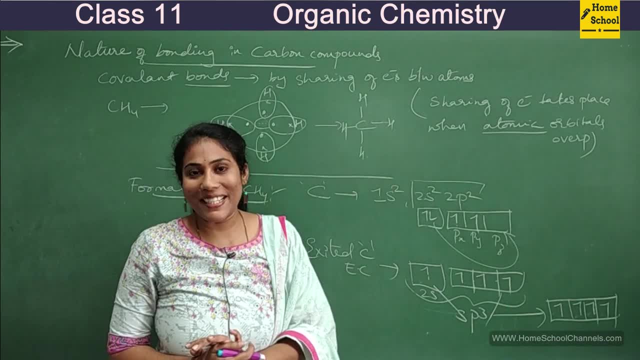 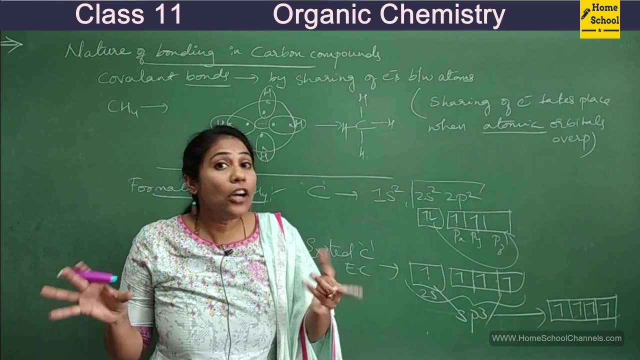 then your answer must be sp3 hybridization. okay, so carbon underwent sp3 hybridization. okay, why we call sp3? because 1 mild capital carbon must be الا two Bla-bla bar. so for one carbon it isойli the amount of él quantity that isன гоřh. 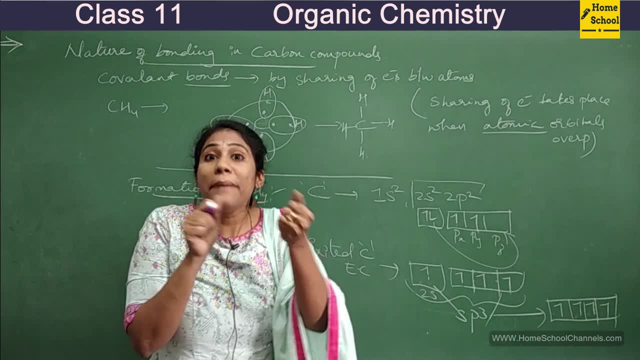 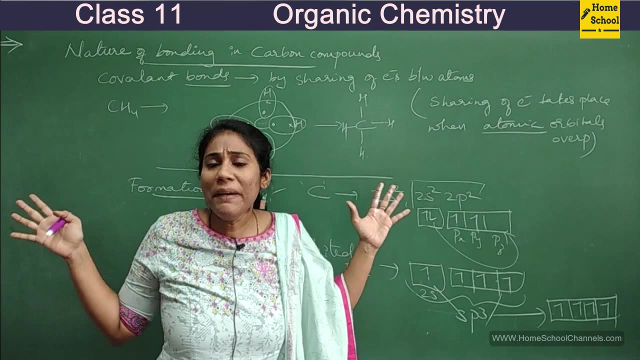 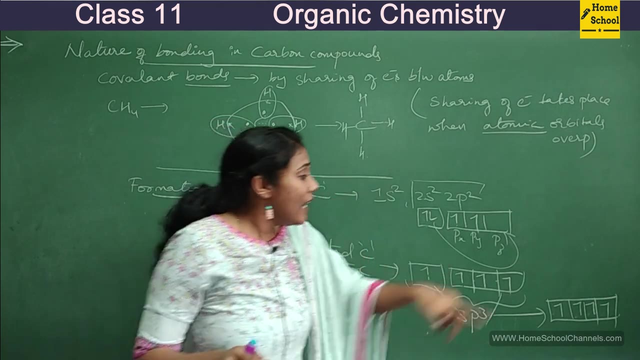 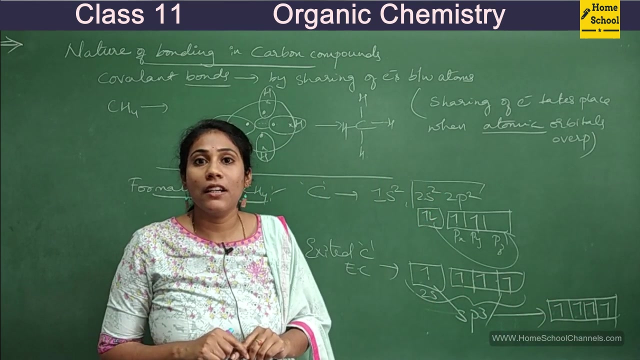 s and 3 p orbitals have mixed up with each other just to distribute their energies- equally okay. now they have become active orbitals completely are rejuvenated orbitals. now we call their name as sp3 hybridized orbitals. okay, there are four sp3 hybridized orbitals. okay, fine, so now this is. 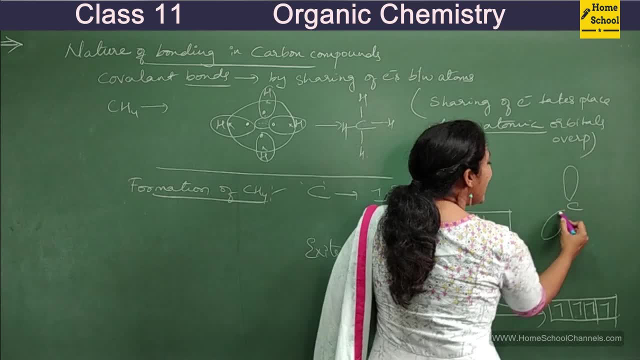 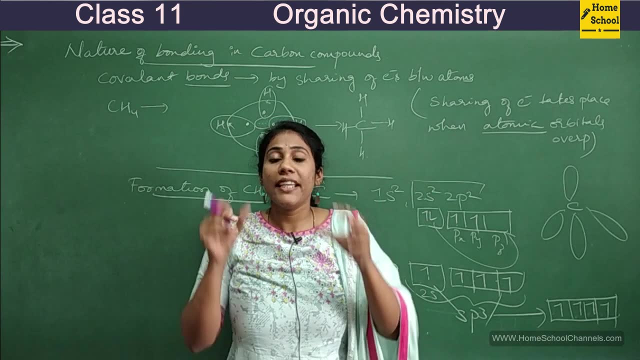 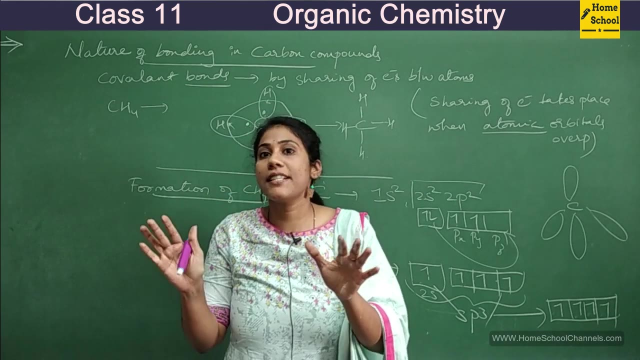 our carbon. so how do these? or orbitals are arranged around carbon, something like this: okay, orbitals are directed in certain position, they are arranged, they are like balloon, like structures, okay, so if you hold four balloons, how do you hold them? say, for example: see, i have 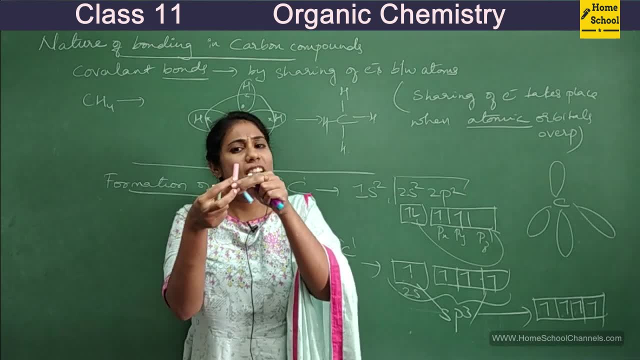 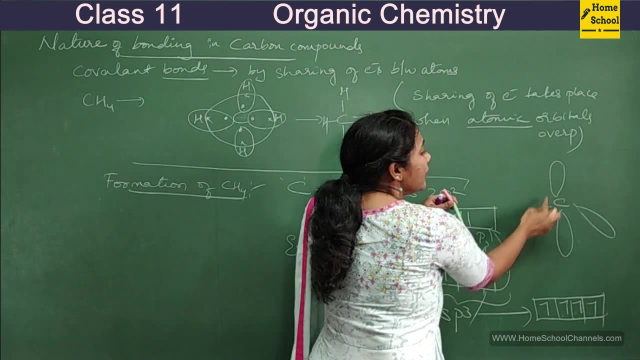 four chalk pieces if i have to hold them as far as possible. you know they should not be present very much near to each other when they are very much near to each other. you know they should not be present very much near to each other when they are very much near. 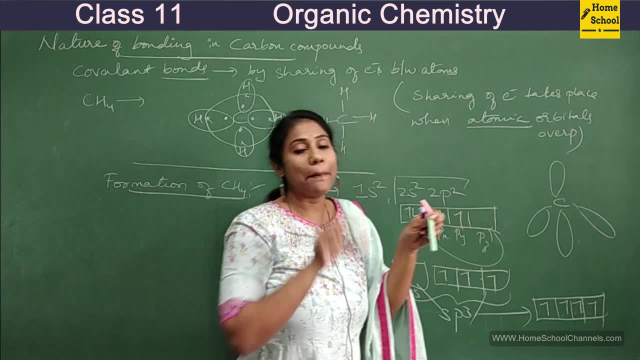 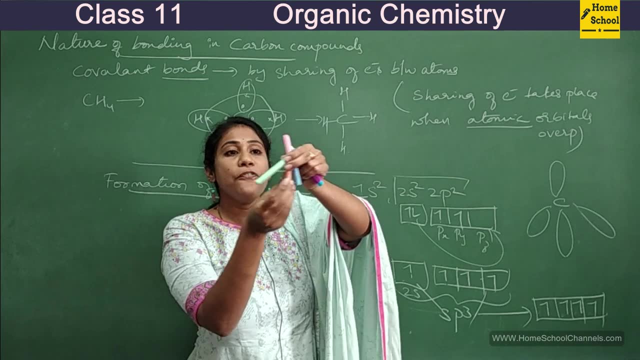 to each other when they are very much near to each other. when they are very much near to each other, they are with electrons, right? if they are near, you will observe the repulsion electron, electron negative, negative charge, so repulsion. so these orbitals are arranged as far as possible, right? 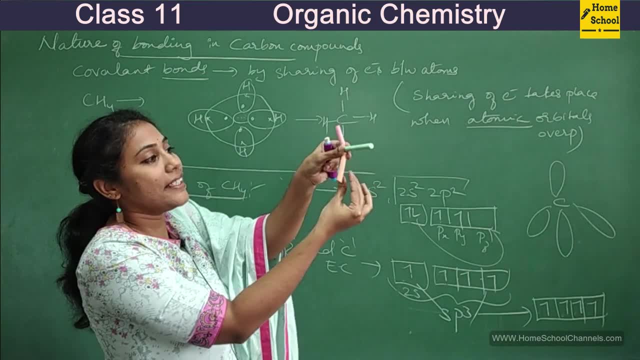 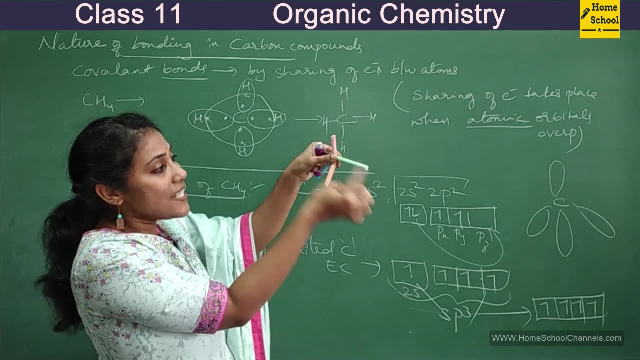 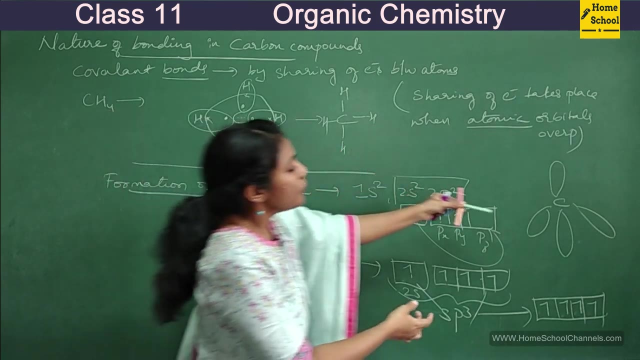 say four chalk pieces if i have, how do i direct them? how do i show them in different directions in space, like i should show them that there is as much distance as possible between them? okay, say one chalk piece like this, the other one like this, other one like this, right, so four. 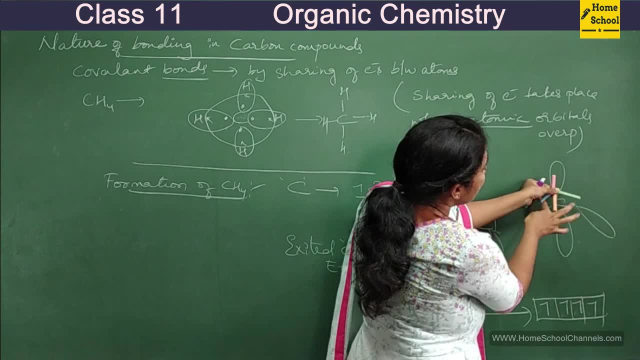 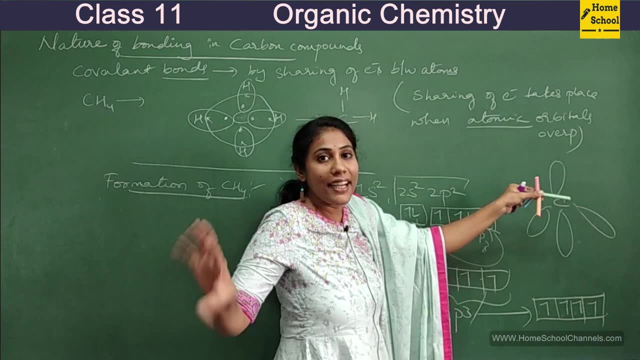 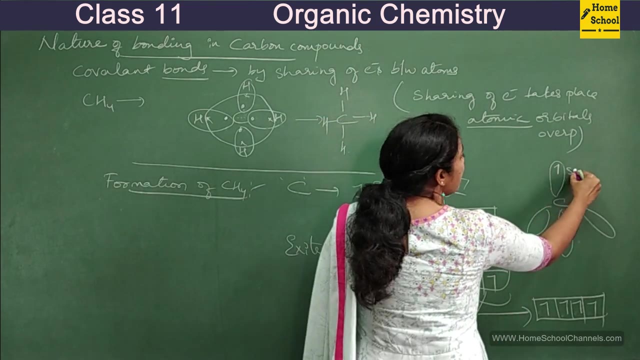 orbitals center carbon, is there four orbitals. the new orbitals, rejuvenated orbitals, have formed. you know, they are arranged in space something like this: okay, they are like balloon, like structures, okay, so each orbital has how many electrons? one electron, this is one sp3 hybridized orbital. 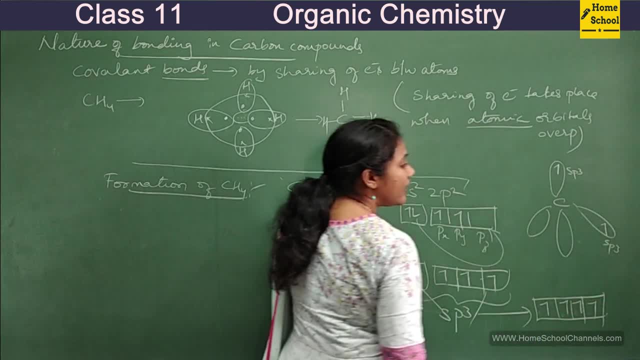 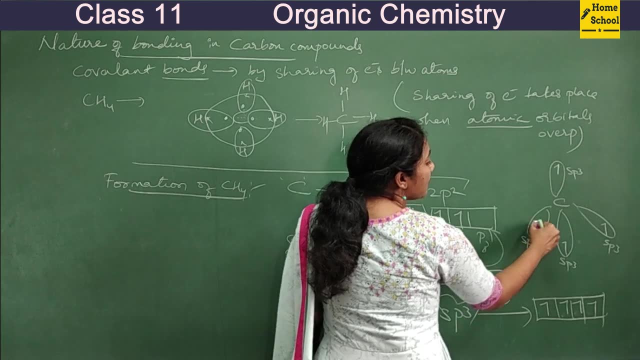 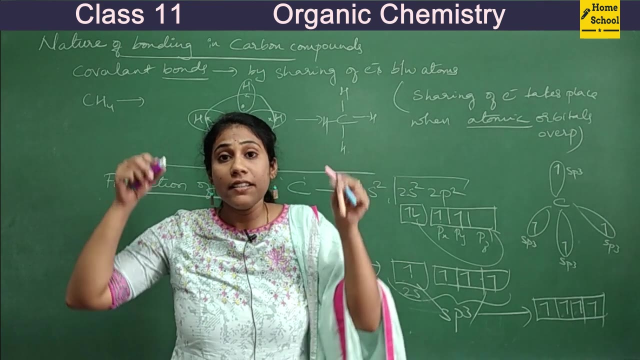 this is another sp3 hybridized orbital with one electron. third sp3 hybridized orbital with one electron. fourth sp3 hybridized orbital. this is another sp3 hybridized orbital with one electron. okay, so orbitals are balloon like structures, so they are directed in certain positions. 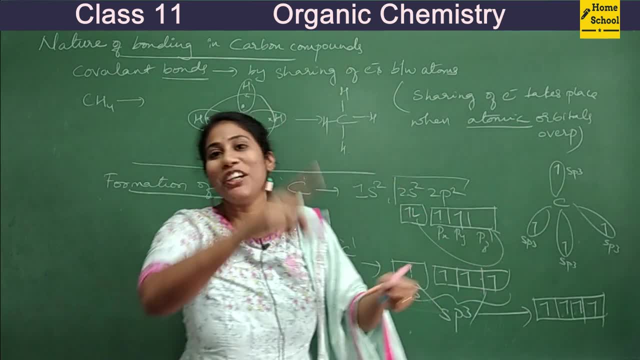 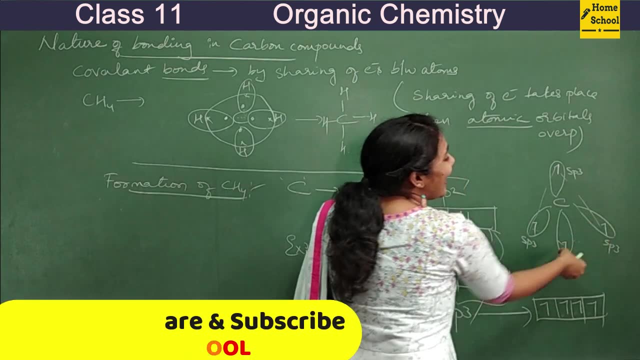 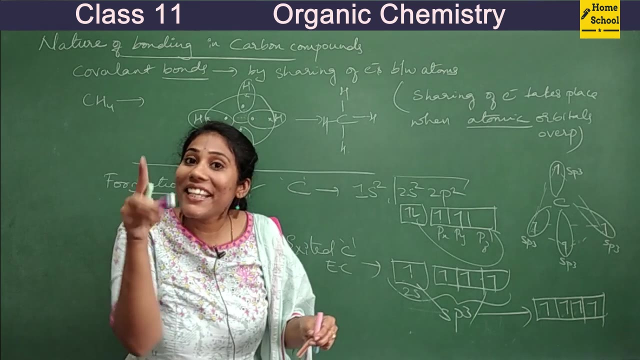 in space. okay, so that is what? giving a shape for organic molecule? okay, say, this is actually. what is this shape? this is a shape of tetrahedron. guys, this is a shape of tetrahedron. you know, these four hybrid orbitals are arranged in the shape of tetrahedron. that is why we say: 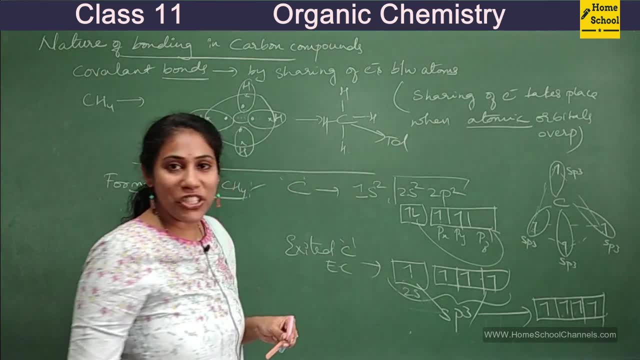 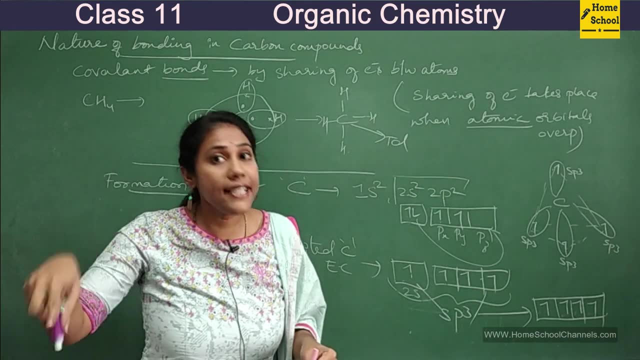 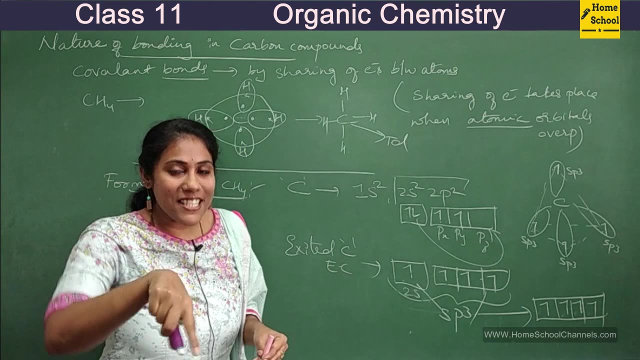 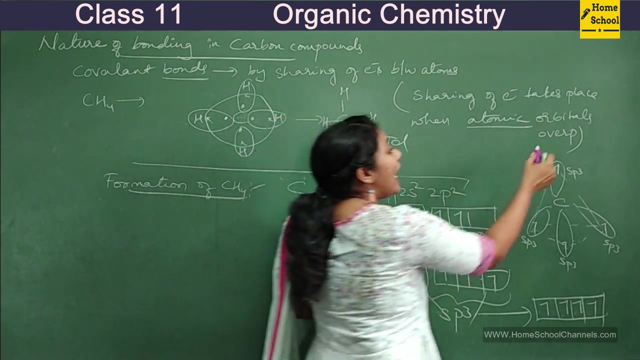 methane molecule has tetrahedral structure. okay, so the arrangement of hybrid orbitals in the space is a reason for a shape of a molecule. okay, so what hybridization? carbon in a methane underwent sp3 hybridization. okay, so now orbitals are ready for overlapping. so now, as hydrogen's orbital. 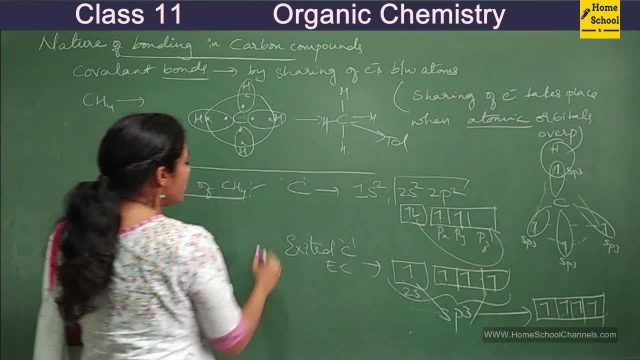 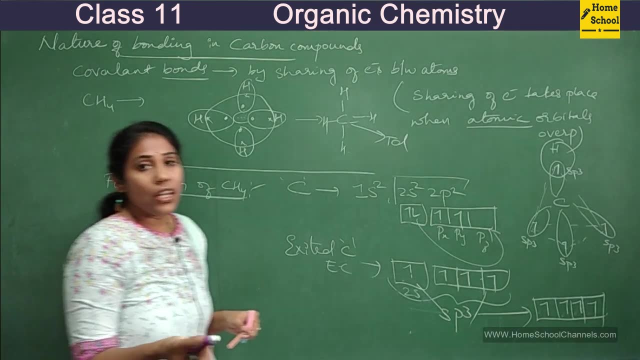 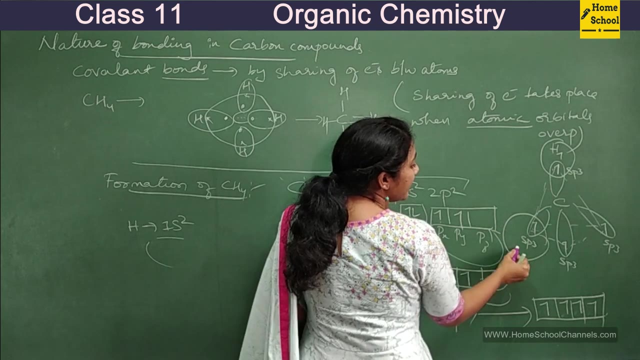 okay, hydrogen hydrogen. what is hydrogen hydrogen is a hydrogen which is a hydrogen, which is a hydrogen's electronic configuration. it is 1s2, right, so hydrogen has s orbital. s orbital is always spherical, so this is one hydrogen orbital carrying one electron. here comes another hydrogen carrying 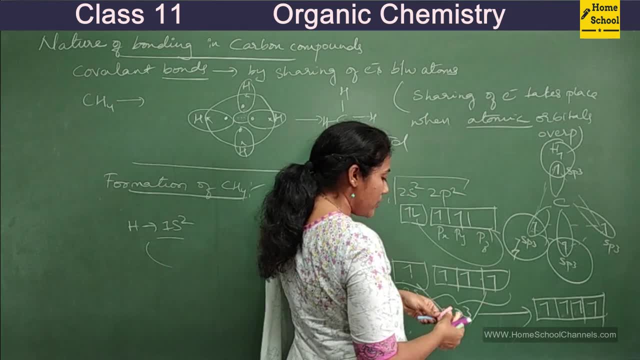 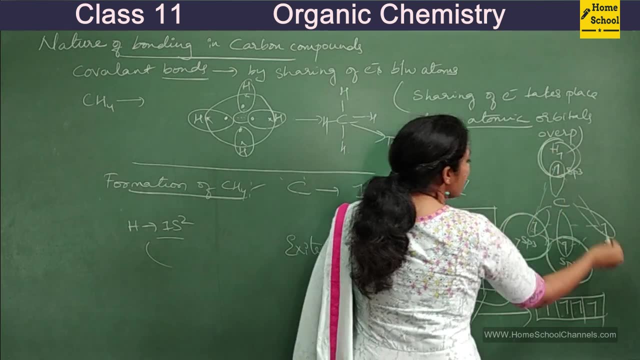 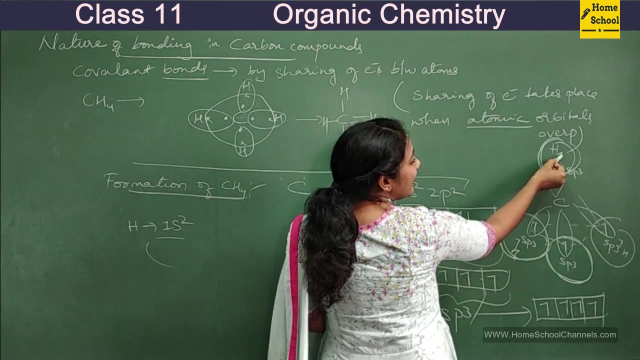 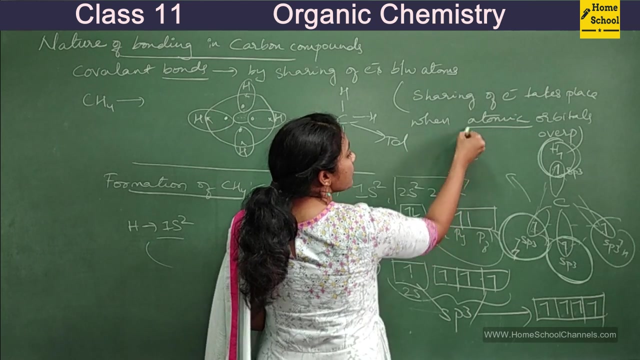 one electron. this is the third hydrogen. okay, let me change the color for a differentiation purpose. so this is the third hydrogen. second hydrogen, first hydrogen. so fourth hydrogen atom carrying one electron. okay, so when hydrogen's orbital carrying one electron overlaps with this sp3 hybrid orbital, then we say a bond is formed. this is one ch bond, another ch bond, third ch bond, fourth ch bond. 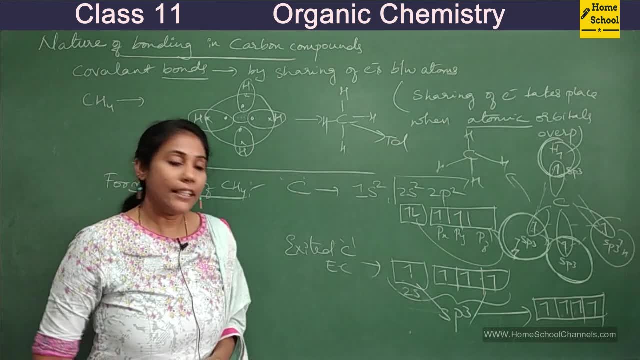 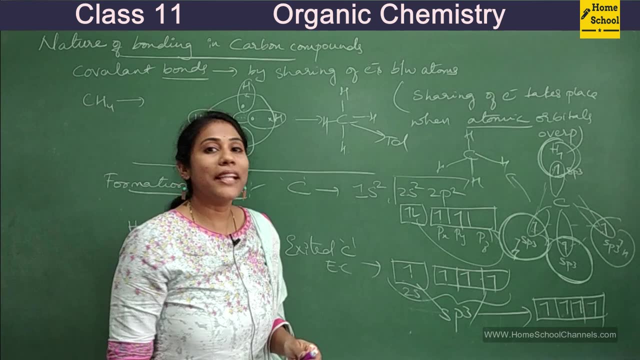 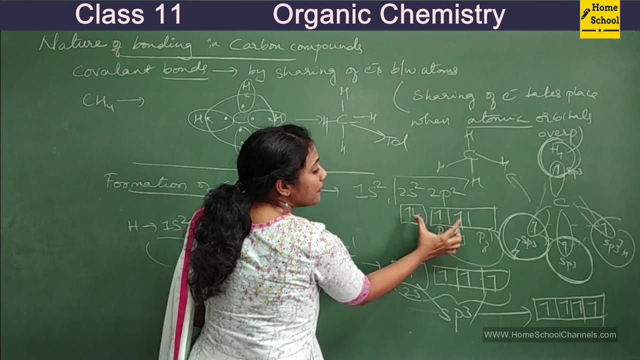 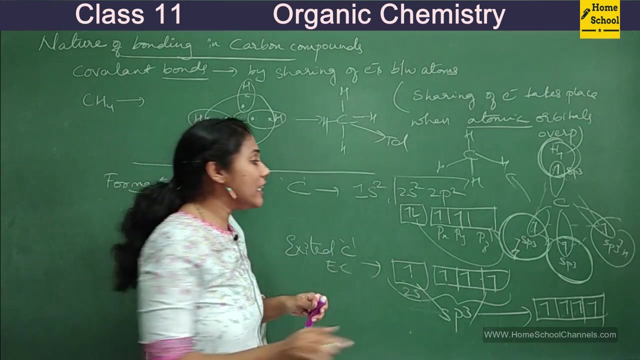 okay, so this is how methane molecule is formed. definitely, sharing of electron took place. window sharing took place when atomic orbitals overlap. okay, so hydrogen's atomic orbital overlap carbon's atomic orbitals, four orbitals to overlap. they should get ready. they must have equal energy. just to make their energies equal, they will undergo a process of mixing orbitals called. 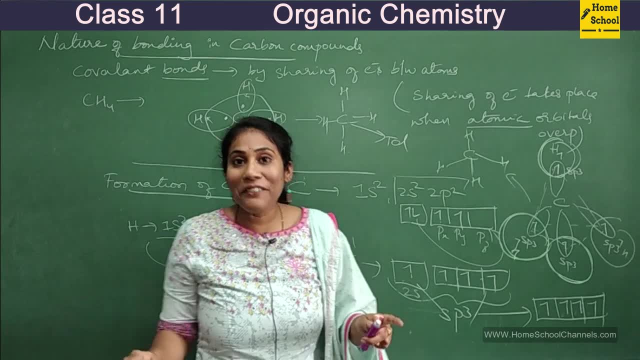 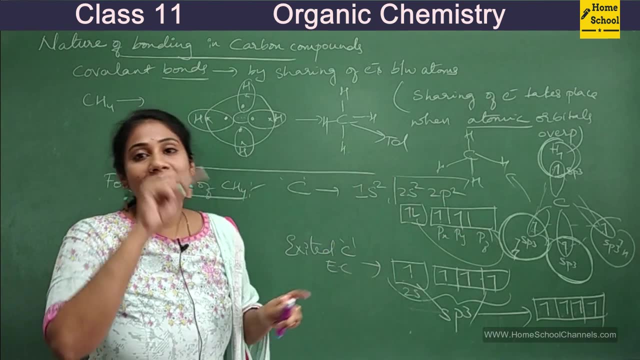 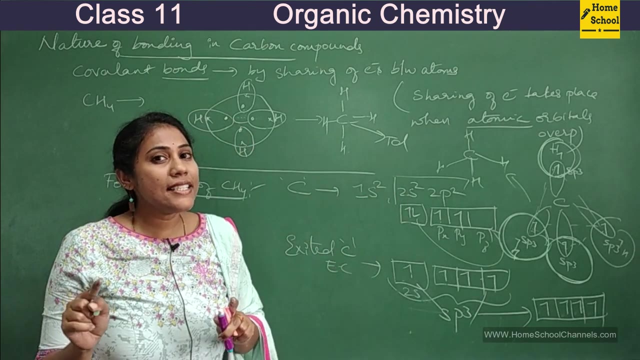 hybridization. okay, so hope you are clear with the concept of hybridization, right? so here the carbon atom is undergoing sp3 hybridization. okay, so this is how methane molecule is formed. now let us understand another type of hybridization, called sp2. carbon can undergo sp3. 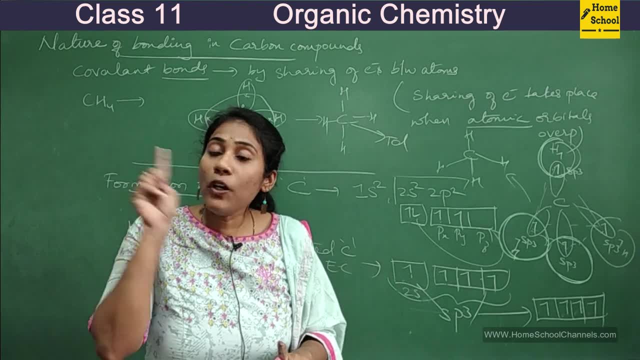 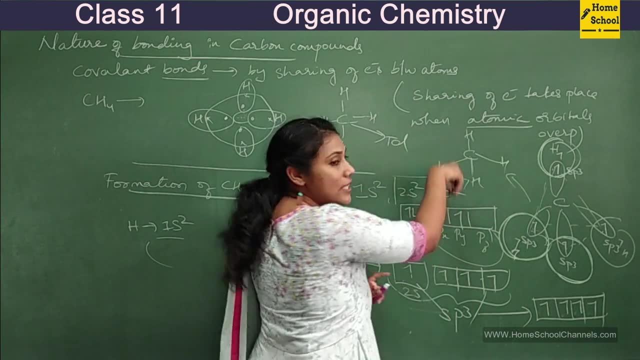 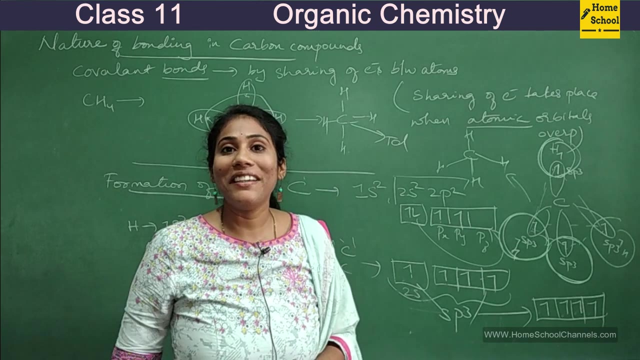 it can undergo sp2. it can also undergo sp3. when it undergoes sp3 hybridization, you know, it will form four single bonds around it. when it undergoes sp2 hybridization, it forms one double bond around it. and when it undergoes sp hybridization, 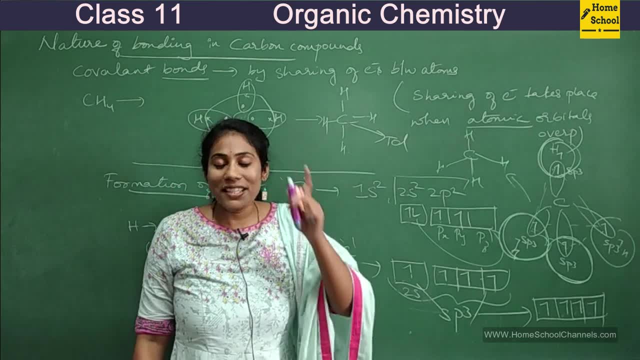 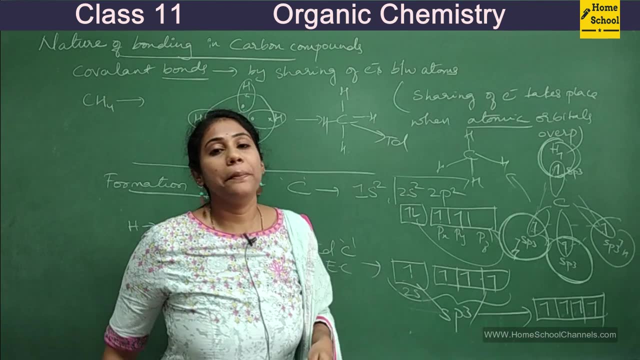 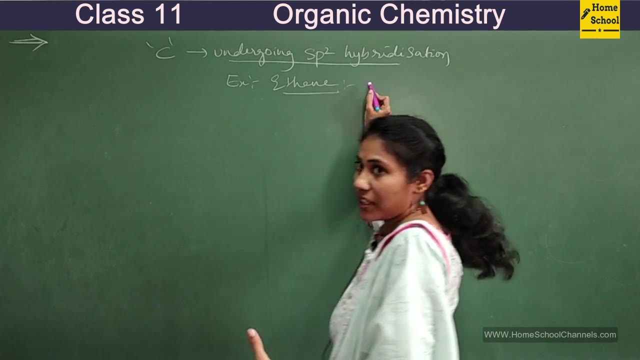 it will form triple bond around it. okay, so this is a very, very important concept. now we will study how carbon can undergo sp2 hybridization. take an example of ethene guys, so you must have studied about ethene structure in your lower classes. how do we write ethene, ch2, double bond, ch2- right? 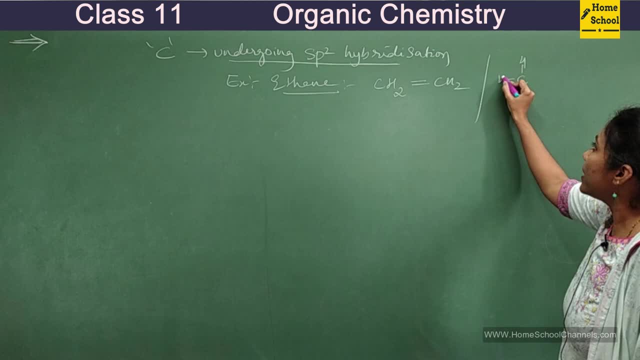 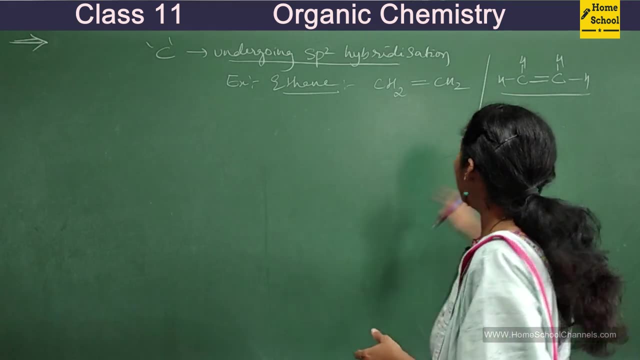 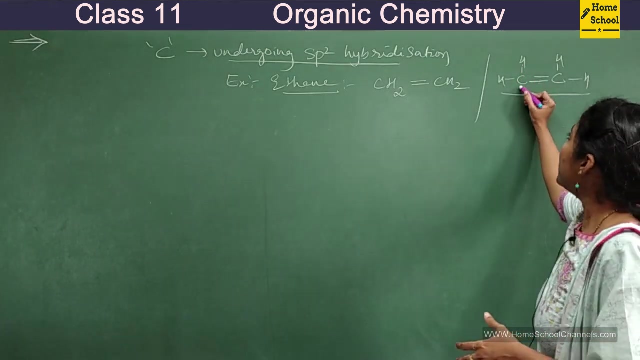 again, if i have to elaborate carbon single bonds with hydrogen double bond with another carbon, right. so this is the elaborate structure of ethene. so now i will tell you how this molecule is formed, how these two single bonds and how this double bond is formed. okay, so this is carbon number one. 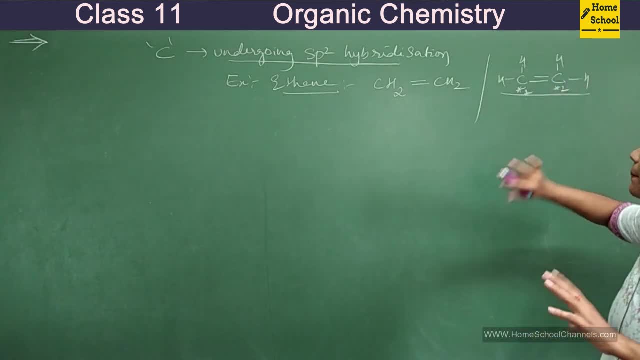 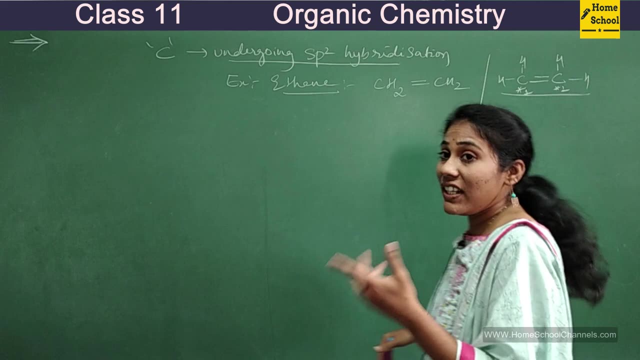 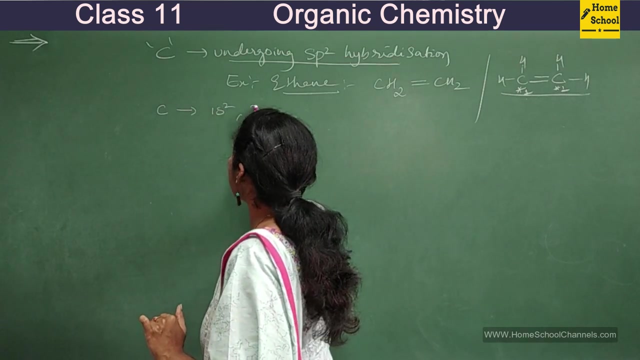 okay, and this is carbon number two. so both of them have to undergo hybridization here. but they will not undergo sp3 hybridization here. okay, they will undergo sp2 hybridization. see, we all know carbon's sp2 hybridization. one s, two, two s, two, two p, two right. so orbital diagram s orbital is only one. 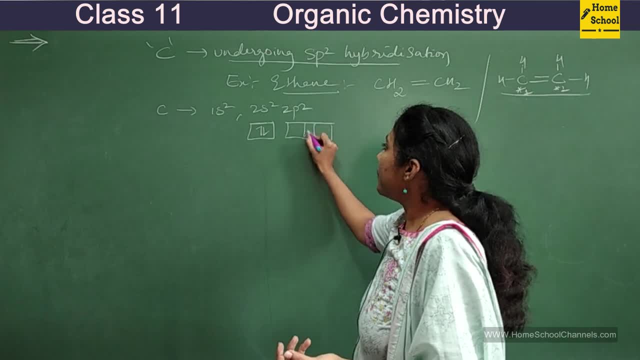 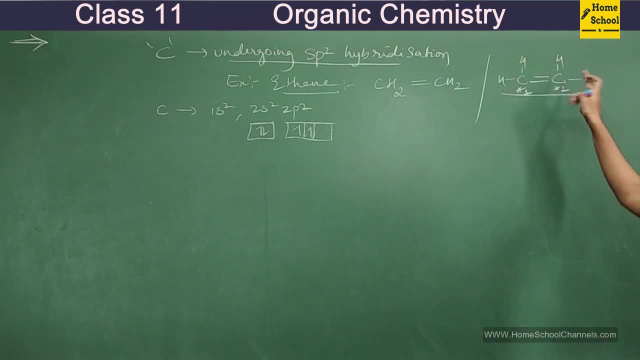 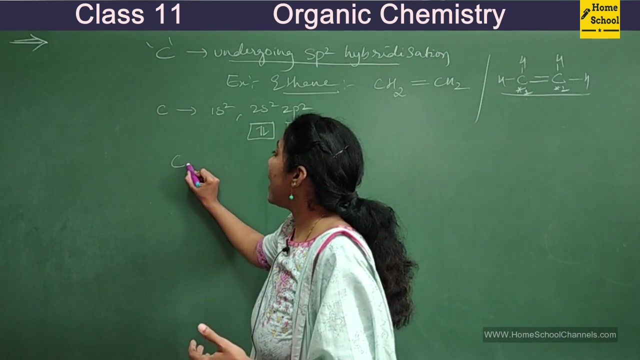 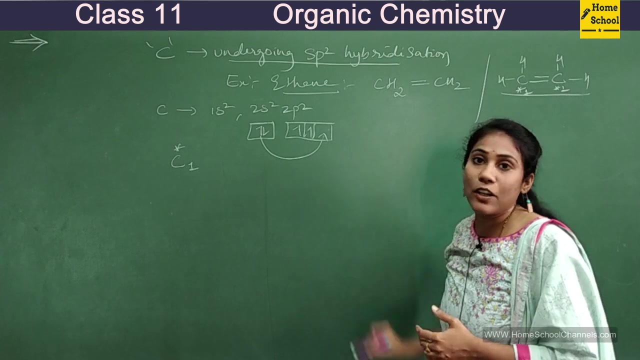 in that two electrons are there, p orbitals are three, you have two electrons each. okay, so now, as these two hydrogens and this carbon approaches towards carbon, approaches towards carbon, carbon gets excited, carbon number one gets excited and one of the electron will move to empty pz orbital. so now, excited state. electronic configuration of carbon one is: 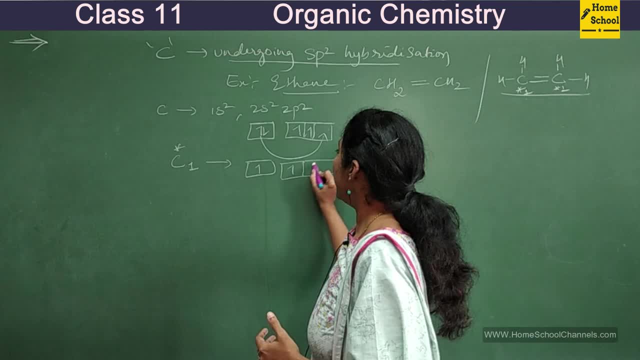 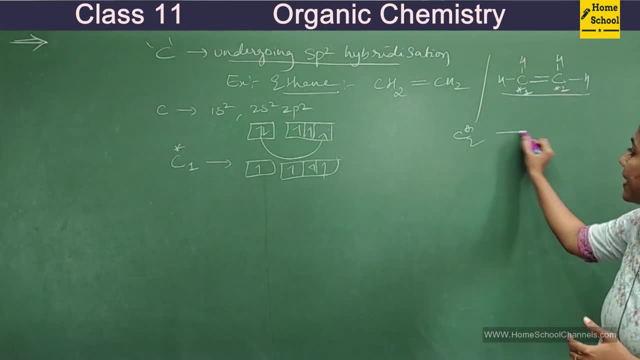 you know, like this right, say one, one, one right. and second carbon. second carbon also gets excited and its excited state electronic configuration is this: okay, so each right, so both carbons gets excited as hydrogens approaches. so this is very excited state electronic configuration okay. and but here you know, 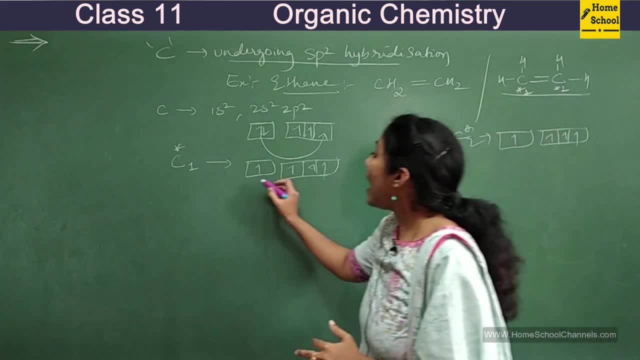 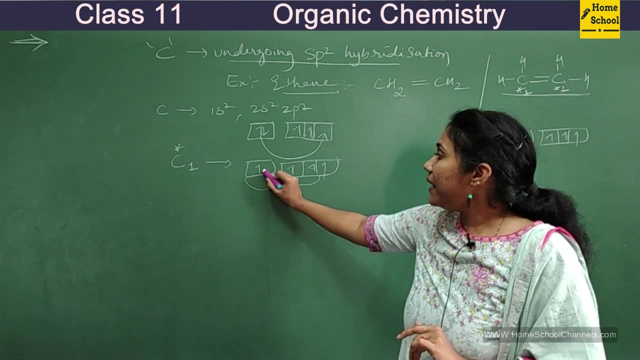 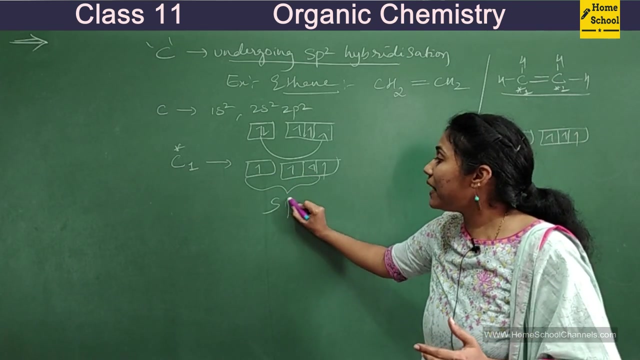 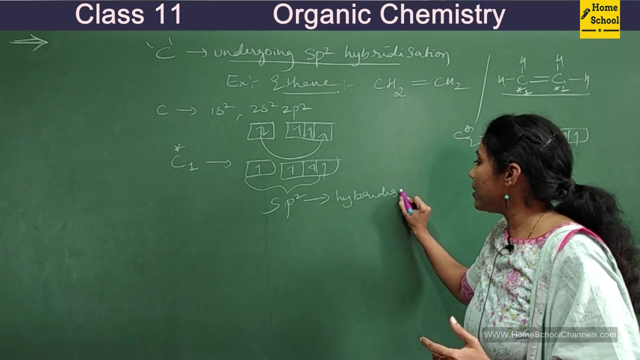 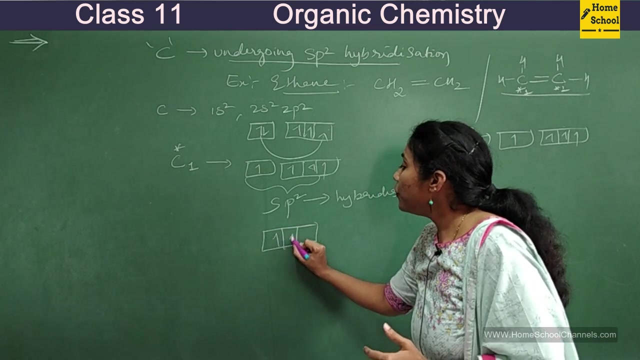 when these hydrogens approaches, carbon will undergo only sp2 hybridization, only this orbital. this orbital and this orbital's overlap. so how many s orbitals one, how many p orbitals two? so here the carbon is undergoing sp2 hybridization, hybridization, sp2 hybridization. okay. so how many new hybrid orbitals you will get? you will get only. 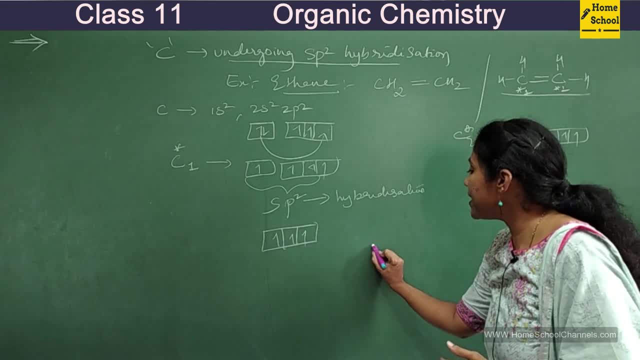 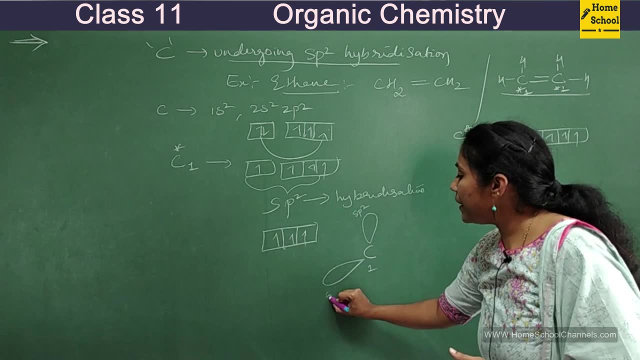 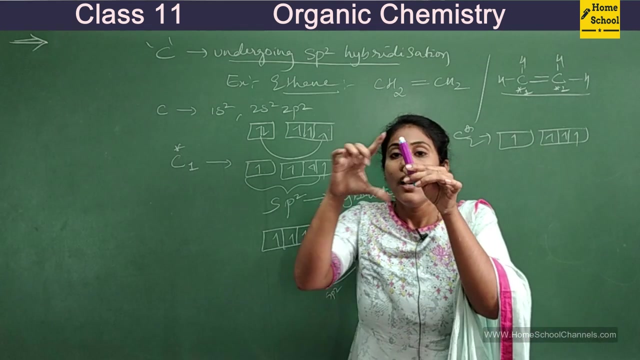 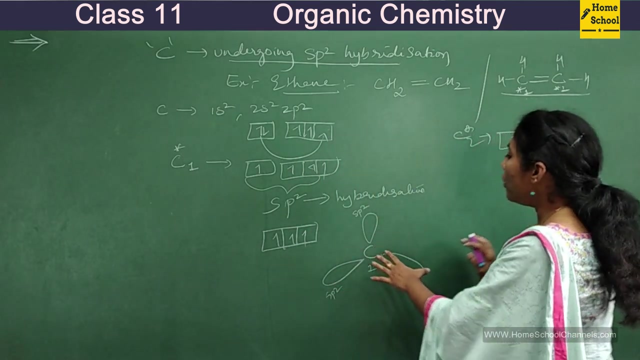 three. so how, how they are arranged. say, if this is c1 carbon, so this is one sp2 hybrid orbital, this is another sp2 hybrid orbital, this is the third sp2 hybrid orbital. okay, so when there are three things, how they will get arranged as far as possible in a triangular way. okay, fine, so our 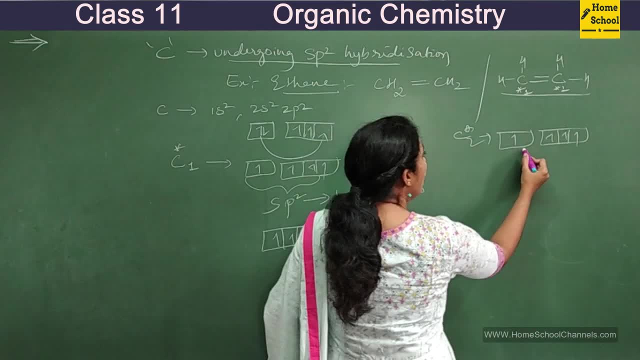 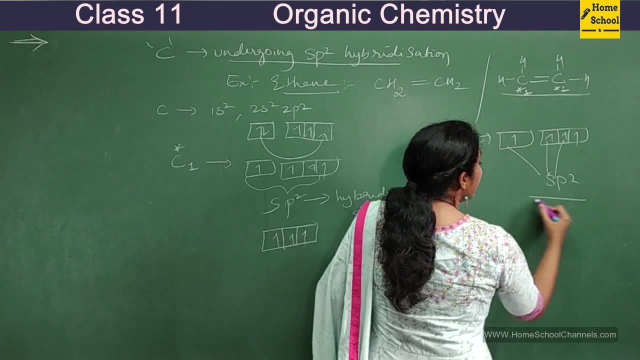 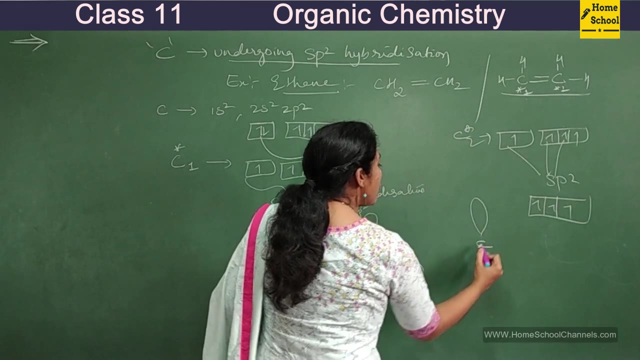 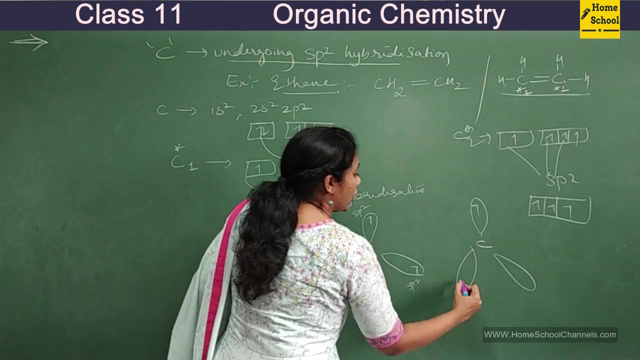 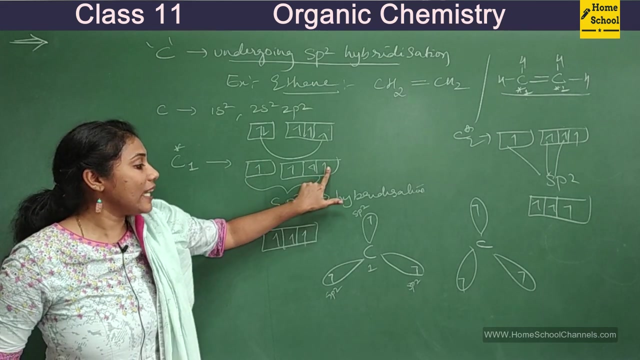 carbon. number two also, will undergo sp2 hybridization. only it will also undergo sp2 hybridization. and three new sp2 hybrid orbitals, it will get okay. so here also. these orbitals are arranged in a triangular way itself, so each orbital has one, one electron. this is how okay. and now remember, oh, the unhybridized orbital. 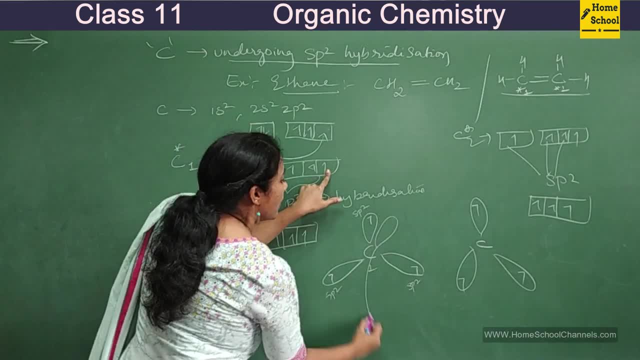 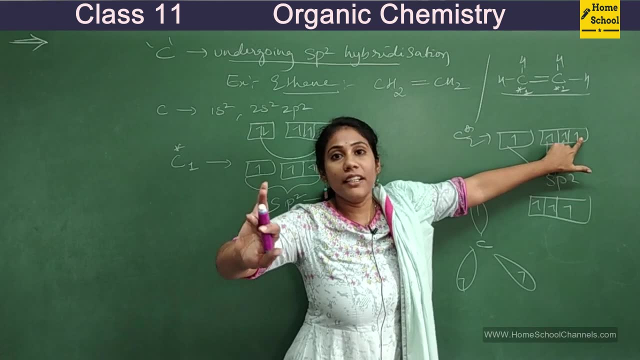 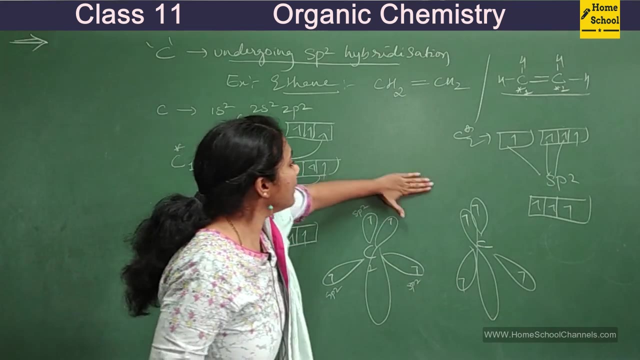 is as it is right. so this is unhybridized orbital. i will mention like this: this also has electron. even in this carbon there is one orbital which did not undergo hybridization. that is there as it is, with one electron. okay, fine, so now what will happen? you know two hydrolysis. 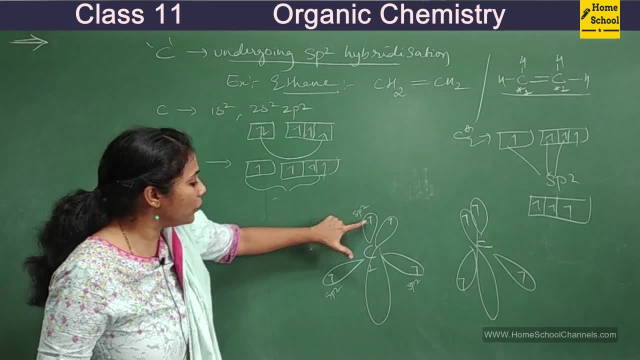 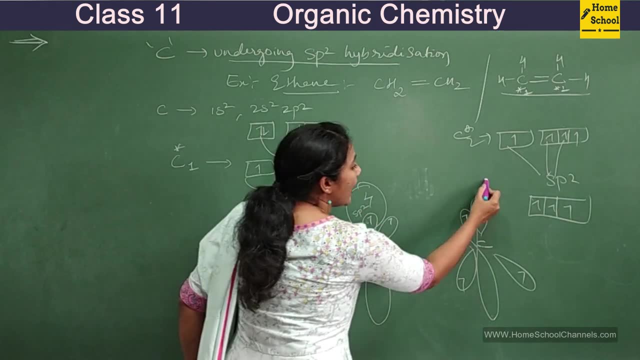 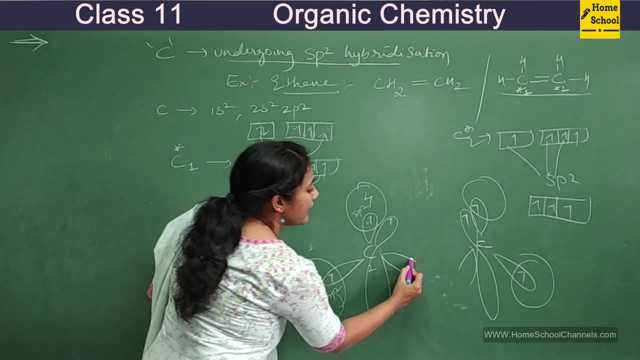 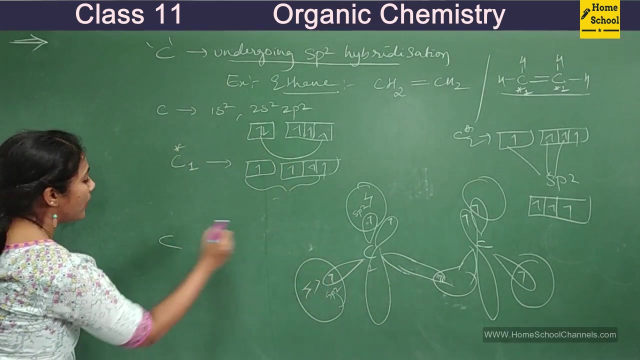 will come to. two hydrogens will come to these carbons, so they will overlap. okay, so here another hydrogen: overlap, two hydrogens will come to this carbon, they will overlap, and this orbital, you know this orbital- gets overlapped with this orbital. okay, is that clear. so now let me write the bond. 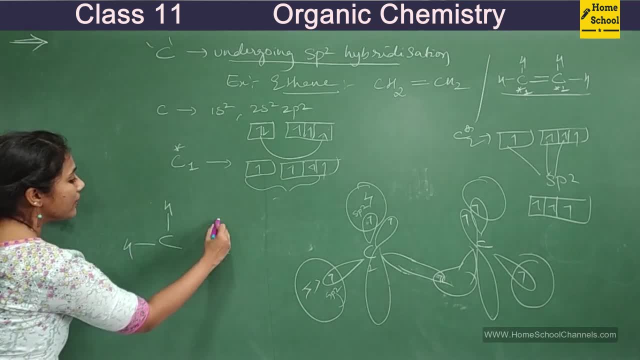 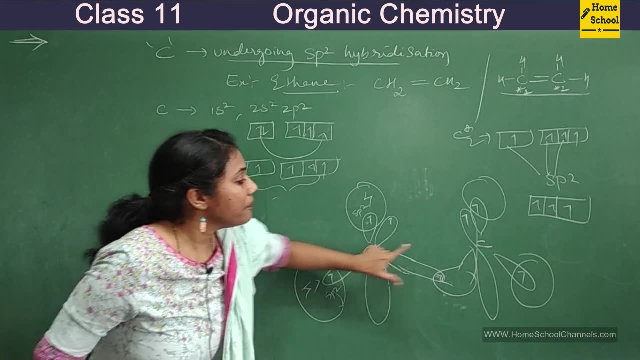 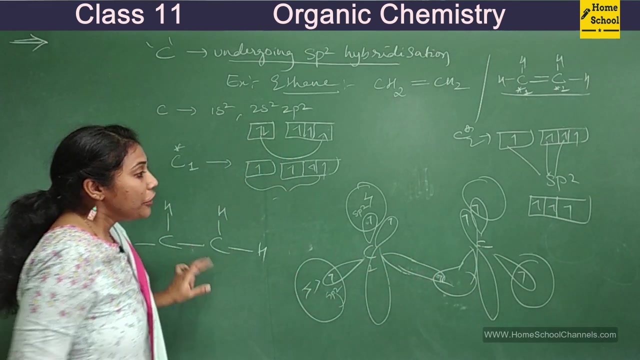 there is one bond with hydrogen, another bond with hydrogen, this carbon also. one bond with hydrogen, another bond, and there is a bond: one of the hybrid orbital of this carbon and one of the hybrid orbital of this carbon also overlapped, so there is a bond. okay, now you know, unhybridized. 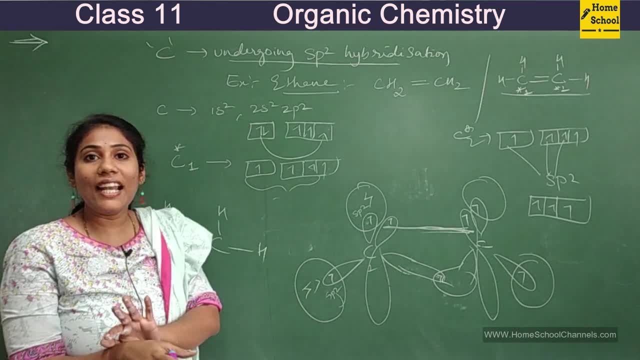 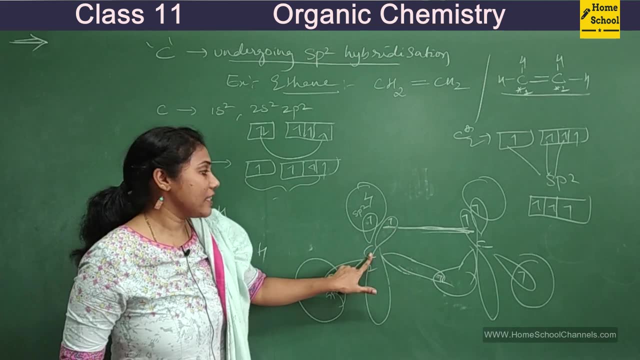 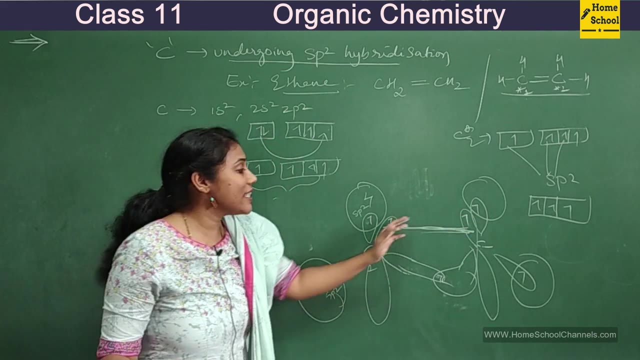 orbitals are there. no, they will also get overlapped, but this overlapping is very, very weak. this unhybridized orbital of this carbon, this unhybridized orbital of this carbon, also overlapped because they also contain electrons they can share right. so that's how you will get a double bond. 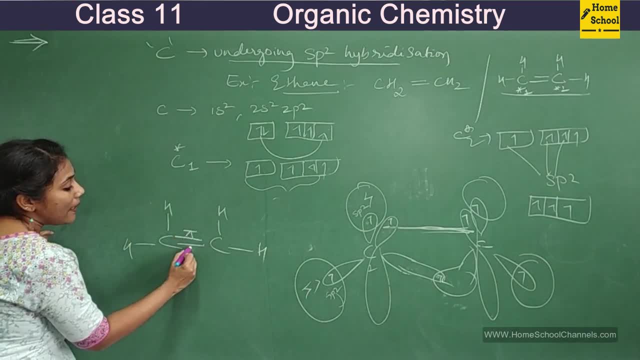 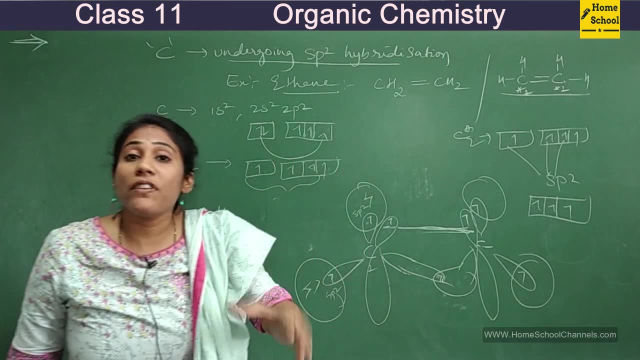 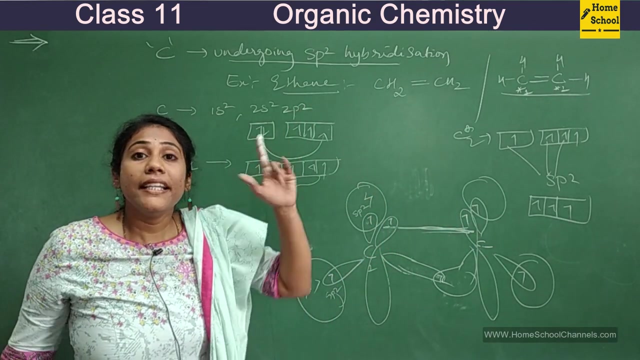 actually this bond we will call it as pi and this bond we will call it as sigma. okay, when hybrid orbitals overlap, it leads to a stronger bonding called sigma bond. when unhybridized orbitals overlap, it leads to a weak bond, weak covalent bond, called pi bond. so that is why we 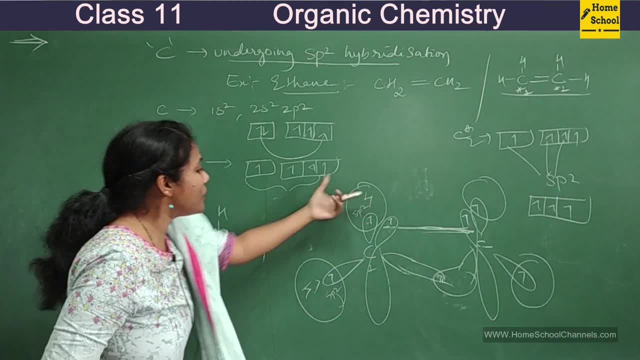 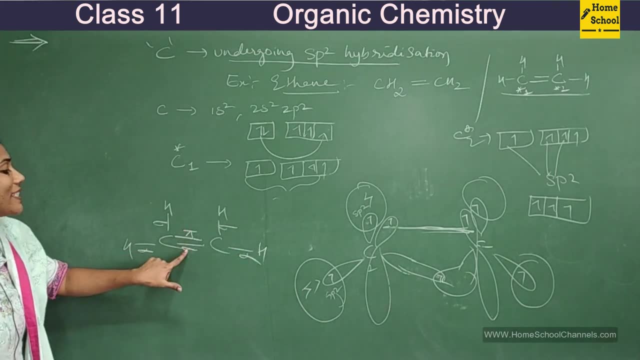 say: you know, this is also sigma bond, because hybrid orbitals only are overlapping right, this is also sigma bond. this is also sigma bond. this is also sigma bond. so, one pi bond is there, one sigma bond is there. so here, what is the hybridization of every carbon? this underwent sp2. 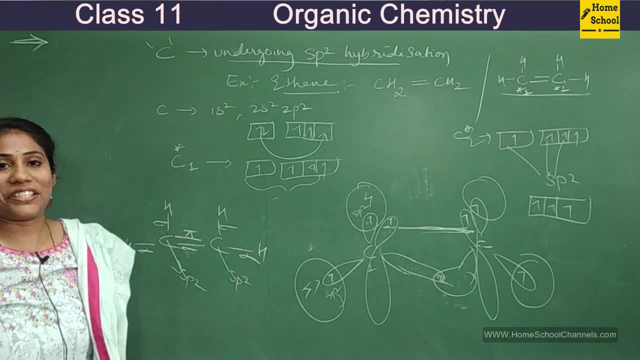 this also underwent sp2 hybridization. okay, so this is how sp2 hybridization is formed with carbon atoms. okay, so this is how sp2 hybridization is formed with carbon atoms. right? so similarly, if i take an example of ethane: right, so similarly, if i take an example of ethane. 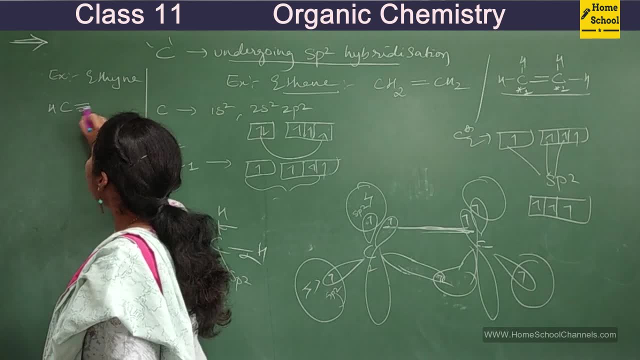 right. so similarly, if i take an example of ethane: okay, ethine. how do you write the structure ch? okay, ethine. how do you write the structure ch? okay, ethine. how do you write the structure ch? triple bond ch. so here actually the carbon. triple bond ch, so here actually the carbon. 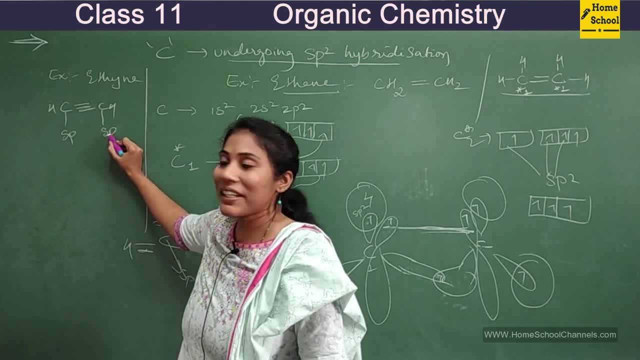 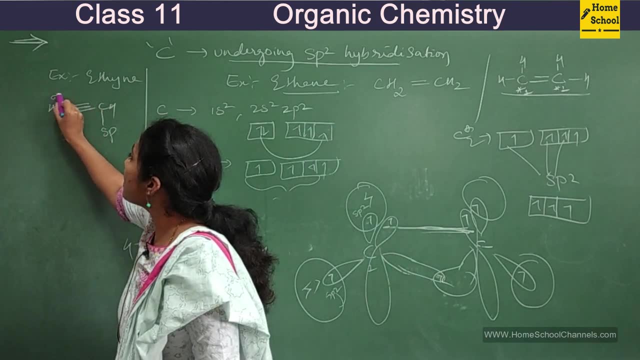 triple bond ch. so here actually the carbon must have undergone sp hybridization. okay, say must have undergone sp hybridization. okay, say must have undergone sp hybridization. okay say, uh sp hybridization, every carbon, uh sp hybridization, every carbon, uh sp hybridization, every carbon underwent. so here this bond is sigma. 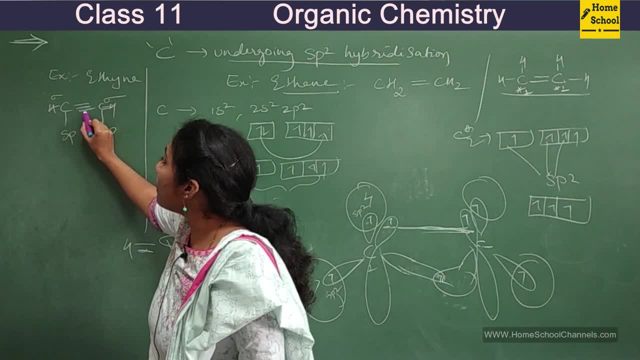 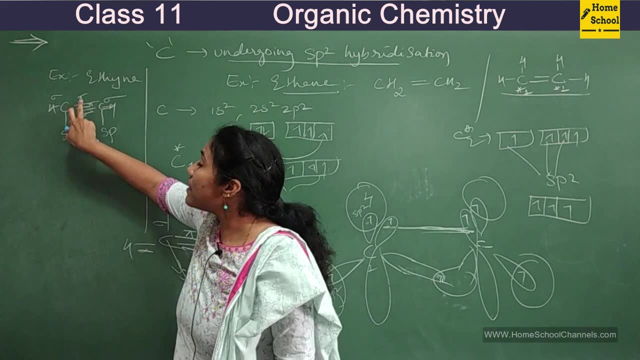 underwent. so here this bond is sigma underwent. so here this bond is sigma. this ch bond is sigma among the triple bond. this ch bond is sigma among the triple bond. you know, one bond is sigma, two bonds are pi. that means these two bonds are formed by overlapping of. 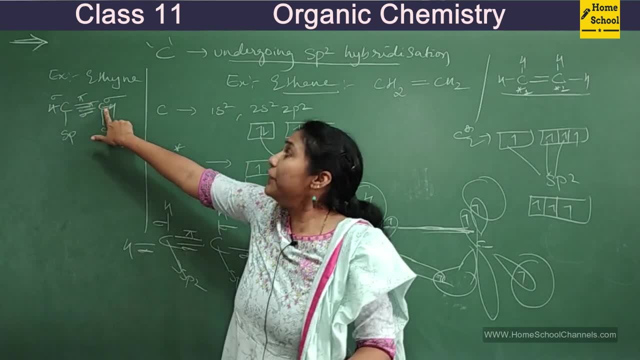 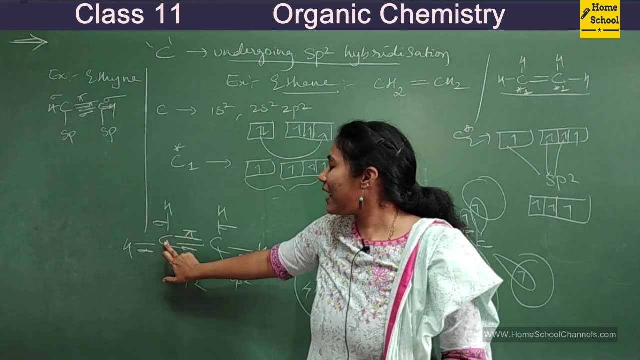 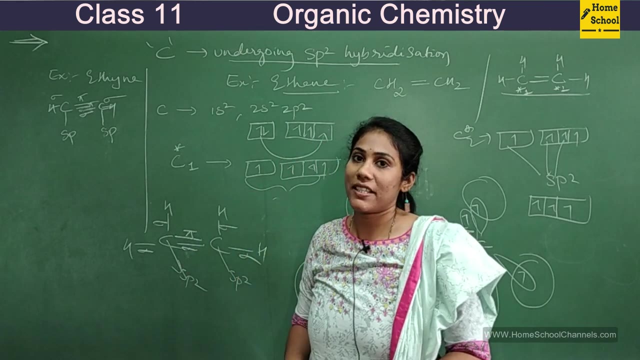 two unhybridized orbitals of this carbon and two unhybridized orbitals of this carbon. okay, so like this: if you have a double bond with a carbon, it is- uh, you know, noted that that carbon must have underwent sp2 hybridization. if you have triple bond with carbon, it should be. 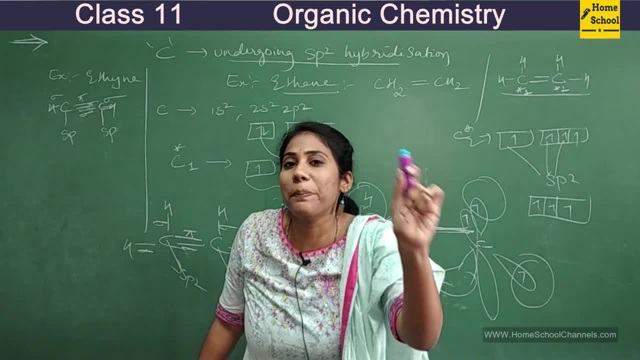 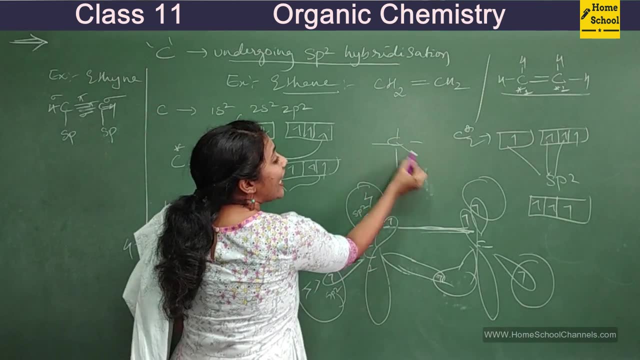 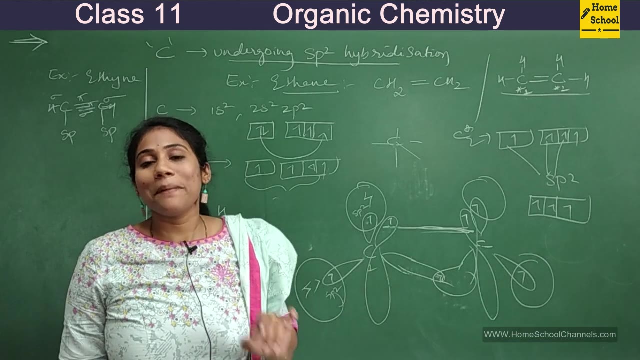 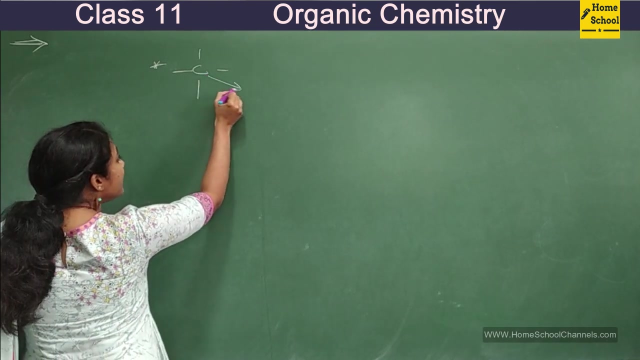 noted that those carbons must have undergone sp hybridization. okay, if a carbon has all single bonds only around it, then that carbon must have undergone sp hybridize, sp3 hybridization. so this concept is really very, very important. you guys, if a carbon has all single bonds around it, then that carbon has what hybridization? sp3 hybridization. 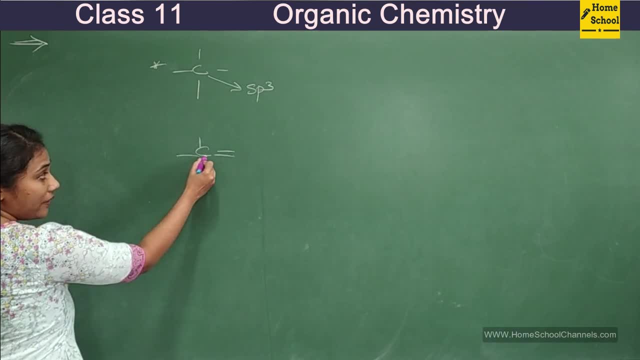 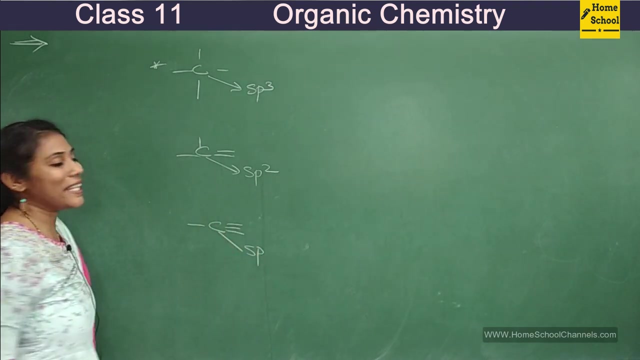 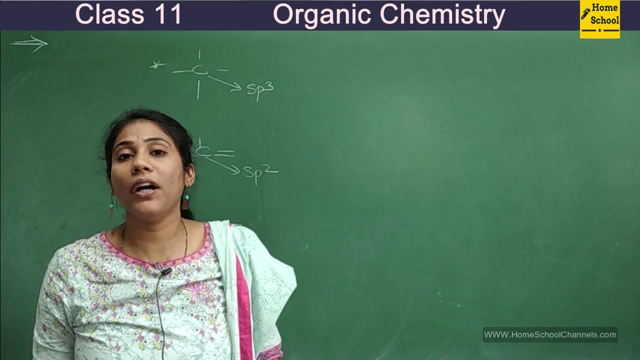 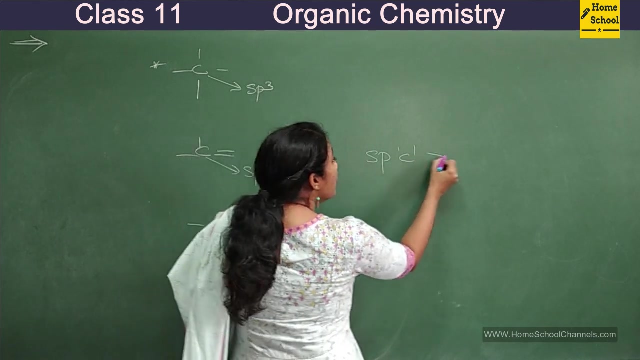 okay, if a carbon has a double bond associated with it, then that particular carbon must have undergone sp2 hybridization. okay, if a carbon has a triple bond with it, then that carbon must have undergone sp hybridization. okay, so identification of carbon atoms hybridization is very, very important, guys. why? because you know what sp hybridized carbon is more reactive than 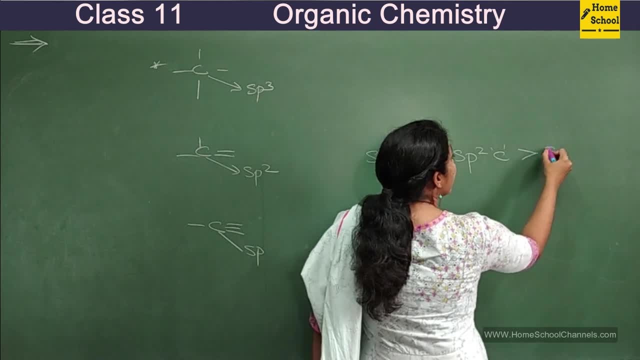 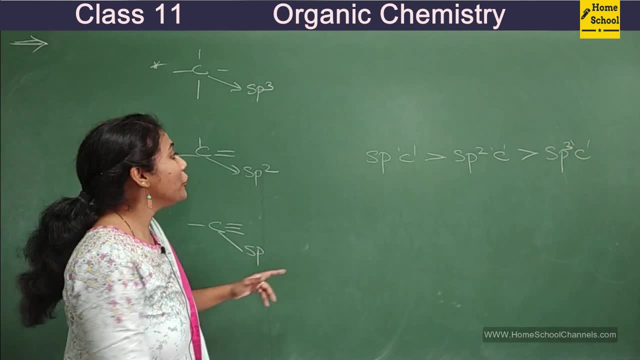 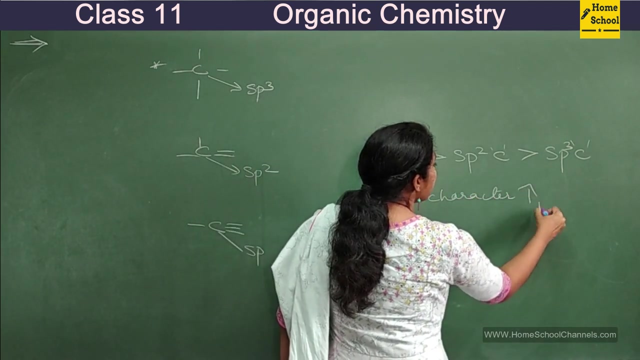 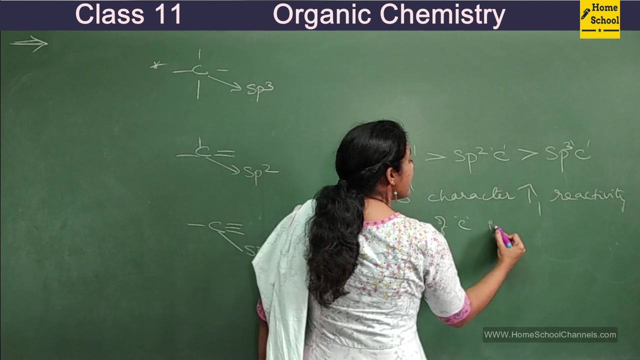 sp2 hybridized carbon. this is more reactive than sp hybridized car, sp3 hybridized carbon, clear. so you know what? as s character increases, as s character increases reactivity, reactivity of carbon increases. okay, clear. say, for example, among the three carbons, which is more? 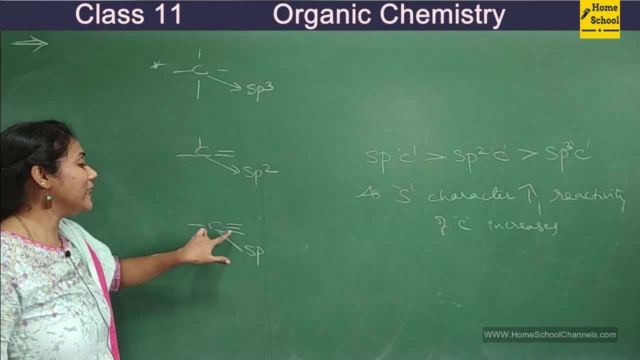 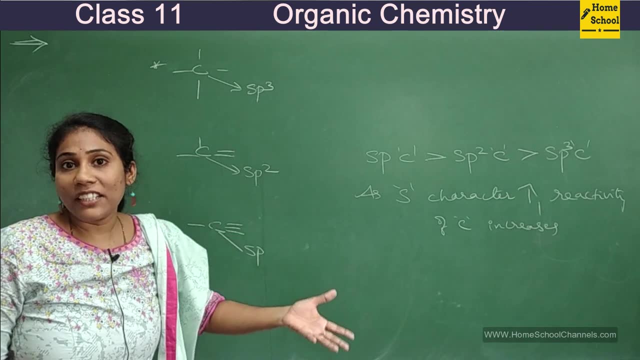 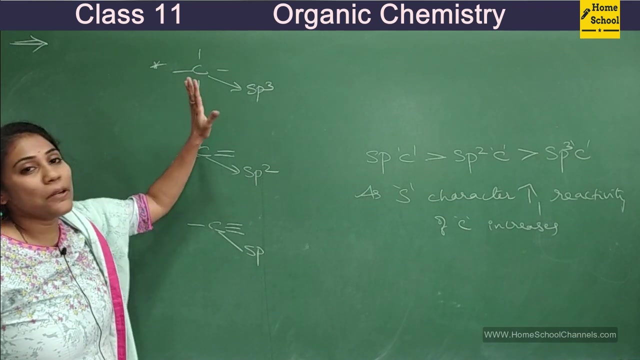 reactive. this particular carbon is more reactive if a carbon has triple bond, then that is a more reactive. okay, so a triple bonded carbon will show more reactions- varieties of reactions compared to double bonded carbon. okay, single bonded carbon if a carbon has all single bonds around it. actually, 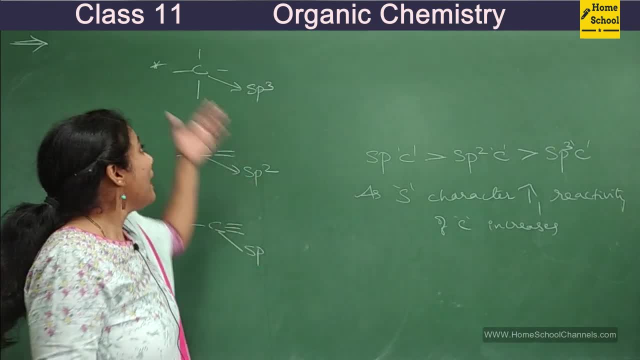 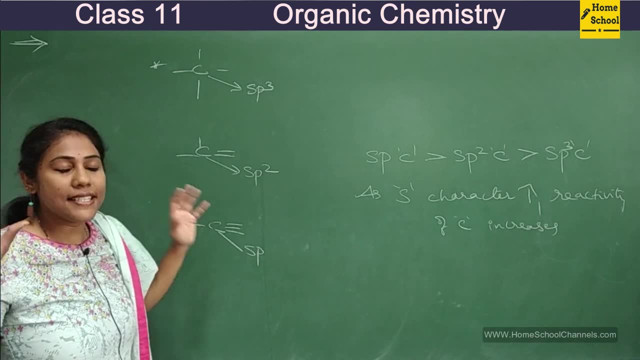 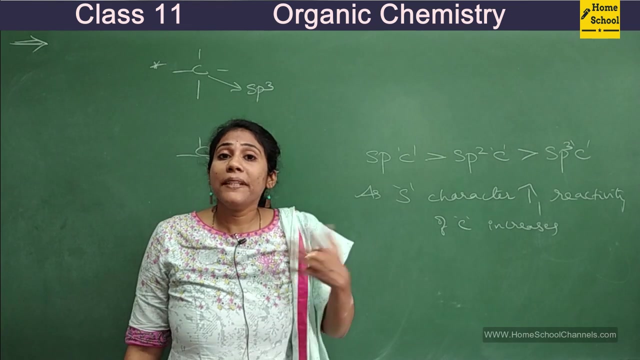 the least reactive. okay, so it is a very, very passive, inactive type, inert type of carbon atom. okay, so hybridization has this much importance in organic compounds, so it is very much essential to understand that which carbon has what hybridization. okay, so now let us deal with some. 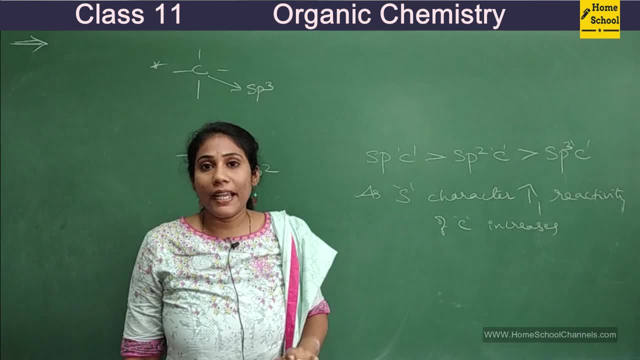 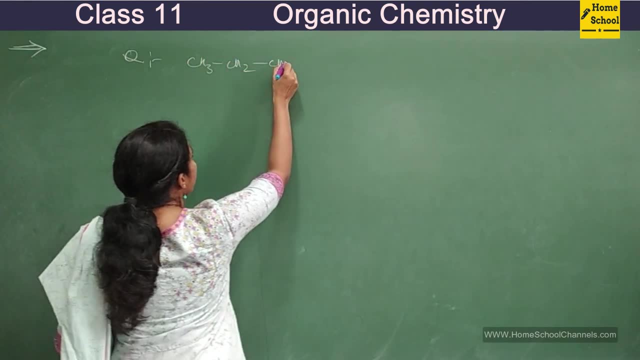 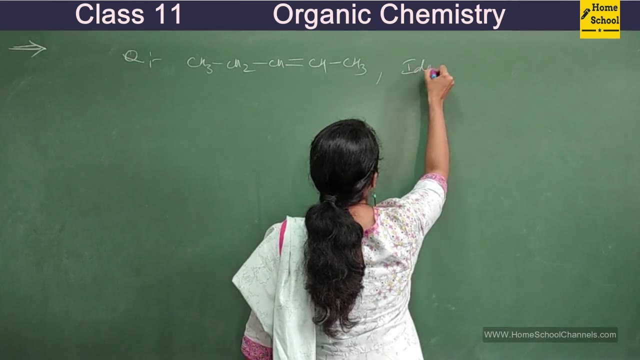 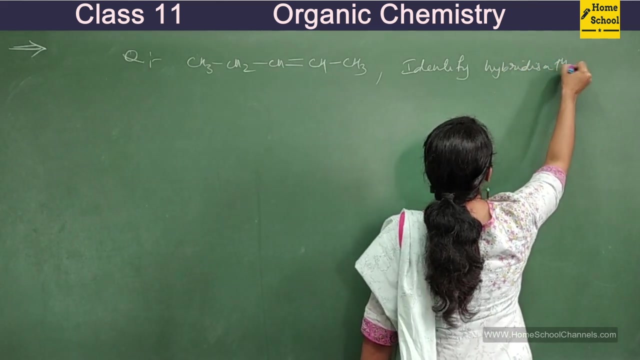 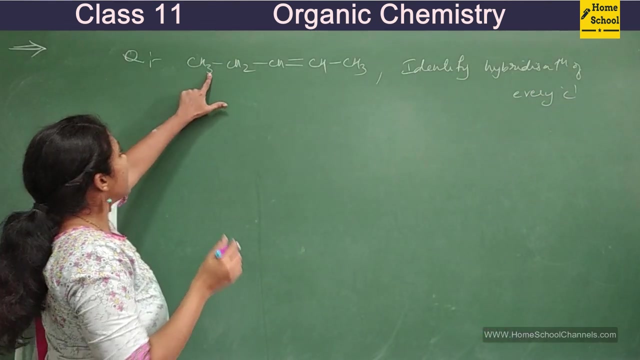 questions relating to this hybridization of carbon atoms topic. see, guys observe the question here: ch3, ch2, ch, double bond, ch, ch3. okay so identify, identify, hybridization, hybridization of every carbon, of every carbon in a molecule. okay, so ch3 means what you know: three hydrogens are arranged. 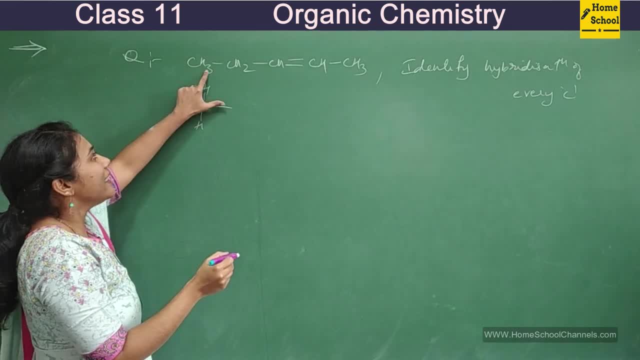 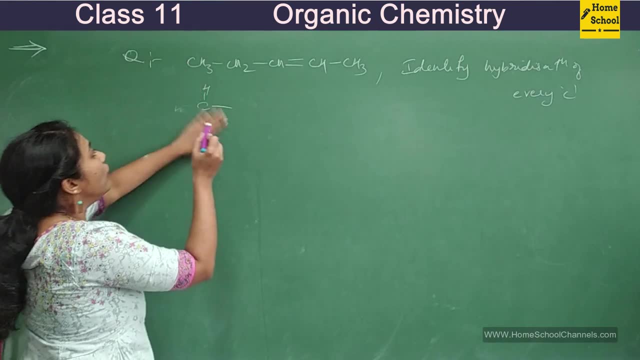 around it. something like this. which example? okay, so we have ch3 and ch2, we have ch2, and so now let's single bonds only, right, so with hydrogens, always single bonds you will find between carbon and hydrogen. okay so, all single bonds around this carbon. right, so this carbon has sp3 hybridization. 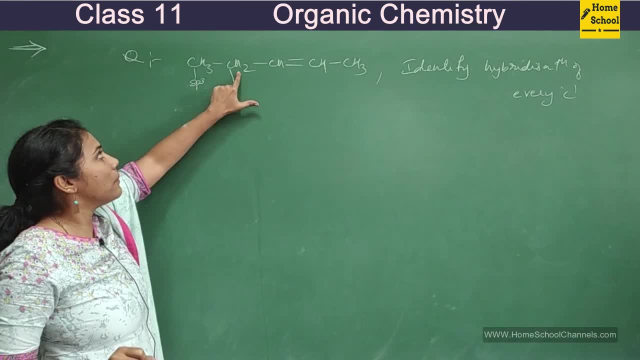 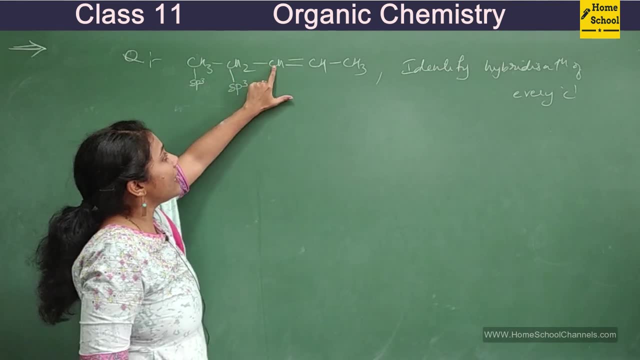 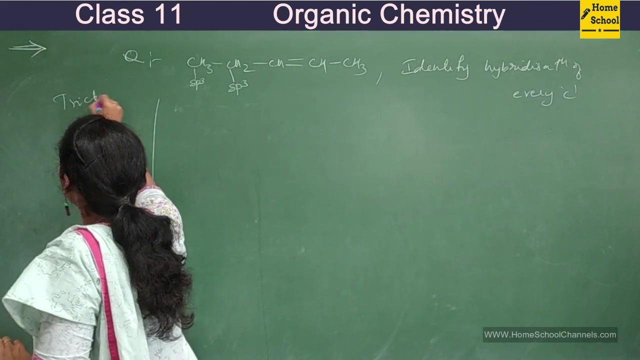 this carbon? two hydrogens means two single bonds, and this is one bond, this is another bond. so even this carbon has sp3 hybridization. what about this carbon double bond? is there? what did i tell you? always? remember a trick here, guys, very, very important: if a carbon has all, 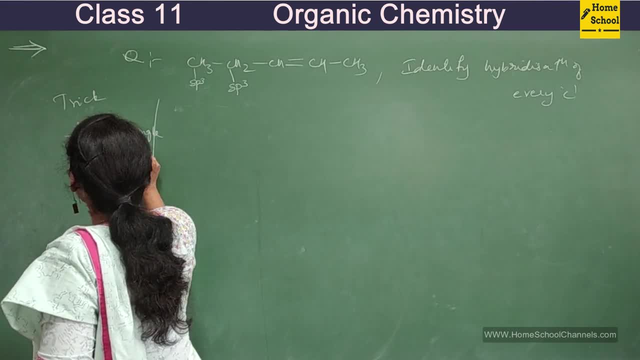 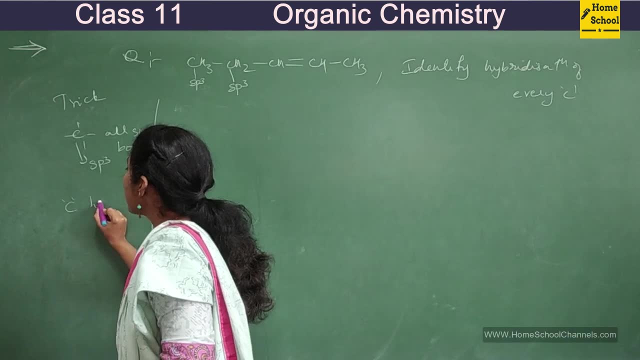 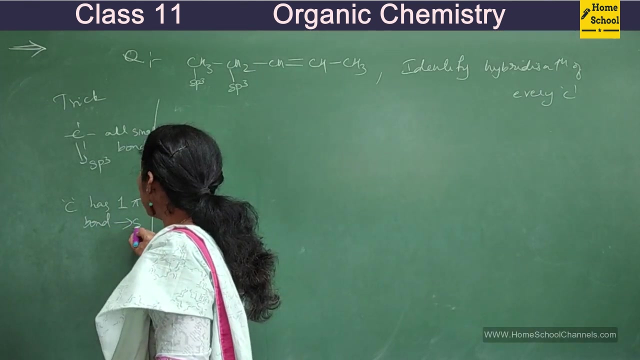 single bonds around it, then that carbon is sp3 hybridized carbon. so if a carbon has at least one pi bond, if a carbon has one pi bond with it, then that carbon has sp2 hybridization. if a carbon has one pi bond with it, then that carbon has sp2 hybridization. 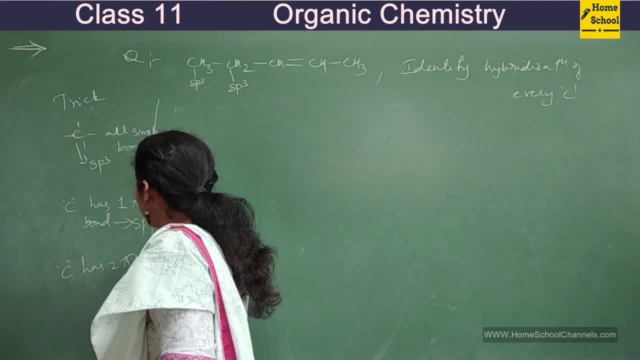 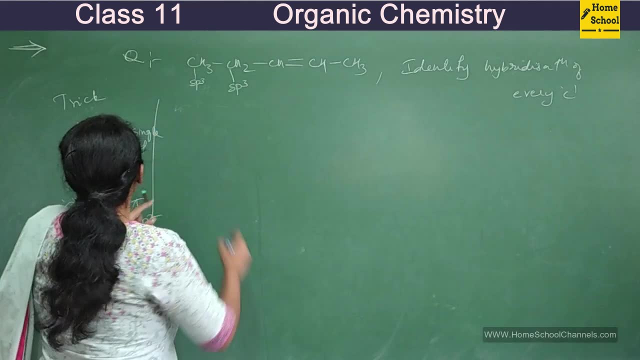 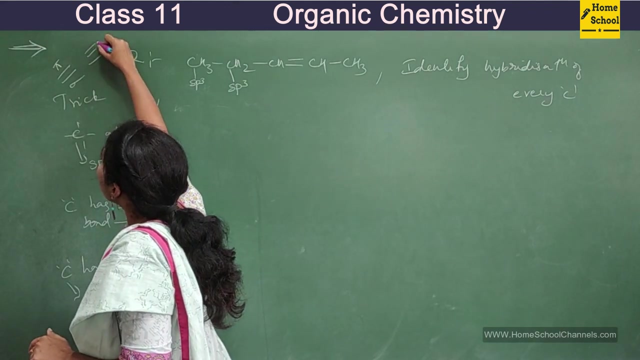 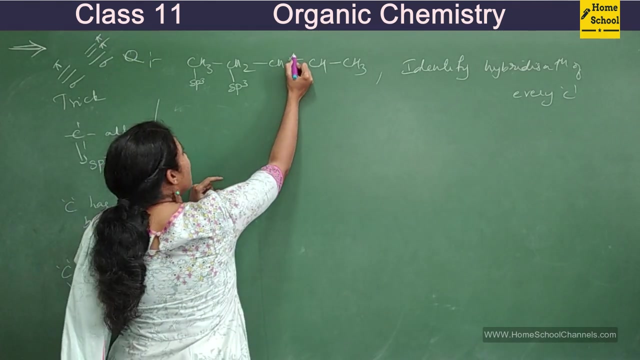 if a carbon has two pi bonds around it, then that carbon is sp hybridization. see, here is a double bond among a double bond. among a double bond. one bond is pi, one bond is sigma among a triple bond. you know, one bond is sigma, two bonds are pi. okay, so this is a double bond. so here, one pi bond is: 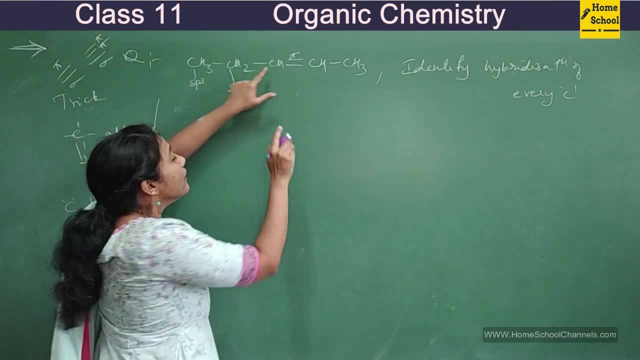 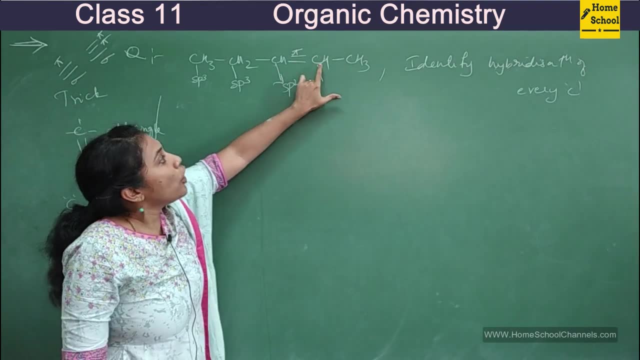 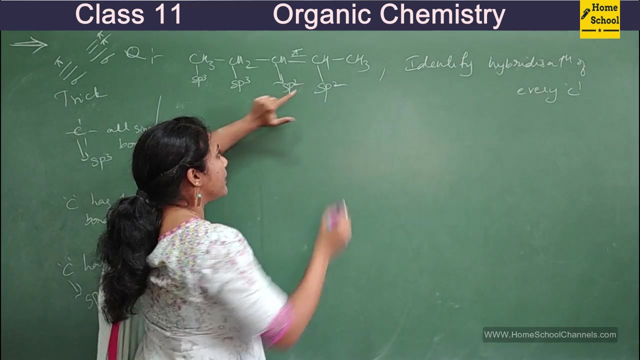 there. so this carbon has one pi bond around it, or whenever a carbon has one pi bond around it as a double bond, then definitely that carbon is sp2. this double bond also belongs to this carbon. so it's like this carbon also have double bond, so even its hybridization is sp2, whereas this 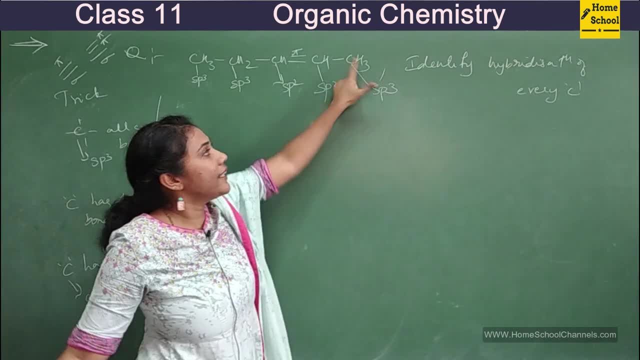 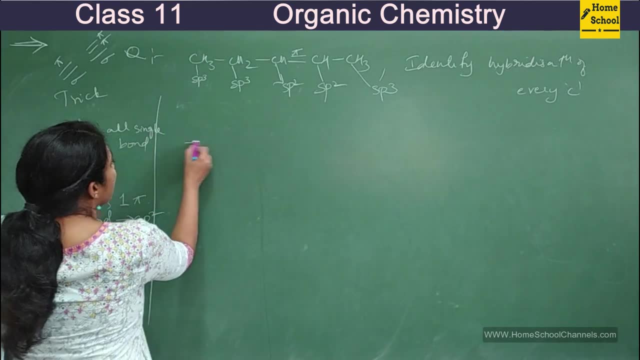 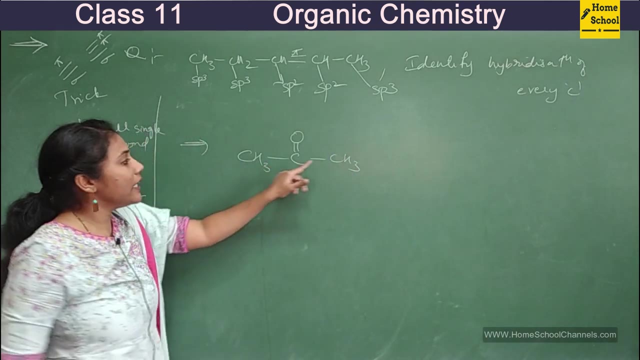 carbon's hybridization is sp3, because all single bonds only around this. three hydrogens means three single bond and this is a fourth bond, so sp3, right. so one more example. one more example. try to observe: ch3, c, double bond, o, ch3. So what is the hybridization of every compound? 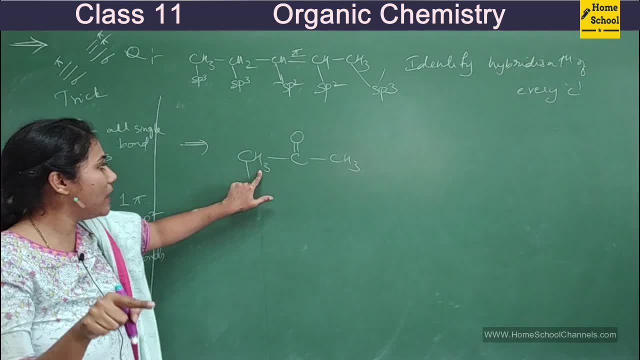 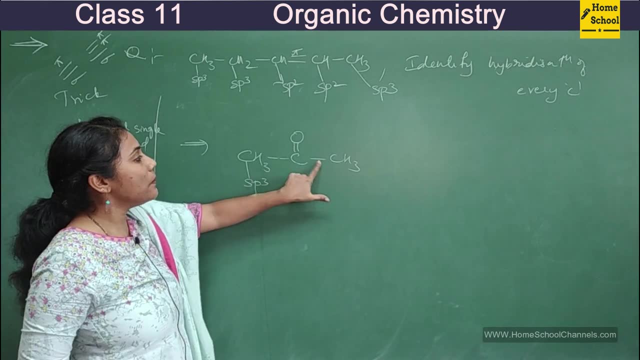 This carbon, all single bonds. 3 hydrogens means 3 single bonds, plus this is 1 bond, 4th bond, So this carbon hybridization, sp3.. What about this carbon? 2 single bonds and 1 double bond for this carbon. 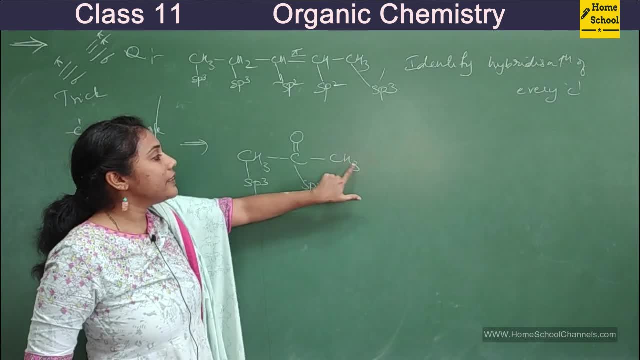 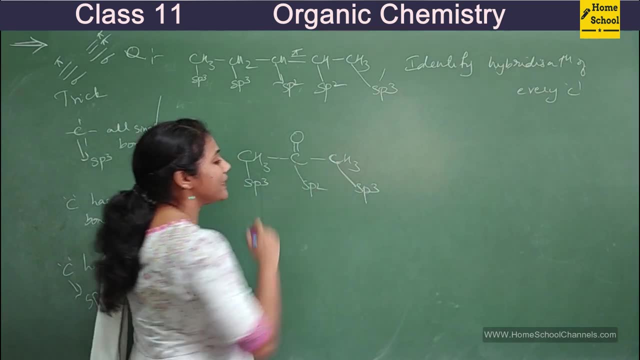 So its hybridization is sp2.. This carbon 3 single bonds and this is the 4th single bond, all single bonds only around this. So this carbon also has got sp3 hybridization like this. So questions can be asked like this: 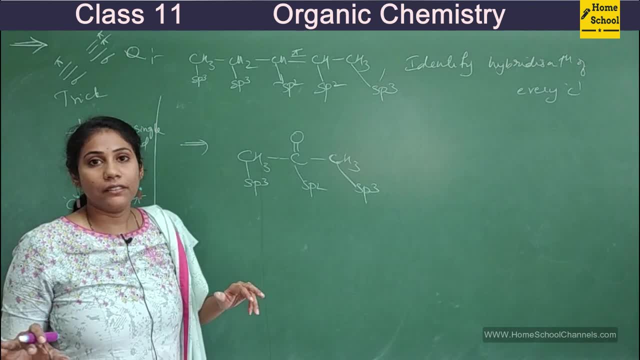 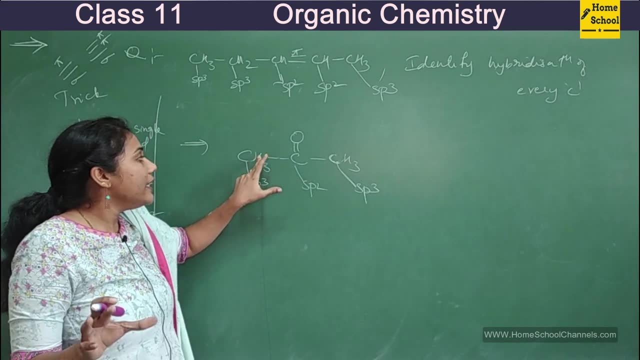 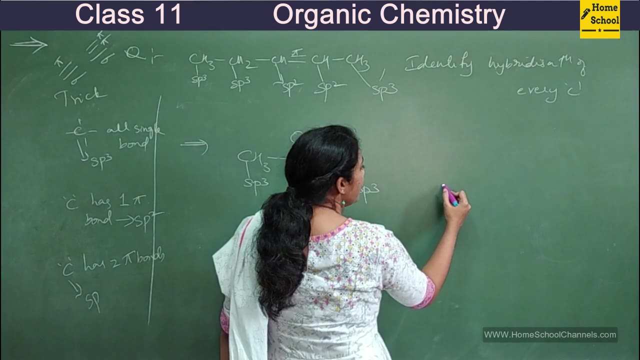 Every carbon atom's hybridization they will ask you to find. So only hybridization means it is related to only carbon atom. It is not related to hydrogen or oxygen or any other element present. So one more example. For example, you see CH3, C double bond O. 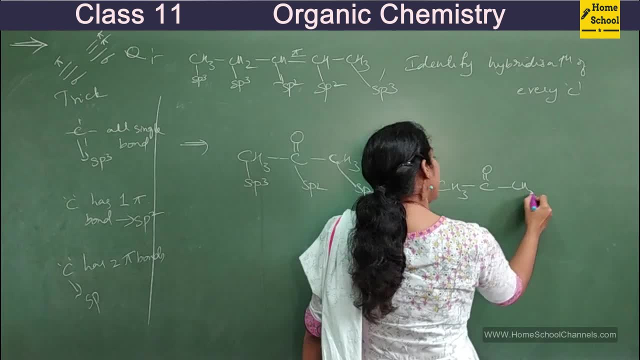 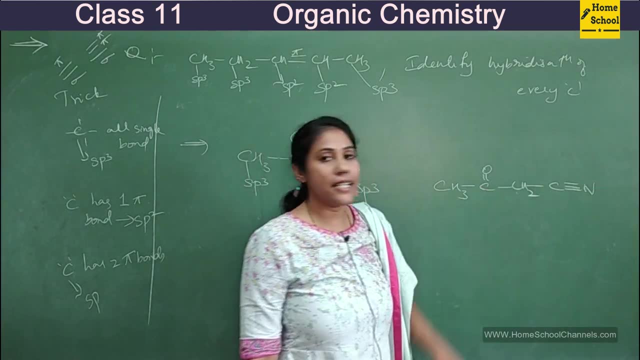 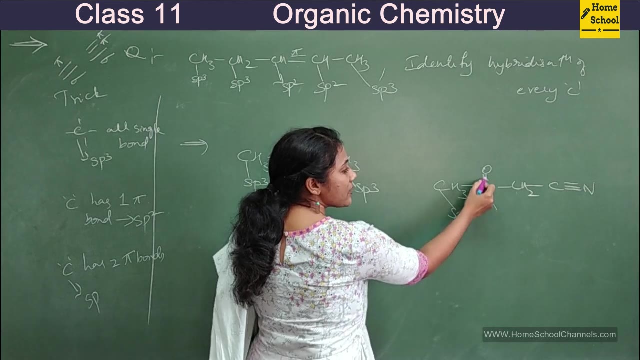 CH2 or CH2, C triple bond N. So imagine this is an organic compound. Every carbon's hybridization you have to find. So what is the hybridization of this carbon sp3, all single bonds? Hybridization of this carbon double bond is associated with it. 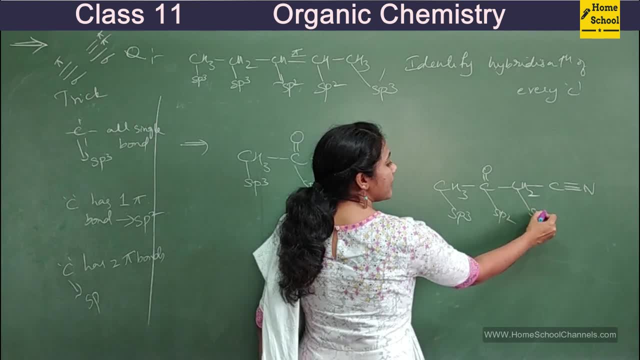 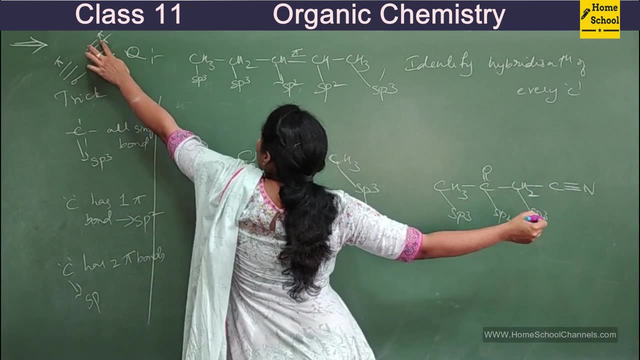 So sp2.. This carbon, all single bonds. sp3. This carbon. you see, triple bond is there with this carbon. Triple bond means what did I tell you? If you have A two pi bonds, then that carbon must have undergone sp hybridization. 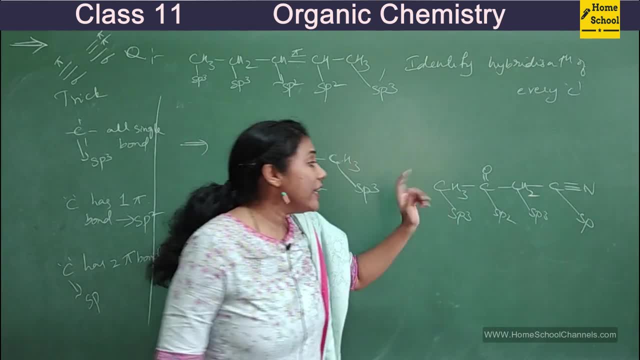 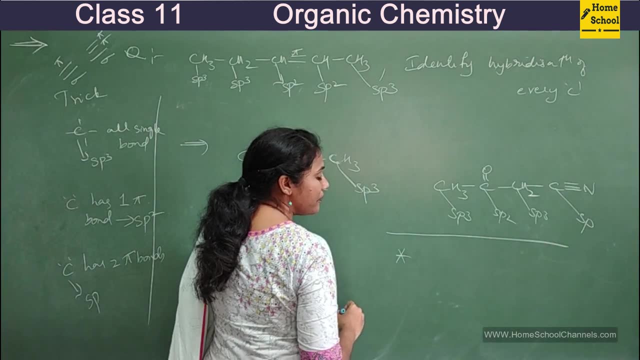 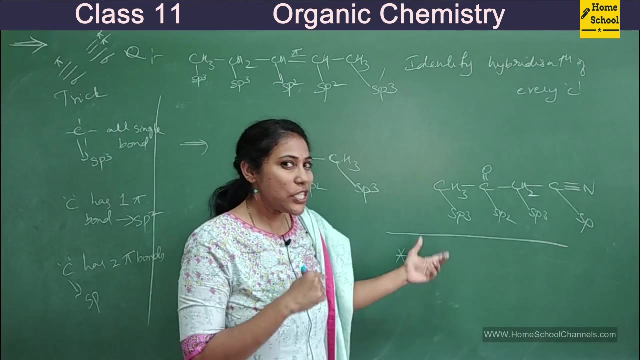 Okay, So this is how you will have to decide the answers. Very, very important concept. Okay, So now take a question. So this question's answer I will be discussing in my next video. Please do watch. It's a quite challenging question. Think and answer. So, before I give this question again, I am telling you: If a carbon has all sigma bonds, all single bonds, sp3.. If a carbon has one pi bond around it, sp2.. If a carbon has two pi bonds around it, sp. 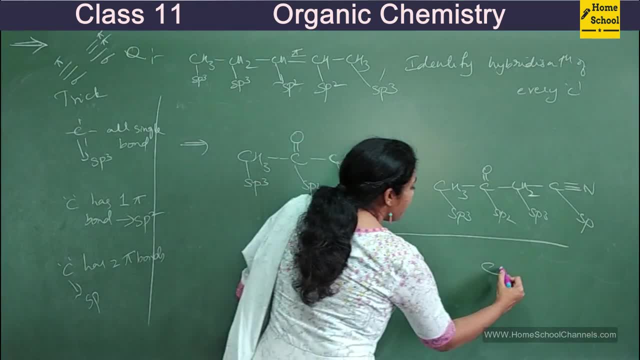 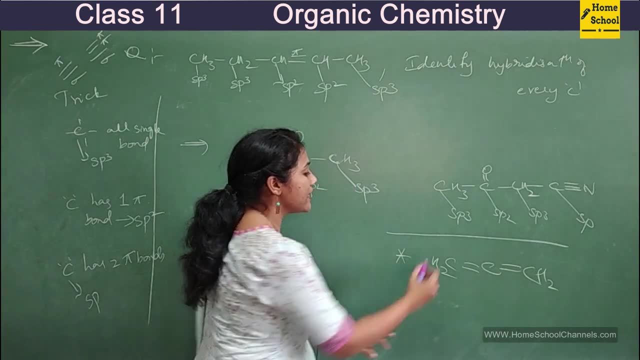 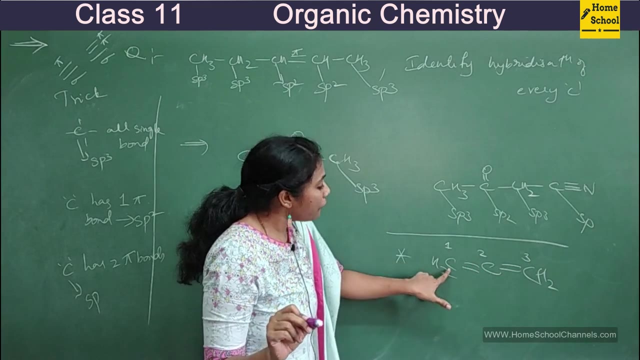 Okay, So observe example. So this is the organic compound, This is carbon number 1, carbon number 2 and carbon number 3.. So if a carbon has two pi bonds around it, sp2.. So tell me the hybridization of carbon number 1, carbon number 2 and carbon number 3.. 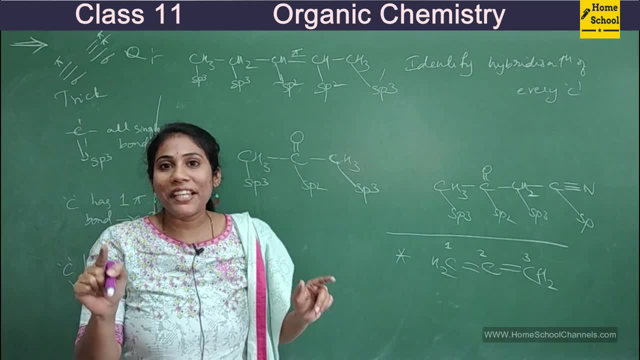 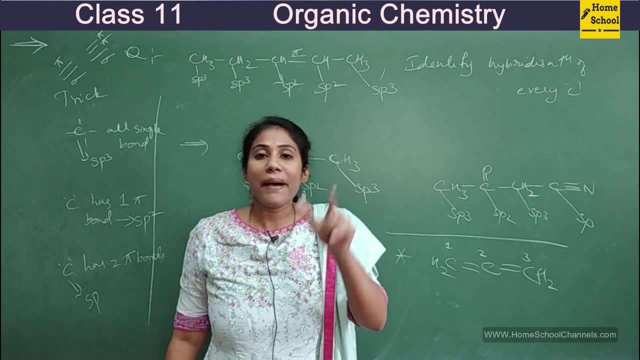 Okay And post your answer in a comment section. Let me check it out. Who will give a correct answer? Very, very important question, guys. It's answered. I will discuss in my next video, That is, in part 2 of organic chemistry.